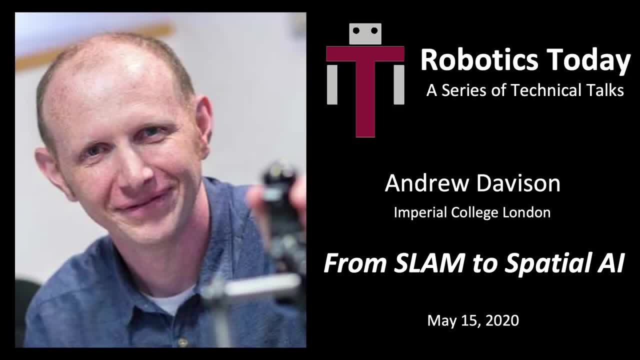 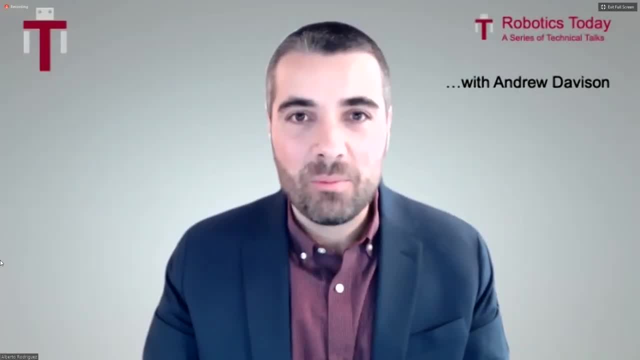 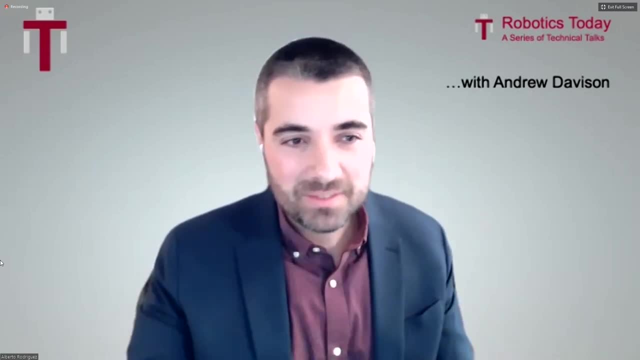 Hello everyone, My name is Alberto Rodriguez and this is Robotics Today, an open series of technical talks in robotics. I'm happy to be here to introduce the kickoff of this series with Andrew Davison, But before that, whoever you are, wherever you are, we hope. 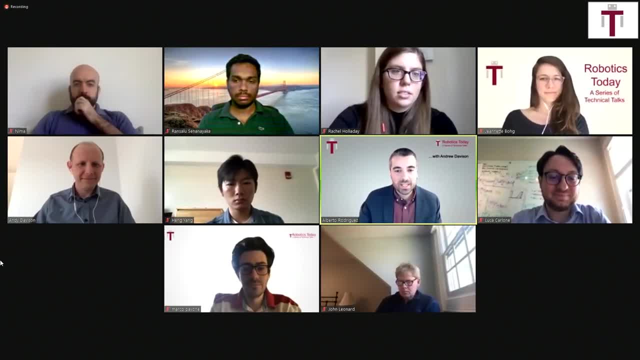 that you and your loved ones are doing well and staying safe. You know COVID has challenged the way we live and the way we work and the way we relate to our communities. including robotics And sort of that constraint has given us a great motivation to try to explore. 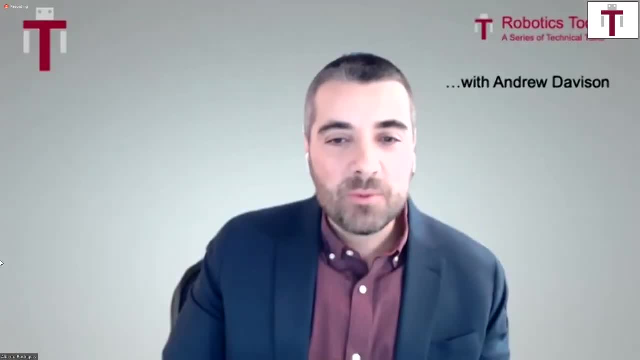 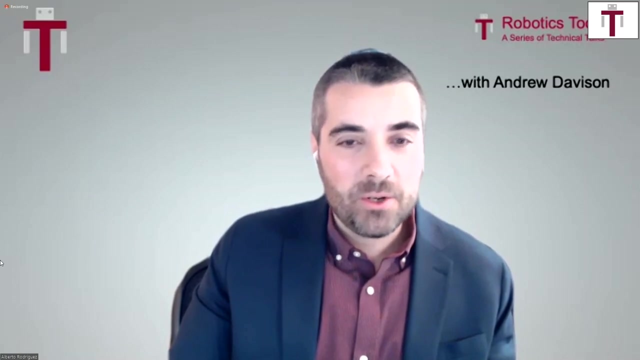 the online format and see how much we can get out of it For all of you, those of you that are listening right now. thank you. If you're not, we're recording all these and we will make the video Available in YouTube later on. So, without more delay, I'm pleased to introduce and welcome 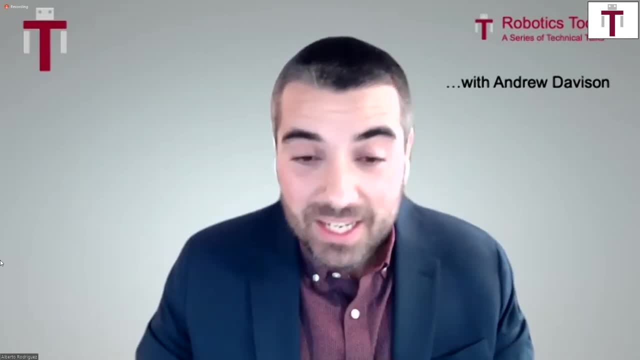 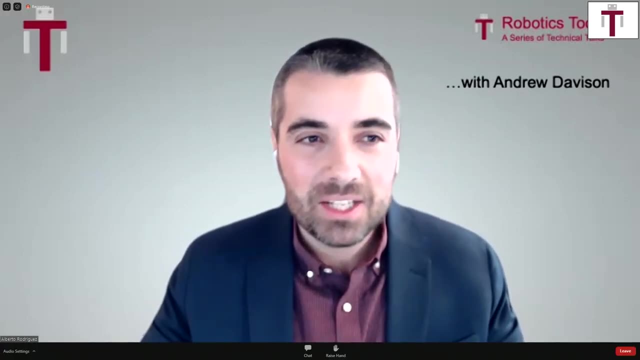 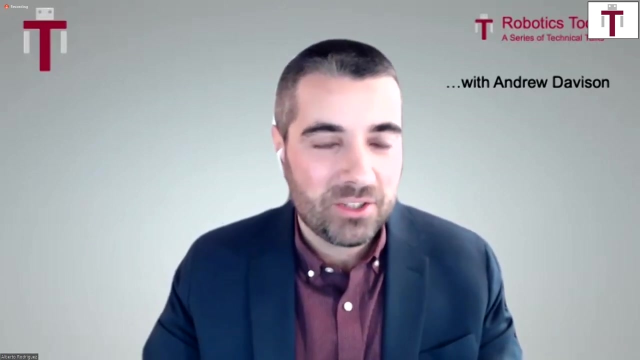 Andrew Davison joining us- I'm guessing from home, I don't know. And before that I want to welcome also John Leonard, who will be with us and the panel discussion after Andy's talk and who we've asked to prepare a spicy question to kickstart that panel discussion. 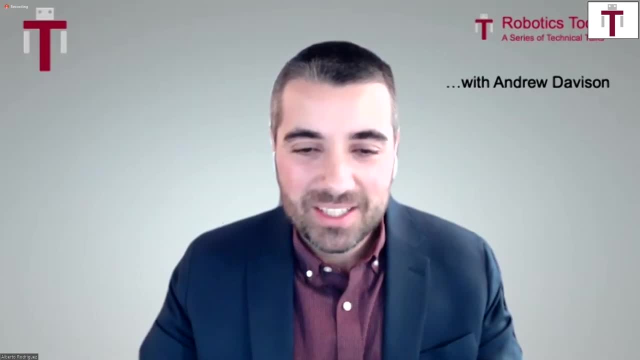 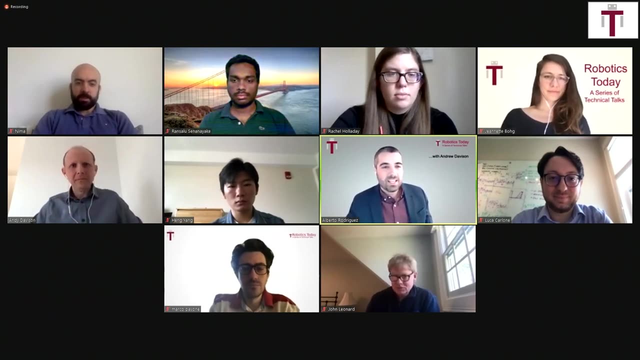 So we are looking Okay. Thank you for that, John. Thanks for joining from MIT. As many of you might know, Andrew, he's a legend in the perception community. He's a professor of robotics, vision and director of the Dyson Robotics Lab at Imperial College London, And he has developed several perception. 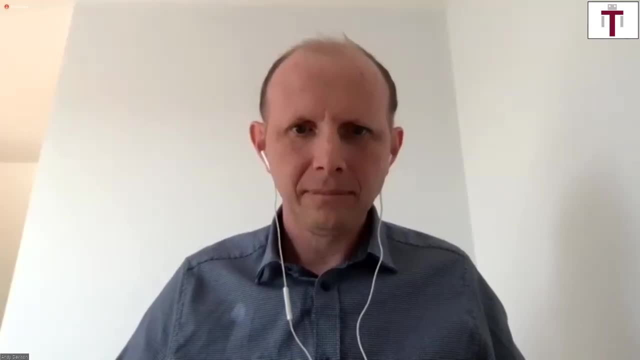 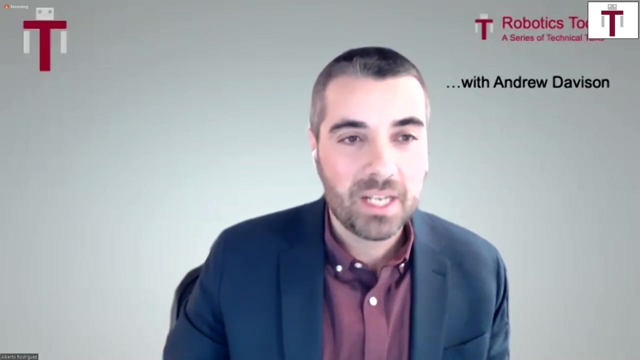 systems that have been widely adopted by a big part of our community- maybe Monoslam and Kinect Fusion are the most famous ones- And he has also deployed some of his algorithms in real robotic systems, including intelligent robot vacuum cleaners. But most of all, I 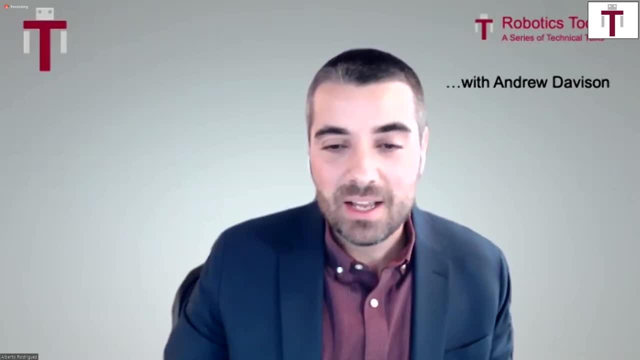 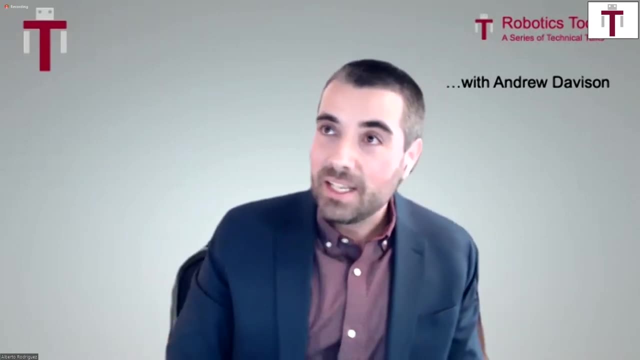 would like to highlight a couple of things from his trajectory and the large influence that it has had on many of us right. So, on one hand, Andy has been able to keep up with the huge transformation that we've had over the last few years And, on the other hand, he's been able to keep up with the huge transformation that we've had over the last few years. And he's been able to keep up with the huge transformation that we've had over the last few years And, on the other hand, Andy has been able to keep up with the huge transformation that we've 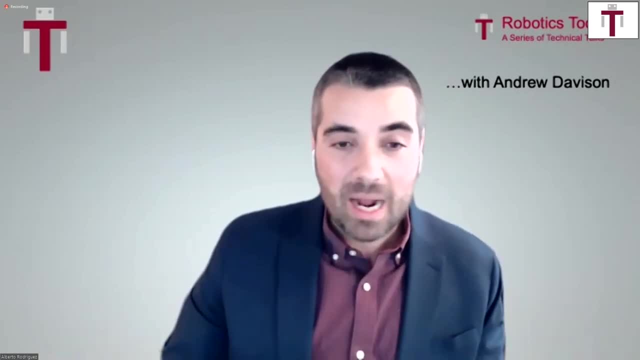 had over the last few years And he has also contributed to the great dots that us AI have, that us AI, haveatz, we MB-SOS able to do. And on the took that elimination that sensors have had in the And on the took that elimination that sensors have had in the last couple decades Right. 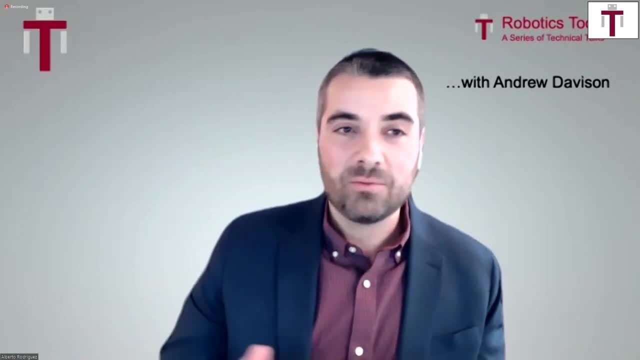 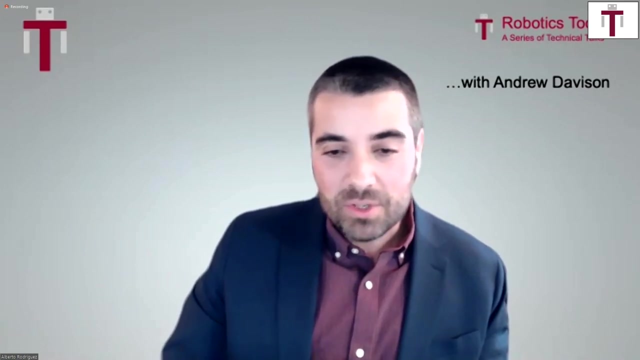 So if you look at the two most influential works or the two most cited works in his career- Monoslam and Kinect Fusion- they drive from very different sensors and somehow Andy has managed to stay at the forefront on both ends of that transformation, which is quite remarkable. 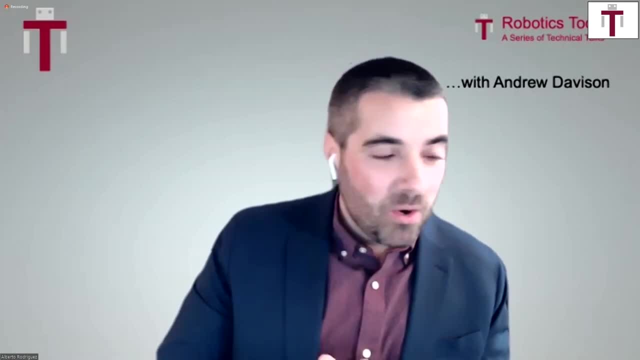 And maybe the second thing is that Andy has also worked us through how we analyzeuen similar sensory systems. we are now using data from the CTR that we have actually became very heavily involved in And, I would compare, has also walked us through another transition that the perception community has undergone. 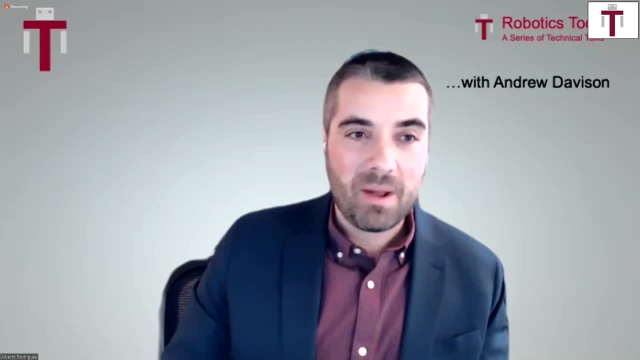 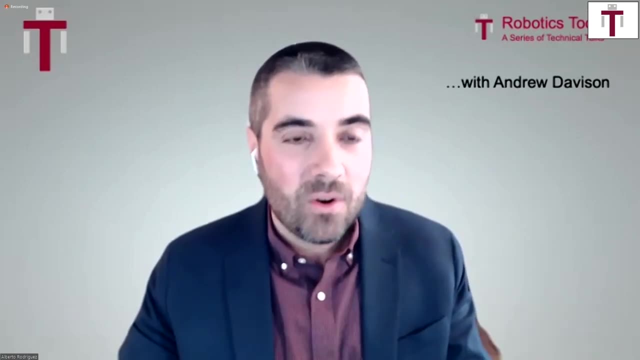 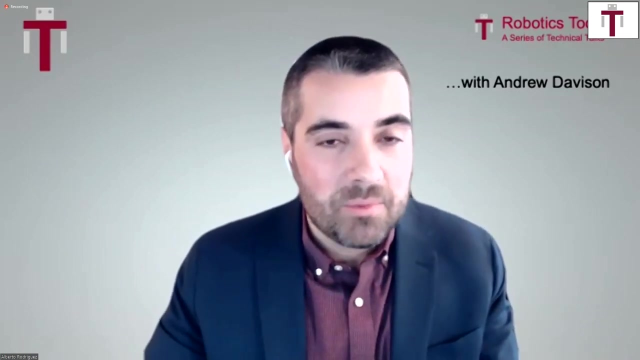 in the last two or three decades, going from maybe a more narrow, maybe narrow, slightly narrow perspective, a geometric perspective on what perception is, to a more broader sort of semantic understanding of what perception is or what how he calls it spatial AI. 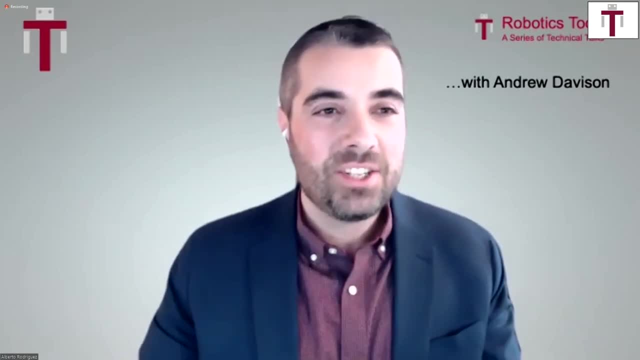 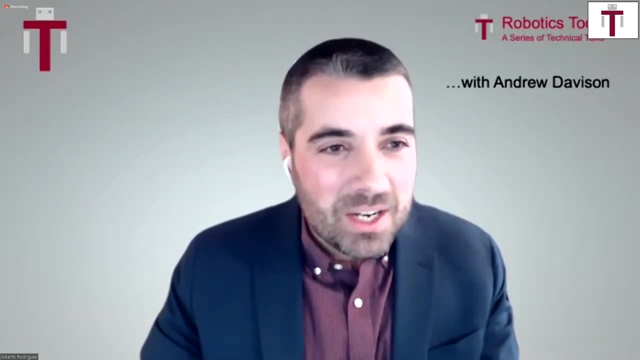 So, without more delay, Andy. of course, the cliche, the long-standing cliche, says that SLAM is a soft problem, but somehow, stubbornly, it seems like it remains to be a soft problem. How is that? Why is that, Andy? 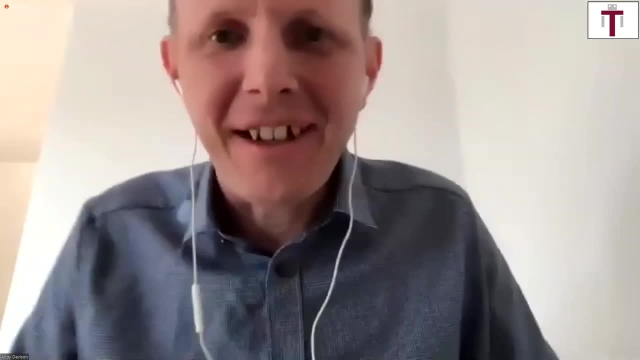 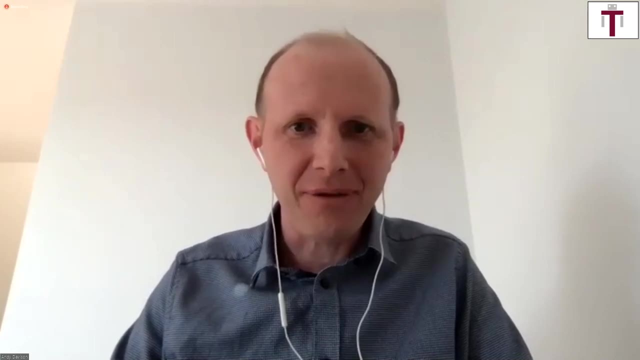 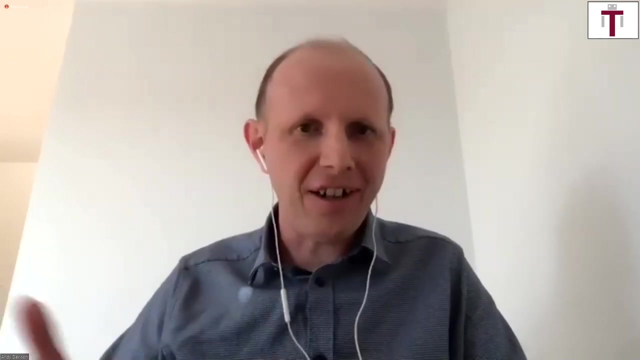 Thank you for joining us. So thanks very much. Yeah, so it's a problem that I think has continued to evolve into more and more interesting and challenging areas. So, as you mentioned, you know sensors change, you know different sorts of, you know the. 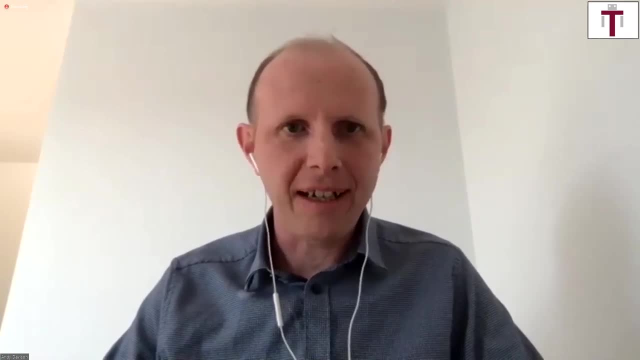 background. algorithms and tools change and our goals in applications change, And you know, one of the messages I want to get across in the talk is that I see SLAM as a rolling problem that's always changing into something even bigger, and that's what 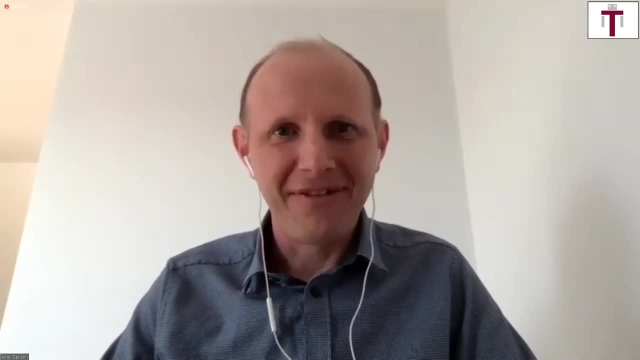 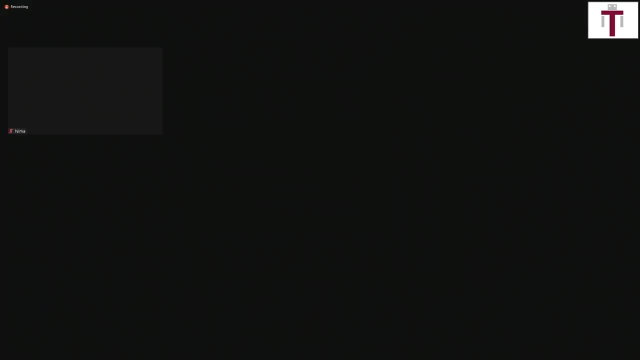 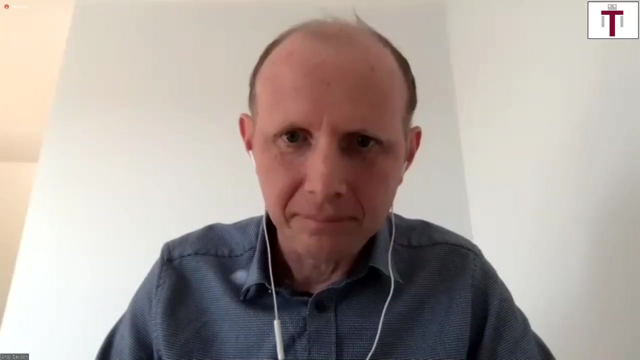 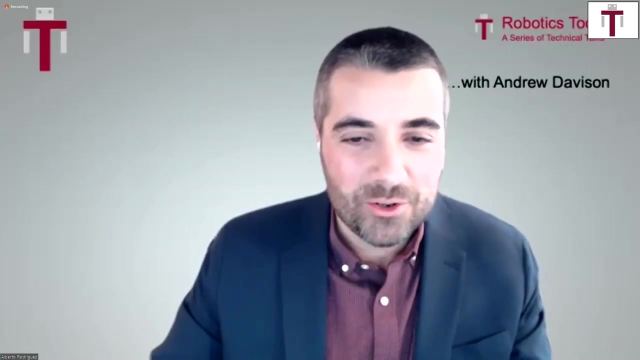 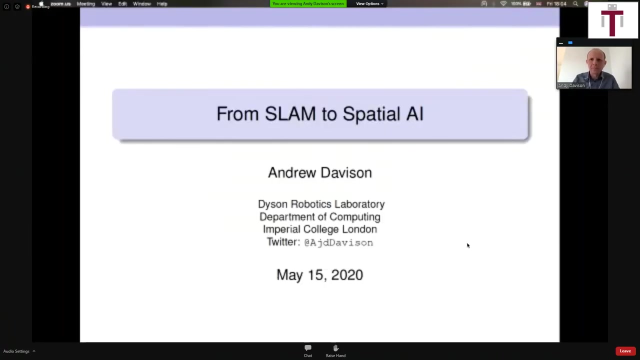 I'm now calling spatial AI. Excellent, Thank you. So I'll share my screen and start: Yeah, Yeah, go ahead. Okay, Yeah, sure, Your show, Just give me a second. Okay, So my slides are coming through, okay. 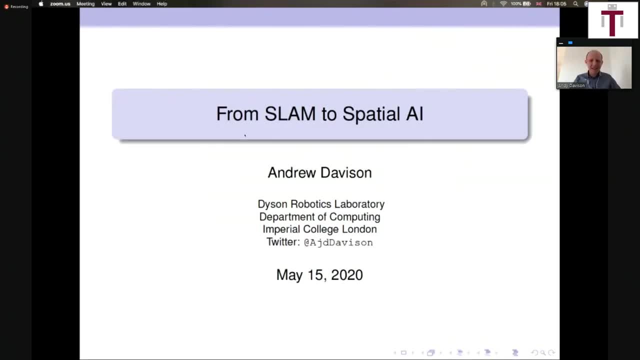 Yeah, Good, Okay. So thank you very much for the introduction, Alberto, Thanks to all of the organizers of this fantastic new series. So, of course, it's a great honor to be invited to be the first speaker, and I'm, you know. 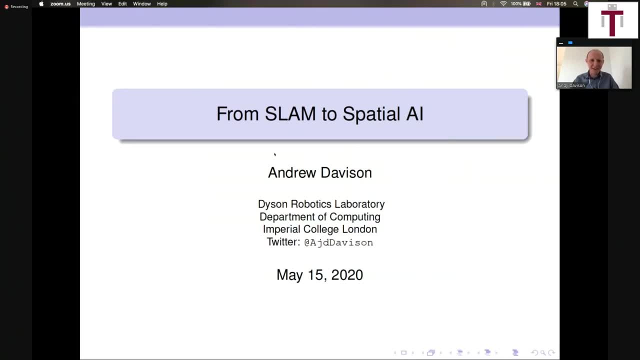 excited to watch the rest of the talks and what it looked like. It's going to be a great program. Thanks also to John for joining the panel. So John's someone I've known and followed his work, you know, right since the time of. 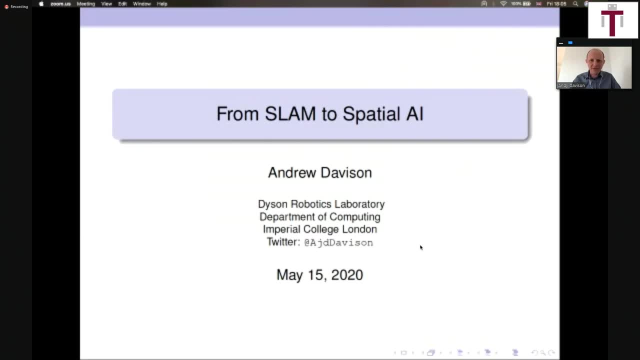 my PhD. Okay, So my talk is called from SLAM to Spatial AI, and I've already said something about what that means, So I'll go into a bit more detail on that. I'm going to talk a little bit about a little bit of history- not too much, a little bit. 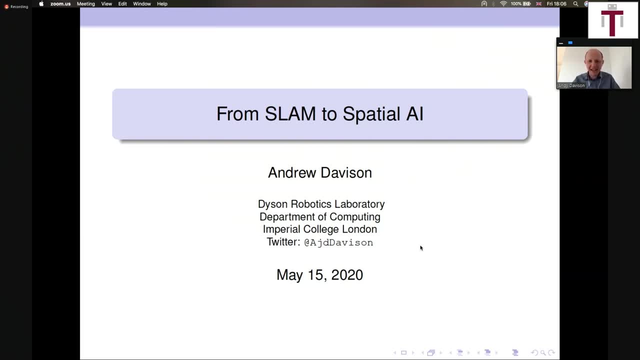 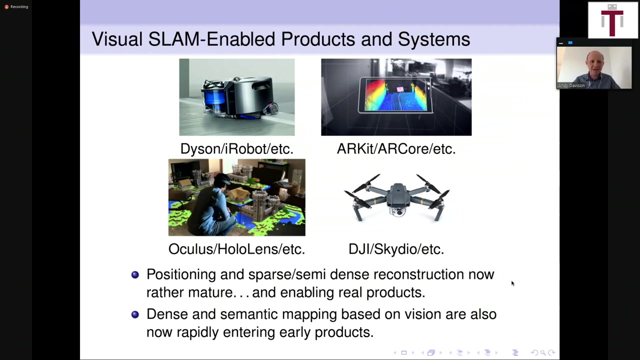 about my general thoughts about where this whole field is heading and then also show you, you know, various examples, in particular from recent work in our lab, of systems that I think are representative of progress in this area. So let's start by thinking about what's actually out there at the moment. 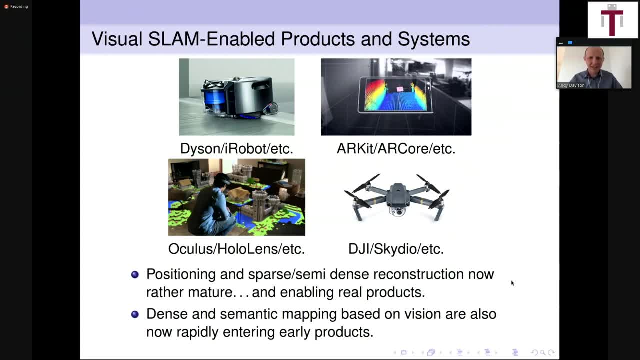 So, having worked in this domain now- for you know, over 25 years since I started my PhD, when working on SLAM using vision was really just a bit of an out there research idea- we've now reached the stage where visual SLAM is actually present in a number of products. 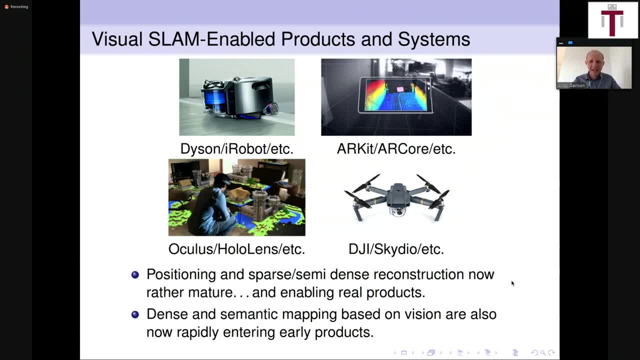 that you can actually buy. So I've shown a selection of them here. You know, These are certainly what we would think of as robots. so the Dyson robot vacuum cleaner- I'm showing there- drones such as from companies like DJI or Skydio. these, you know, run visual. 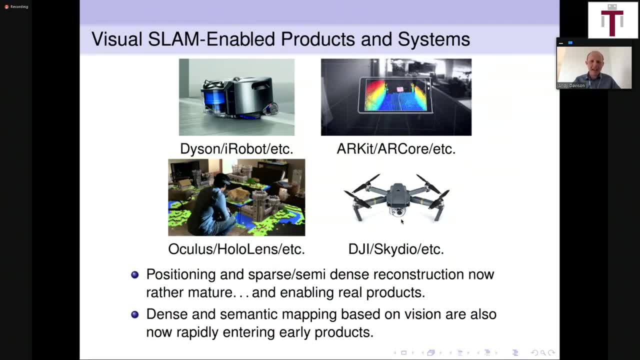 SLAM systems for localization and mapping, but then there are also a lot of other devices that we might not think of as robots. So inside mobile phones there's software like ARKit or ARCore that enables position positioning and real-time mapping on those devices using cameras and other sensors. 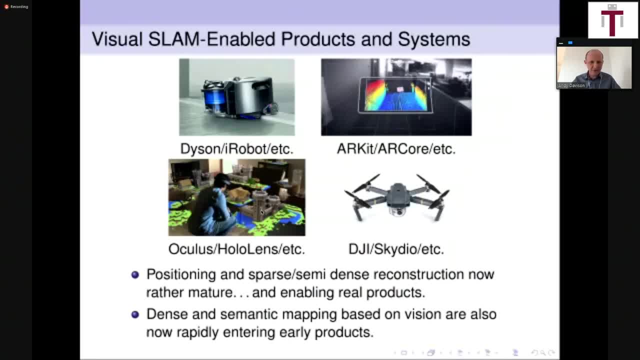 And then this emerging area of headsets for virtual and augmented reality. these are also SLAM enabled devices. So this is, you know, kind of an amazing thing to me that this technology is really getting out there now. But if we look at what's actually in products like this, it's mostly, at the moment, positioning 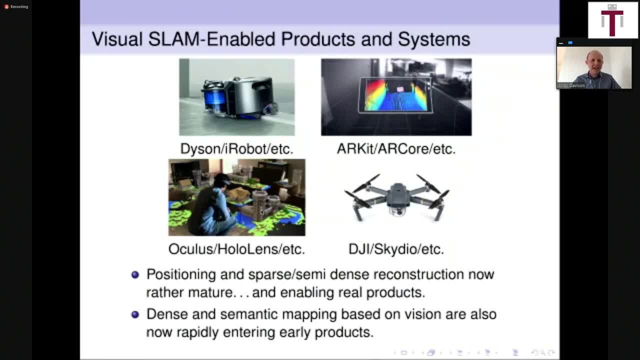 and perhaps sparse or semi-dense reach. So you know, I think that's the technology inside these products. So there's more and more levels of technology gradually coming in. So things like dense and semantic mapping- that I'll talk about later, based on vision. 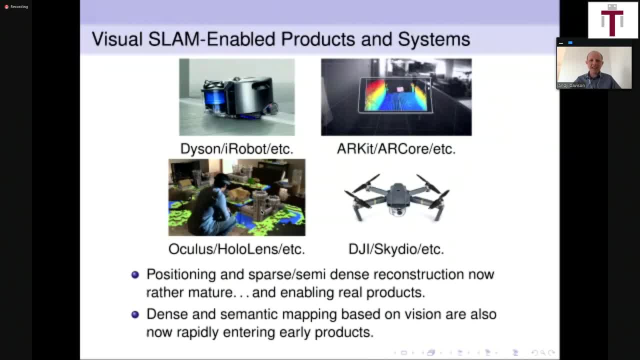 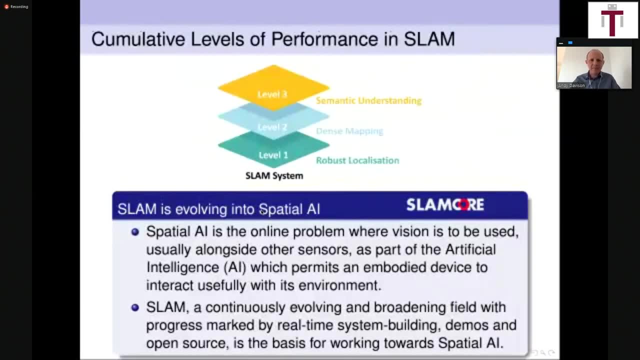 are also entering these products, But I think it would be fair to say that these are all still relatively- you know- early sorts of products out there on the market. So one way of thinking about SLAM is to think of Gradual progress in terms of adding levels of capability. 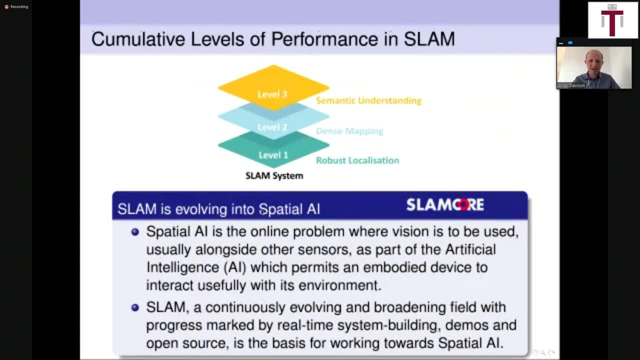 So this is a picture that comes from our startup, SLAM Core, where we really think of levels of capability in SLAM, from localization up through dense mapping and then eventually to semantic understanding. So I think of SLAM as this. really, you know, rather than saying SLAM is something that's. 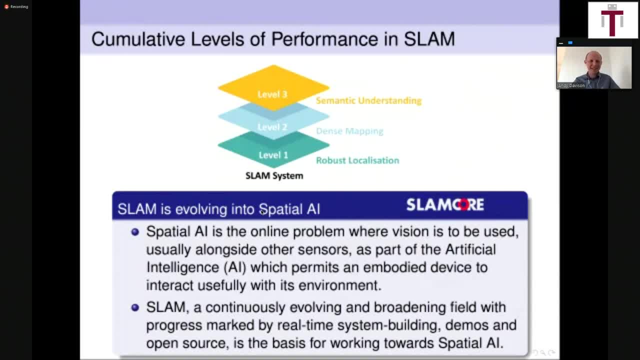 done and then these levels sit on top. For me, all of this is SLAM, And it's gradually evolving. So I think of SLAM as this, really, you know, rather than saying SLAM is something that's done and then these levels sit on top. For me, all of this is SLAM and it's gradually. 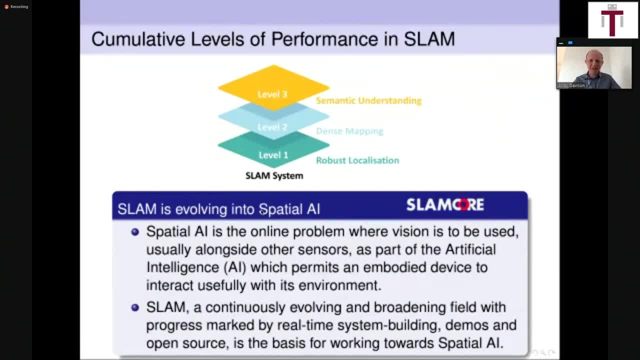 evolving into a bigger system And for me that's a valid way of thinking about it, because I always come back to SLAM like ways of thinking whenever we're trying to add these new layers. So every time you add a new capability, it may affect, you know, the ability of the robot. 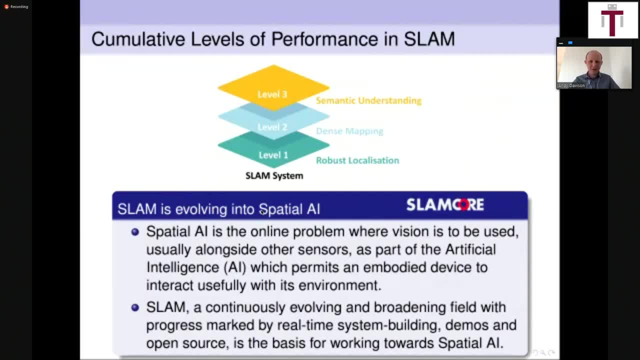 to localize, for instance. So I see it always as a kind of closed loop, And hence my argument that SLAM is evolving into something bigger, spatial AI, which I define here as as the online problem where vision is to be used, usually alongside other. 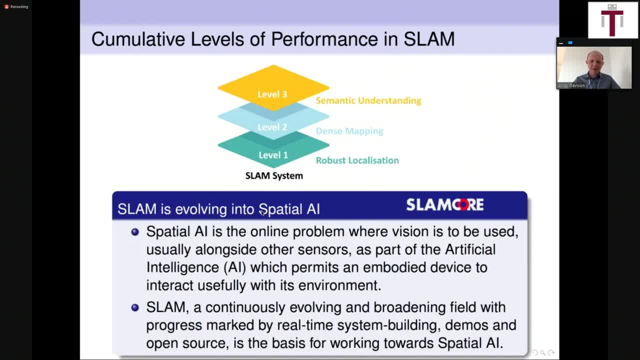 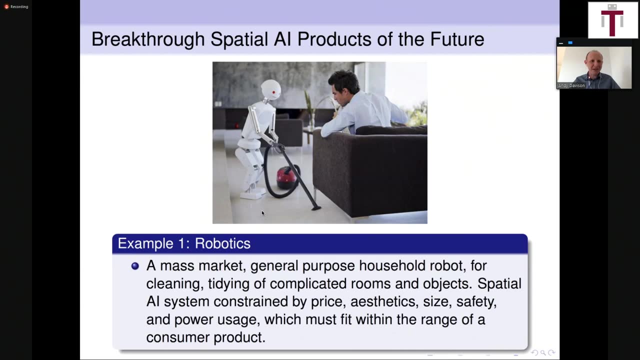 sensors as part of the AI which permits an embodied device to interact usefully with its environment. So really we're thinking about embodied spatial AI in a general sense here. So where might that take us in the longer term? So I've just got a couple of ideas here of products we might imagine in the longer term. 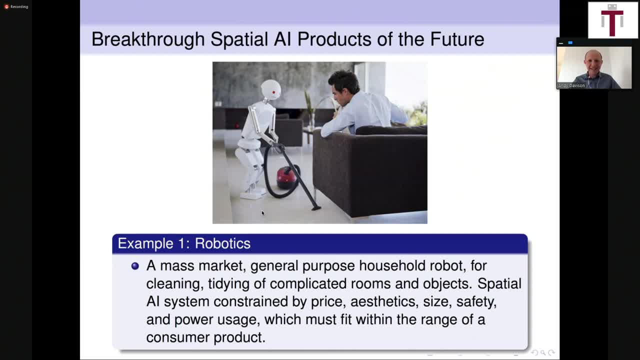 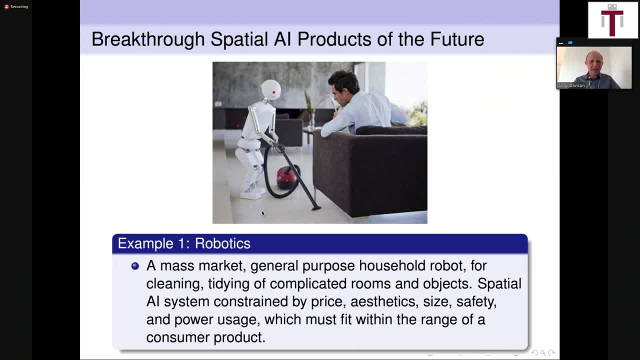 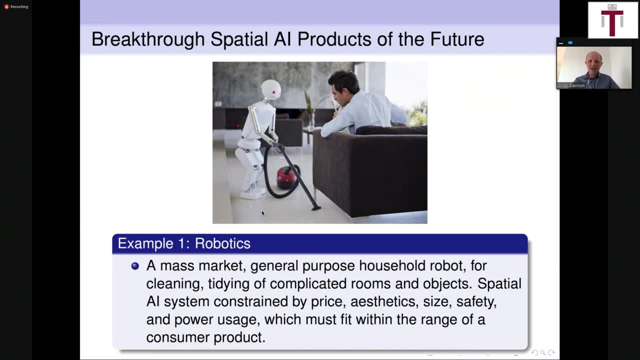 But let's imagine this product, a mass market, general purpose household robot. So it may look nothing at all like this. Probably won't look humanoid at all, I strongly expect. But its job is cleaning, tidying of complicated rooms and objects. 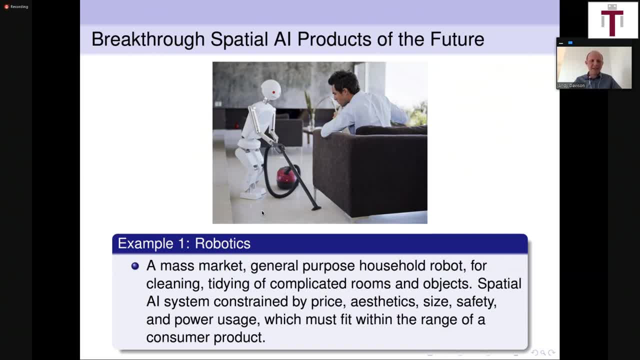 And it's going to need a spatial AI system that gives it all the perception that it needs to do all of that. But let's bear in mind that the system that it has will be constrained by price, aesthetics, size, safety, power usage and all these things which must fit within the range of a 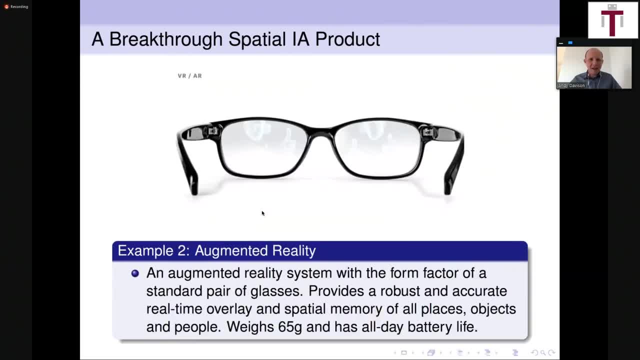 consumer product. here's another product that i think could really be a breakthrough, and note note that i've called this a spatial ia product. so this is a rather cute inversion of ai to to stand for intelligence augmentation. so i think of this as as a sort of intelligent device. but 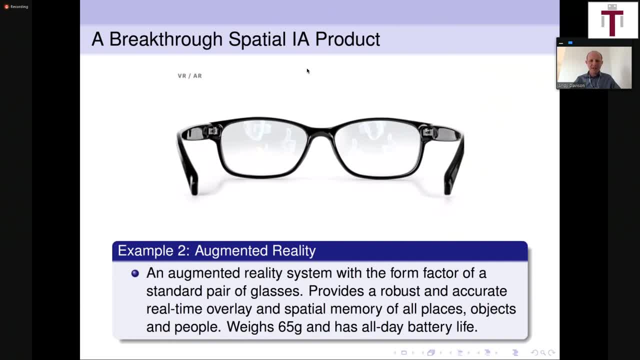 that's designed to work with a human in the loop. so this is a concept for a future augmented reality system. with the form factor of a standard pair of glasses, it provides a robust and accurate real-time overlay and spatial memory of all places, objects and people, but it has very, very strong. 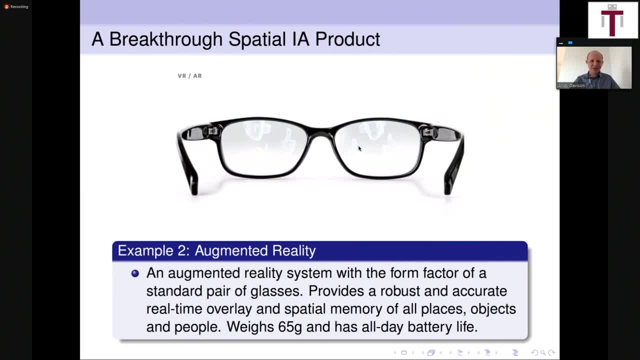 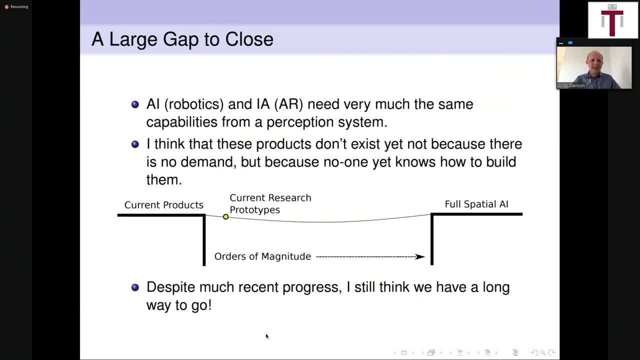 constraints on how it can work. so i think for this to really change the world, it may have to weigh 65 grams and have all day battery life. so i'd like to make the point that you know, i think, both of these two types of products, they probably require quite similar capabilities from perception. 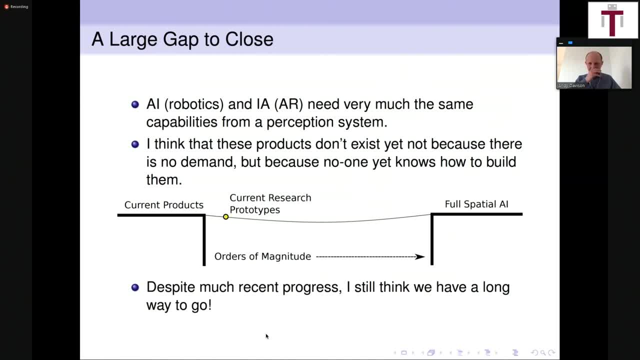 system. i think either of these products would have a massive impact if they existed. the reason they don't exist yet is not because there's no demand, but because no one yet knows how to build them, and especially within those very strong constraints of real products. so i've just got a sketch here. 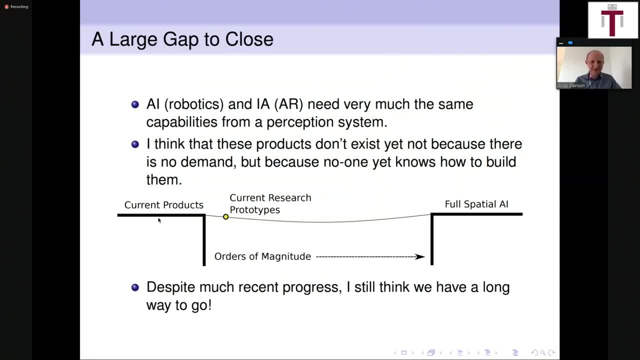 of of how far i think we've got to go. we've got current products on the left, we've got current research prototypes happening in labs, and then we've got this big, big gap to where we really need to get, to this full spatial ai performance constraints of practical devices, And I think we're talking about orders of magnitude of progress. 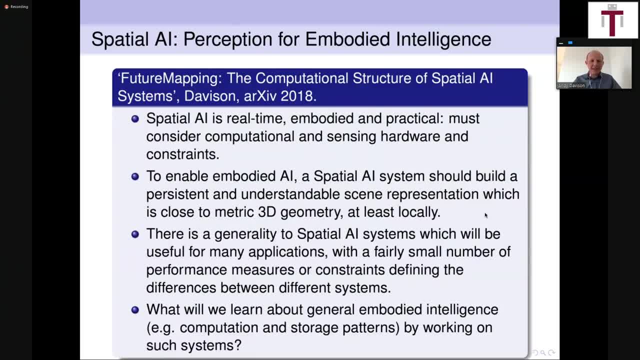 needed. So, thinking about this concept in general of spatial AI, so I think it's perception for embodied intelligence, I've written recently a kind of discussion paper about this whole topic that anyone might be interested to read, So it's called Future Mapping. 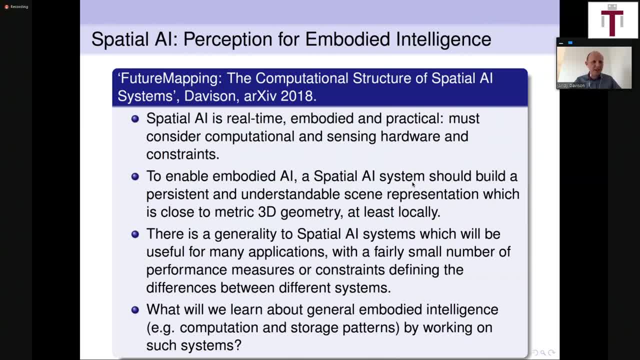 the Computational Structure of Spatial AI Systems. It kind of defines more about what I understand this problem to be. It makes a few hypotheses, and the key hypotheses are along the lines that a spatial AI system should build a persistent and understandable scene representation which is somewhat close to metric 3D geometry, at least locally. Within that it will contain. 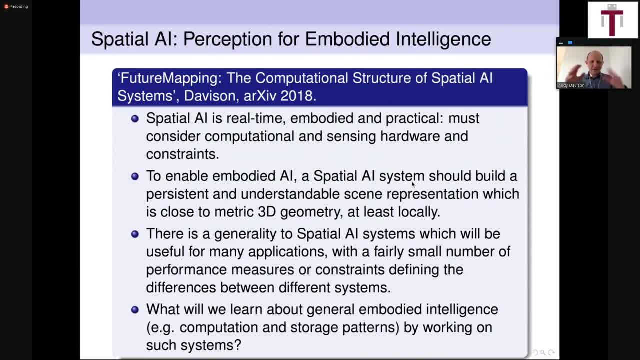 hierarchies of lower-level geometric information and higher-level semantic information, And I also think there's a generality to spatial AI systems. So, whichever of these applications this might be, it's a question of how do we build a spatial AI system, And I think it's a question 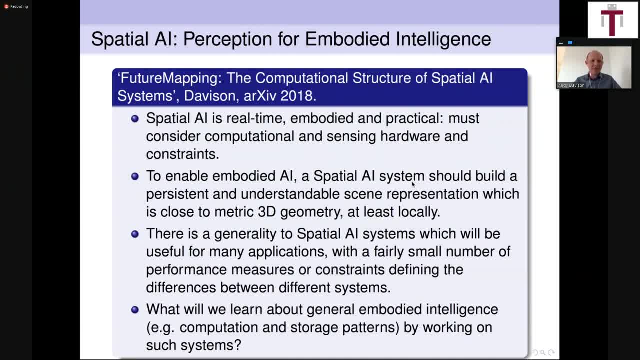 might be ultimately useful, for I think there'll be a lot of commonality between the systems and maybe a fairly small number of performance measures that define the differences. So I also think that by working on this topic with the main goal of actually developing products, 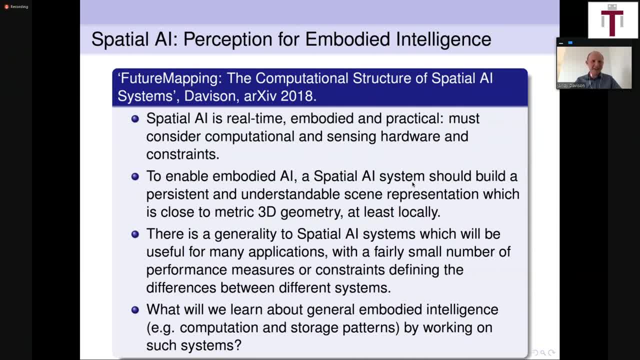 we may learn a lot about general embodied intelligence. I think that's something very interesting to discuss. So what are the kind of computation and storage patterns that are required to do embodied intelligence efficiently? So that's, I think, interesting general research on AI and intelligence. 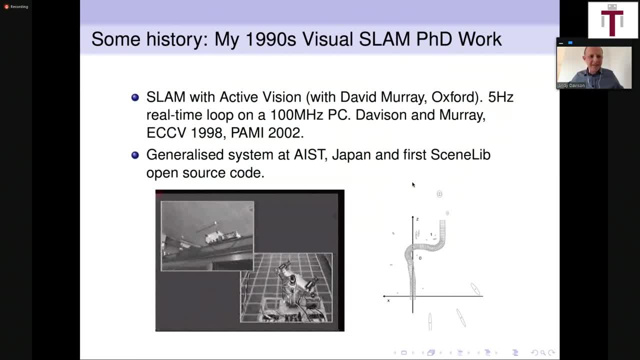 So I'm going to move on to a little bit of history here, So really to guide you a little bit through these levels of progress that I've talked about in SLAM. So just very first, briefly- so probably John may be the only person here that actually remembers this work- This was my PhD work. 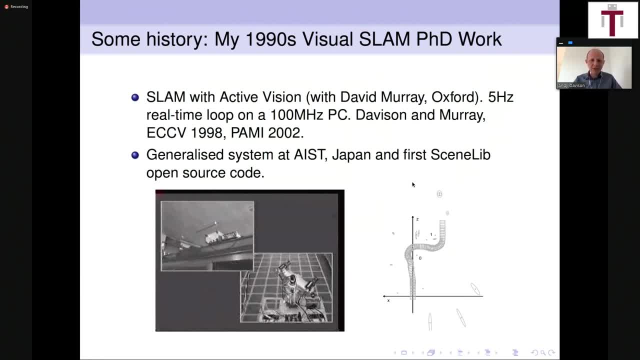 which was in the Activision lab with David Murray in Oxford back in the mid-90s. So I worked on what turned out to be one of the very first visual SLAM systems. So this was a stereo active head with two cameras mounted on top of a mobile robot platform, And we were able. 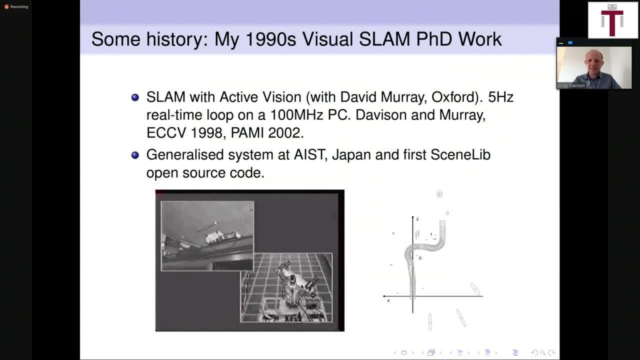 to achieve localization and mapping with this system by having it drive around and map a set of point landmarks in a scene. So on the right you see a picture of the estimated trajectory of the robot and the estimated positions of a set of landmarks that it's built into. 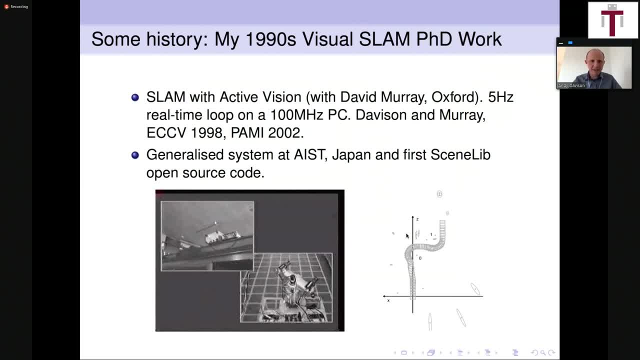 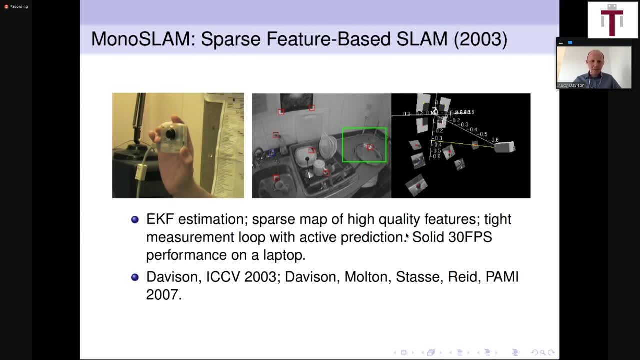 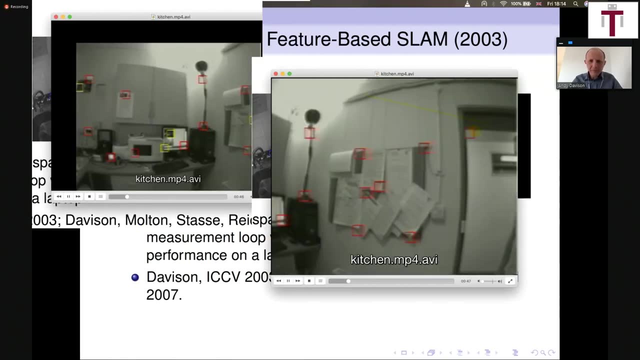 And this was all running in a Kalman filter for joint estimation That led, after a few years onto the MonoSLAM work. So let me just quickly show you a video of this. So this was really inspired by saying: let me just go back a second. So it was inspired by saying: 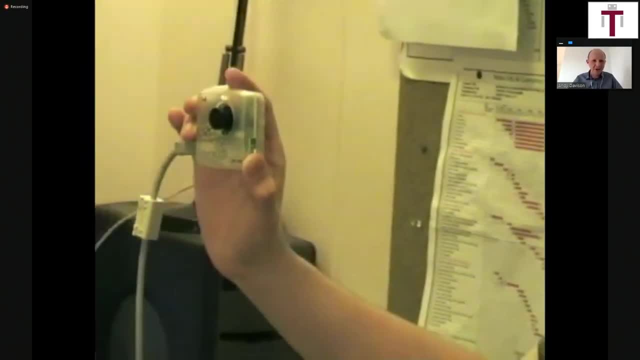 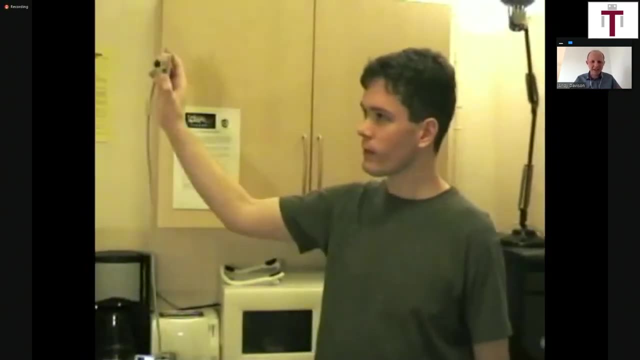 can we do SLAM with the simplest possible vision based hardware setup, ie a single handheld camera moving around in a room with no other kind of sensors and ideally no prior information about the room. So the goal is to localize this camera in 3D as it's moved around. 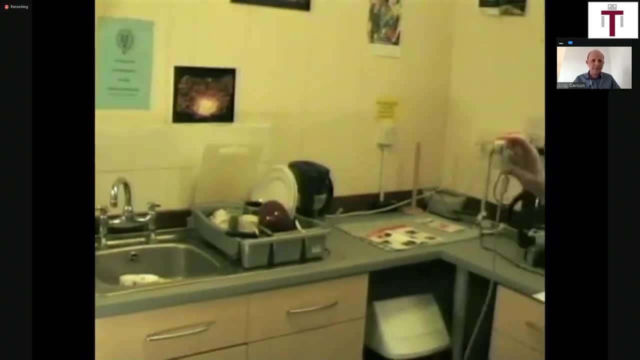 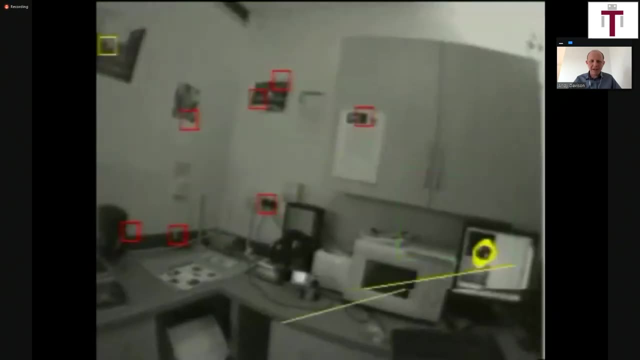 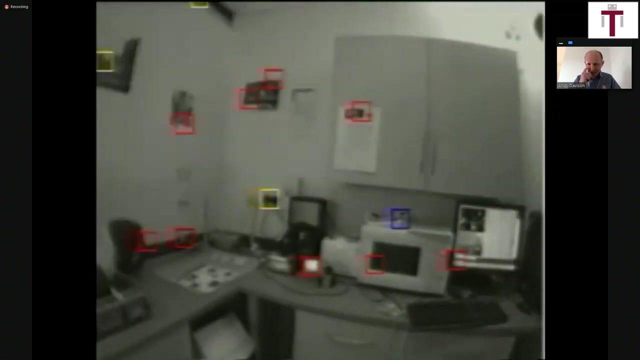 in a general way, in real time, and to build a map of the scene that it sees. So here you'll see the camera's view of the scene And you'll see that what's going on here is we're detecting and tracking a set of landmark features in the scene, And so these are salient points in the scene And 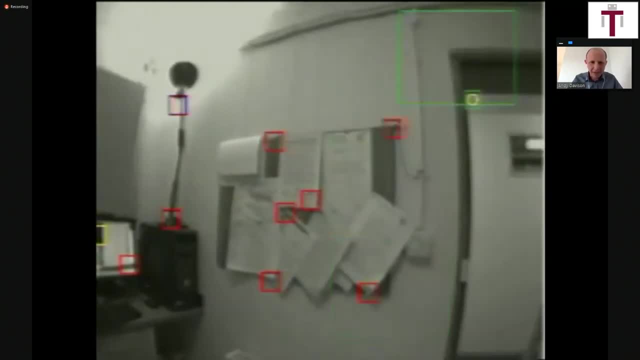 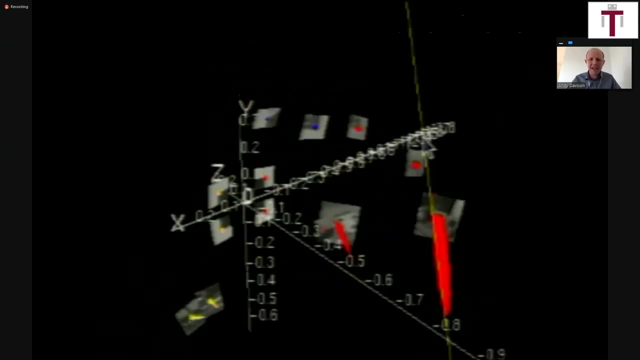 they're building them incrementally into a persistent map. So if I just skip forward slightly here, here you'll basically see the results of that. So this is the real time 3D estimated map of the scene, where the box flying around is the estimated position of the camera and each of these 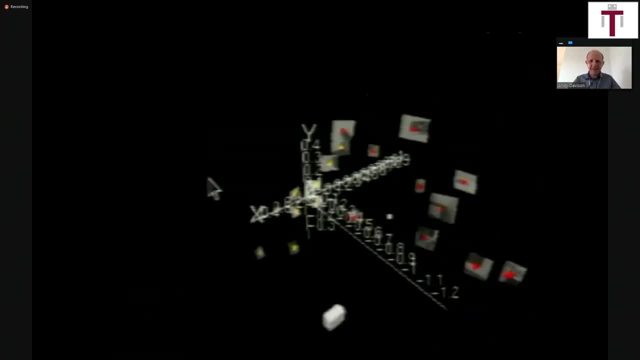 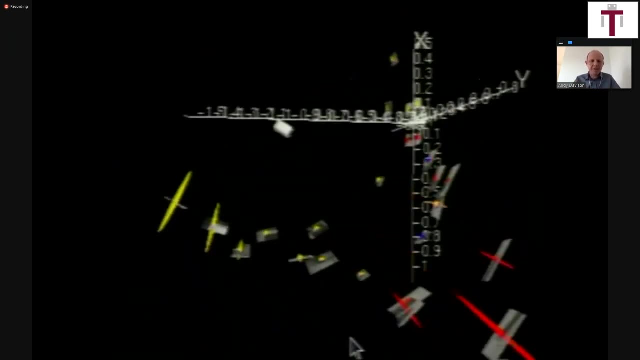 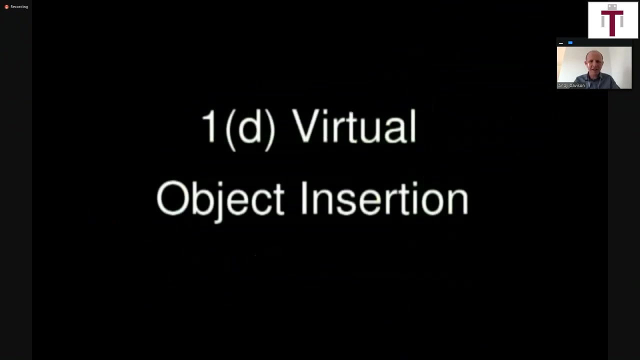 patches is an estimated feature in the world with a 3D ellipsoid. So this is a sparse, feature-based map of the scene And really you'll see that we're not getting much information about the scene. here a map of the scene which is enough to enable localization of the camera. so the main thing. 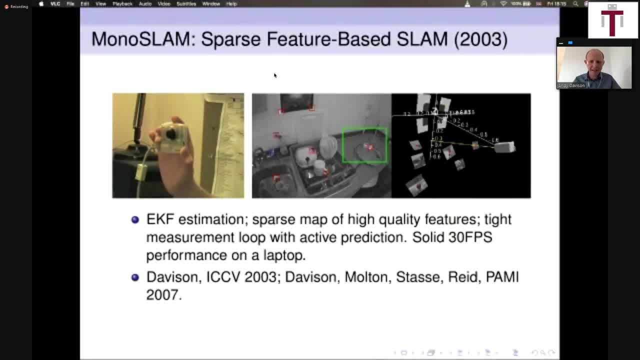 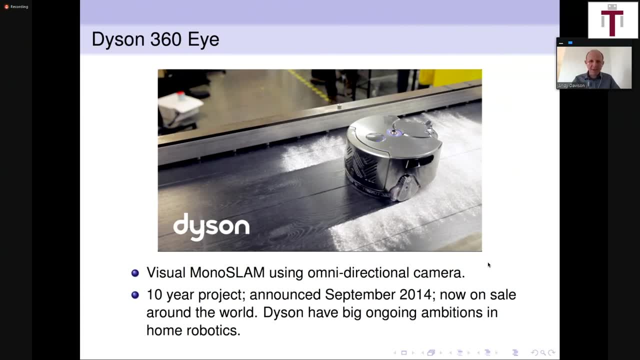 we're interested in here is is: where is the camera? and this is a map that's. that's sufficient to do that um. so that system, or something very uh much based on that, is what enables the um slam capability in in the dyson 360i robot. so, uh, around the time of mono slam, i first met, uh, some of the 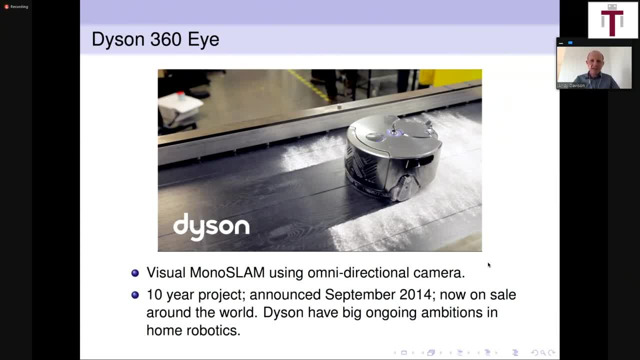 researchers from from dyson and we we decided uh to work together on on what seemed like a very ambitious concept at the time of building a product. that deal did a visual slam and that eventually led to the release in uh in 2014 of the of the dyson 360i robot, which performs a monocular 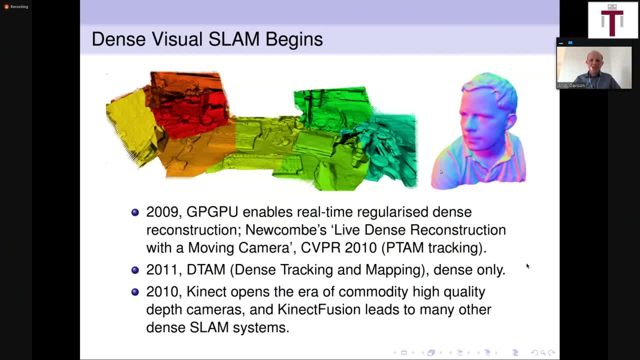 slam. um. so a few years after that, and now we're talking around 2010, i, i think there was the next big kind of a advance in real-time visual slam systems. uh, and this is the arrival of dense slam. so the goal here was now starting to switch towards. you know, we're doing pretty well on. 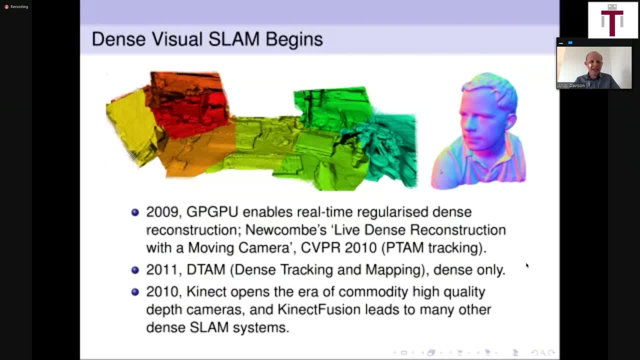 positioning a camera. how about this next thing of getting more significant detailed information about the scene? so can we actually build these really detailed scene representations where we can see the shapes of objects and so on? uh, so in in particular, uh, an important person in this was richard newcombe, who was a 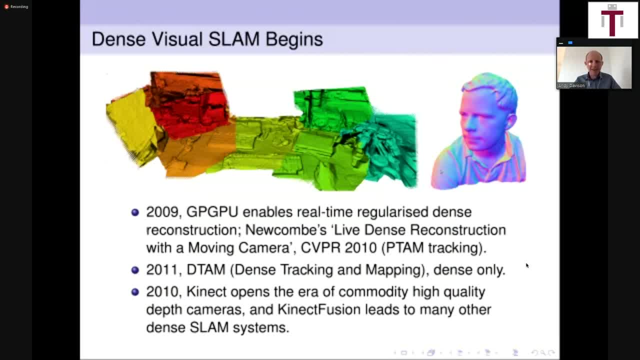 phd student in my lab at the time and he worked on several very influential systems, including dtam, which which was a system just based on pure rgb images and was able to do dense real-time mapping. and then the other important one was connect fusion, um, which used a connect camera. 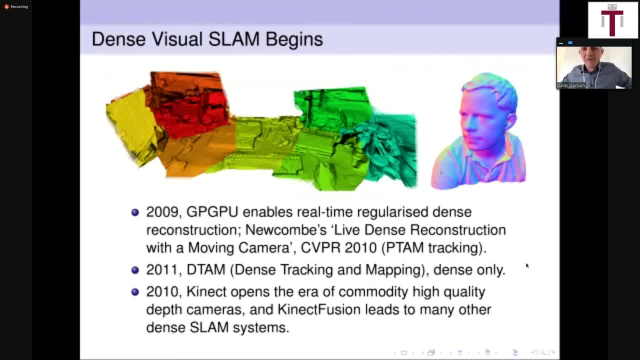 so so you know what's really interesting here is it was the arrival of certain commodity technology that made these kind of things possible, so in particular gpg. so so general purpose, um, graphics cards that were programmable to do computer vision like things are behind all of the parallel processing that you need to do this kind of- uh, real-time dense. 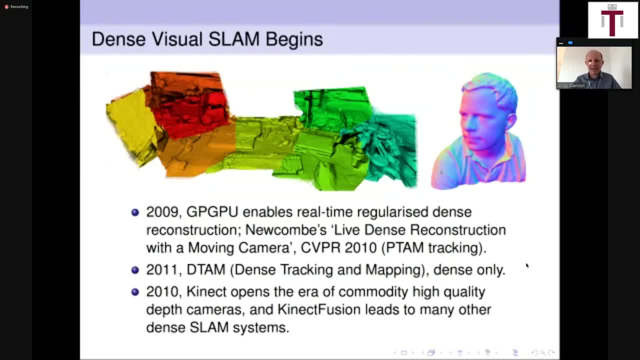 visual slam. and then, of course, depth cameras, and especially kinect, and it's hard to remember now what a kind of revolution that was when it when it came along. so depth cameras had existed before 2010, but they cost thousands of uh dollars and they weren't very good, and suddenly you could. 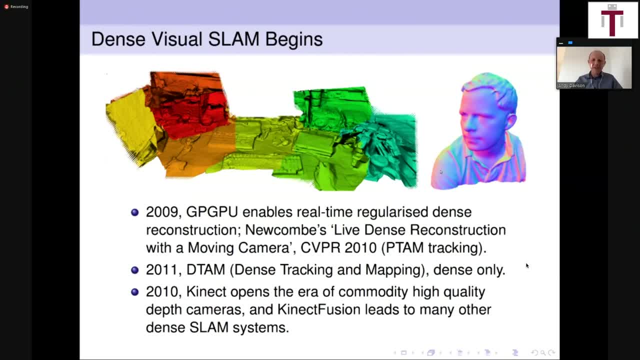 buy this thing for a hundred dollars that there was. there was a lot of money involved in it, so it's. it was great. so, uh, you know, richard actually was doing an internship at microsoft research. um, just as the connect was about to come out, come out and was able to to work on that. uh, and really, 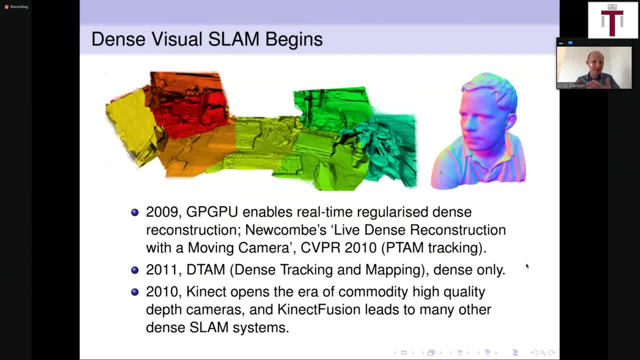 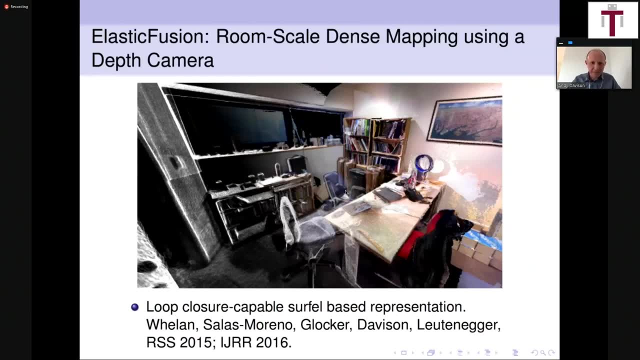 see what, what can you do in real-time slam if you have a stream of pretty high quality uh depth information? so just to show you a video that's representative of dense slam systems, that this is a system called elastic fusion, which was uh work from our lab, the dyson. 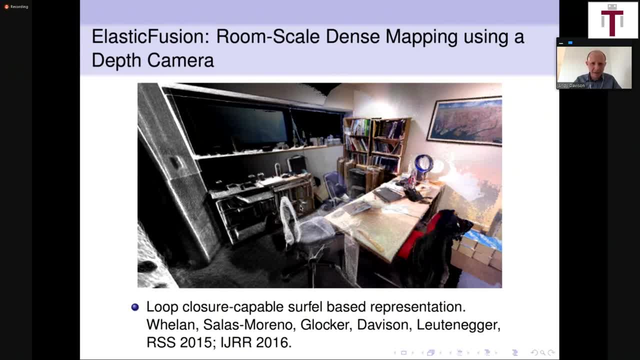 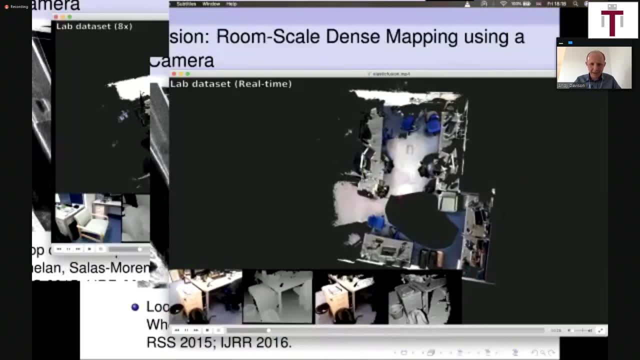 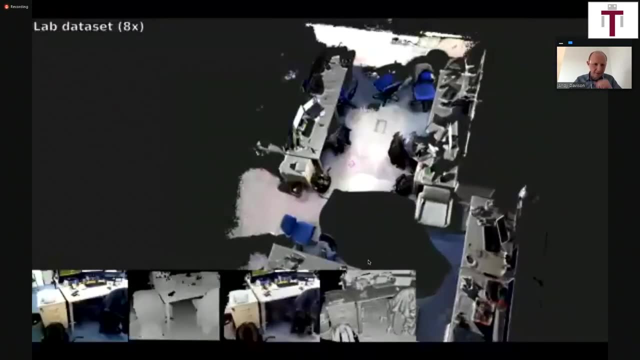 lab about five years ago, led by led by tom wheelan. so here we see a real-time dense slam system here. so the input to this system is what you can see in in the bottom left. let me just full screen this. so in the bottom left you've got, uh, the live kind of image stream from a color camera and 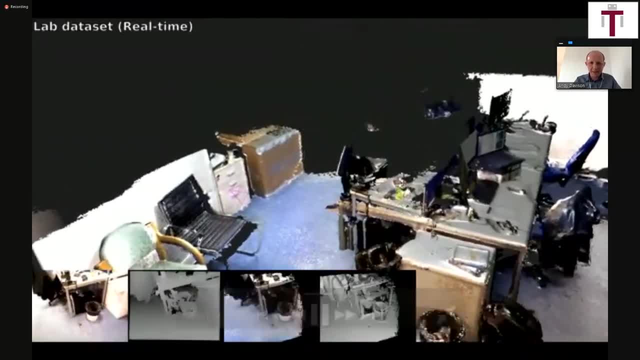 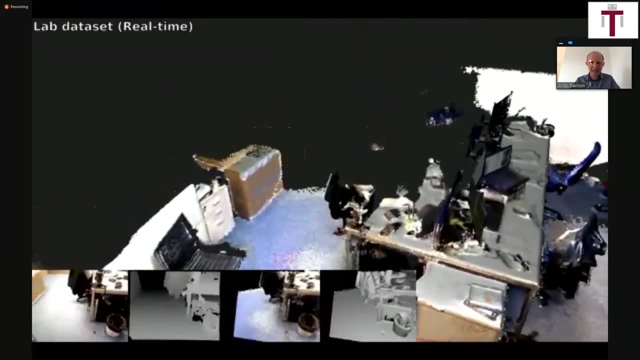 the live depth stream from from a connector- depth measurements, and then what we're doing is both tracking the camera and then fusing all of the information into a dense scene model in real time. so there's many possible ways to represent dense scenes in in this particular system, we're 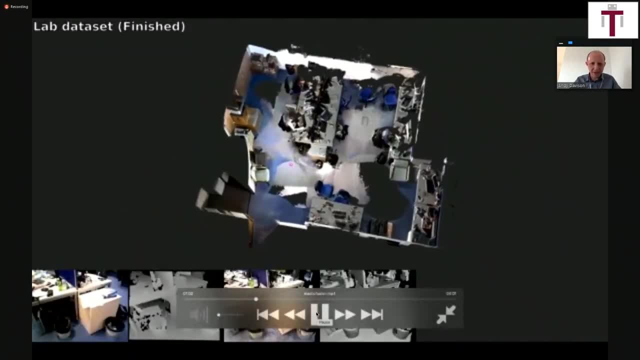 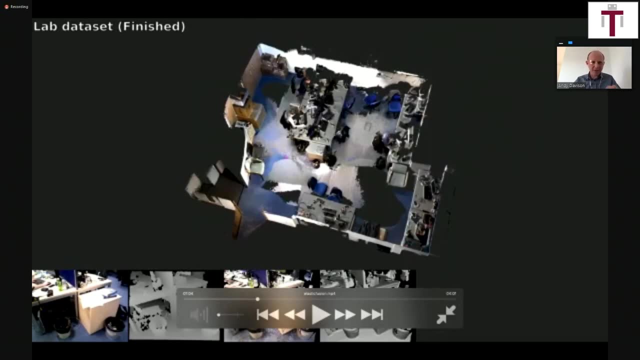 using a representation called surfles, that that means that the representation of the scene is basically a cloud of little discs. so these are points that also have a kind of orientation and and a size. so they're representing uh, small, uh discs. and if you kind of look at the image here, 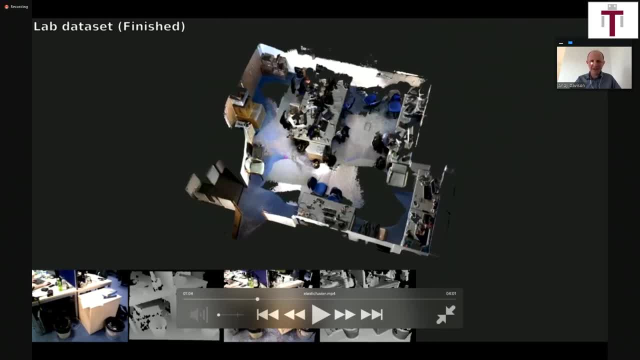 smush enough of them close together, it looks like a continuous surface. so that's one of several options for representing dense geometry. a particularly nice point about um the uh, the the circle representation is is fairly efficient and that enables elastic fusion to do loop closure. so this means that when the camera comes right round, 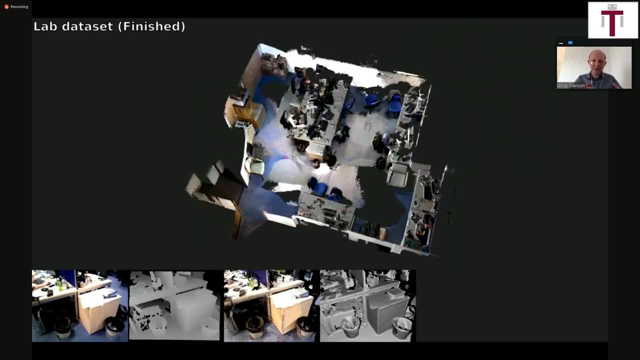 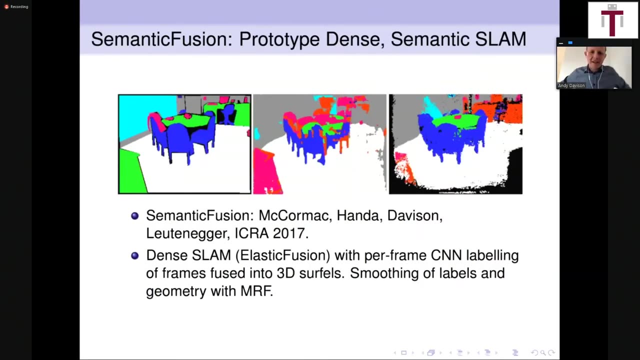 and revisits old parts, parts of the scene, it's able to make corrections to the map so that the map stays consistent, which is something that wasn't possible, for instance, in the original connect fusion system. um, so I think the next, uh, and probably the most recent sort of real advance in real-time visual 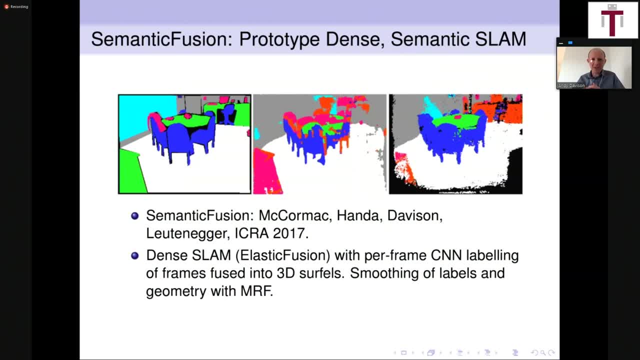 slam is is what's very much going on at the moment, which is trying to add a semantic layer. so the map built in elastic fusion. it's very detailed but it's still just raw geometry in the end it's it's a cloud of points, so there's no meaning associated with it. so you know from from three orato. 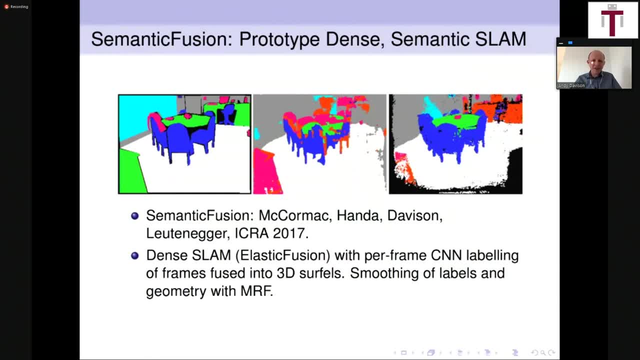 of points. so there's no meaning associated with it. so you know from from three orate of points. so you know from from three orate. you know from from three orate three or four years ago or a little longer ago, of course, the big kind of new technology coming into. 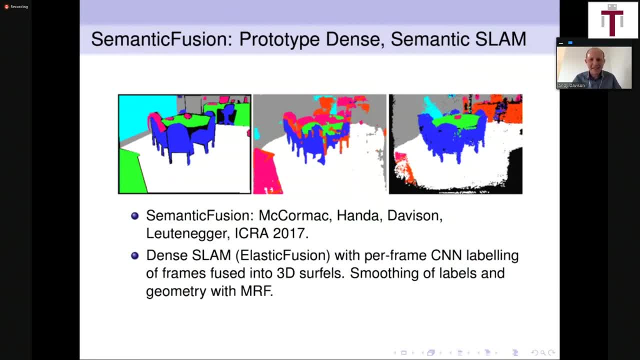 into slam is is deep learning and so enabled of course also by gpus, this capability to do um real-time uh labeling and and recognition. so we built a system called uh semantic fusion, which is aiming to do dense semantic mapping of the scene, and if i show you this video, um 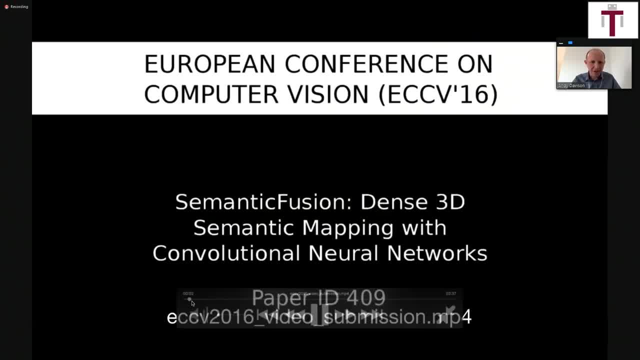 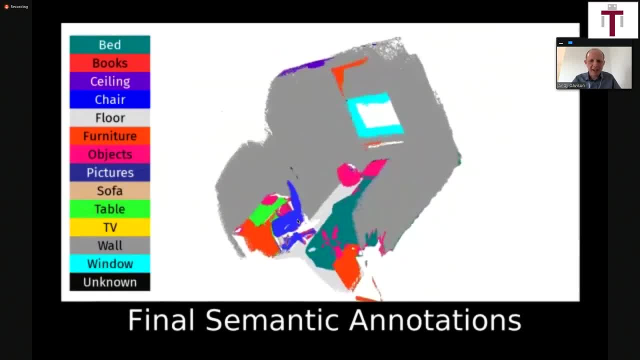 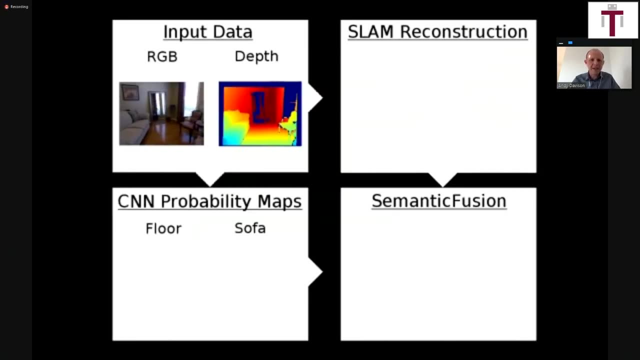 this is. this is what we're trying to achieve, so map a scene densely in 3d, but also apply labels to it, which represents our best estimates of the objects or type of objects that are present, and the way that this system works is actually fairly straightforward. um, so we have our in input data. 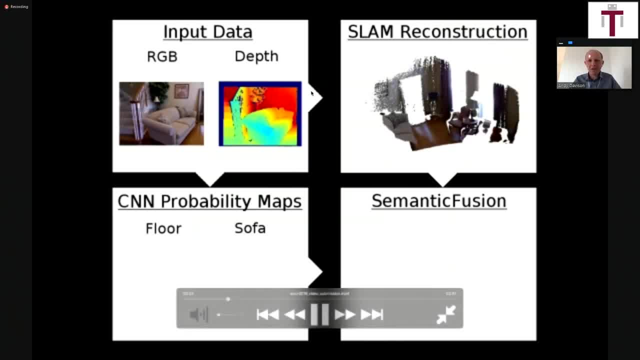 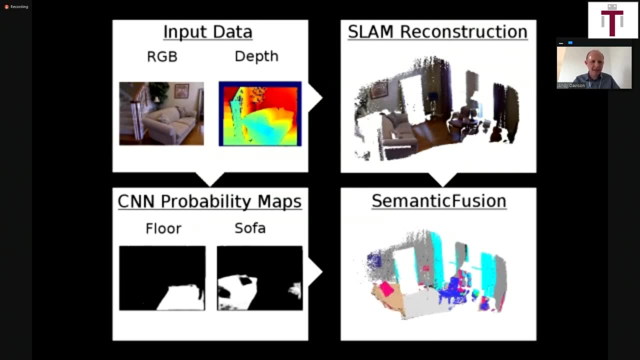 stream of color and depth images. they're fed along two pipe ways. one does slam reconstruction, so this is in fact the illustration of the system- searches the object we're working with and we can make a chart that shows which pieces of the object we use to see which images are in the image, the segmentation we have in the image. 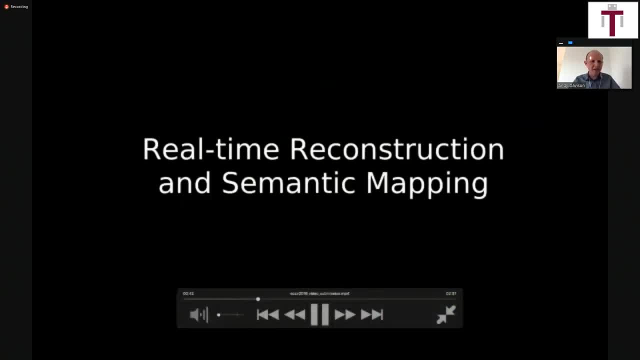 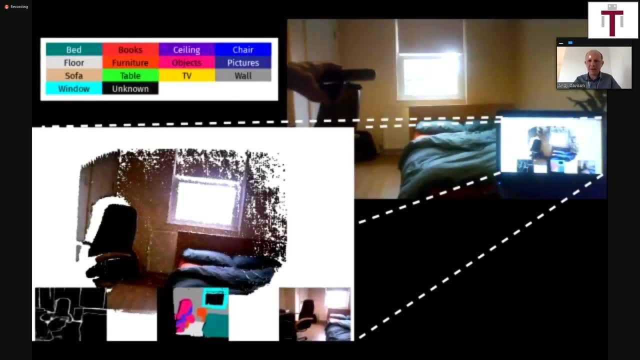 sampling technique, which is kind of a R&D approach to it, so we can make terms that are consistent with the image. that we're working with- and that's what we're interested in is basically a whole of a map set up for the image, for every single image, and we can then 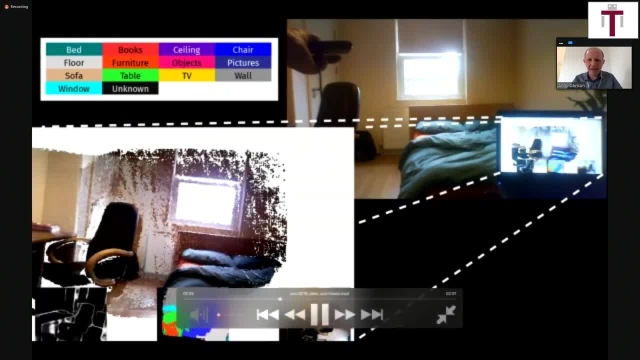 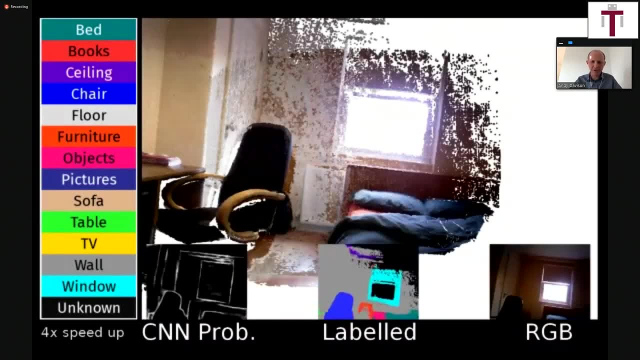 map it, for example, and look at the images. um, we see that, for example, in this circular image, we see that the image in which the image is labeled at one point uh, each circle in the scene over what it thinks the most likely labels are for that point of geometry in the scene. 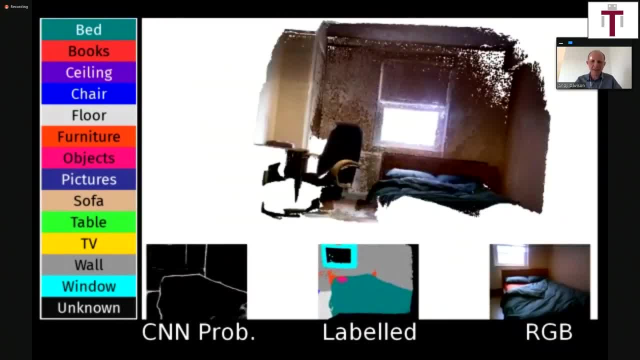 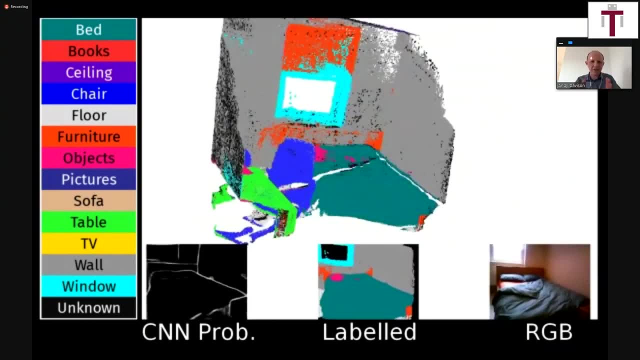 And the interesting point of doing this in a SLAM style is that the label for each point in the scene can gradually change and improve. So from one point of view you might get not a very good labeling of a particular element of the scene. It's quite 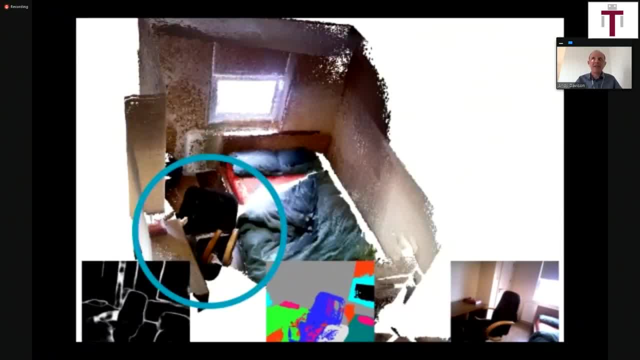 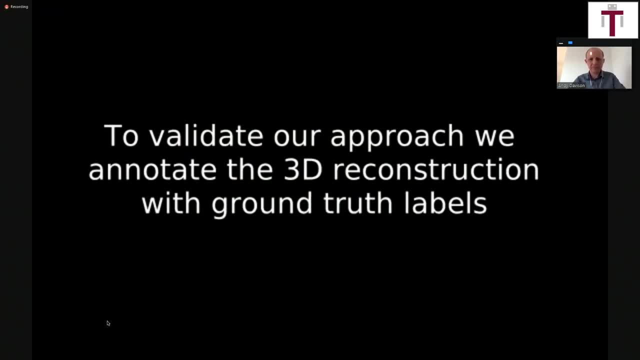 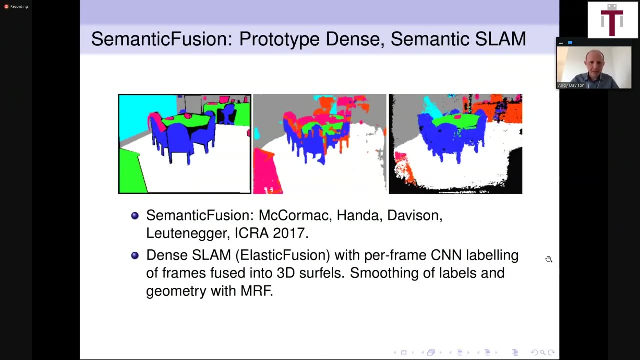 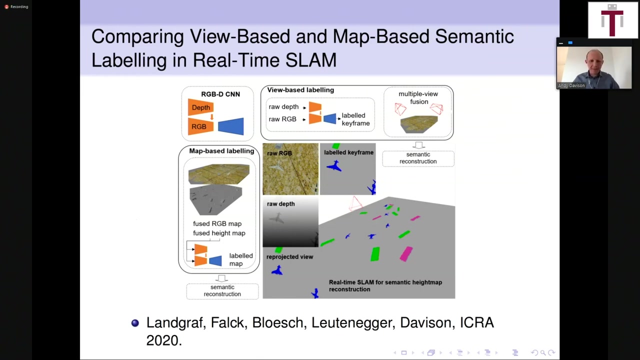 ambiguous, But when the camera moves to a better location, that can actually improve. Ray Abrahams SPLAT. So there's just one paper I would like to mention in connection with that. so something that we've published which just will appear in the ICRA conference that will be signed. 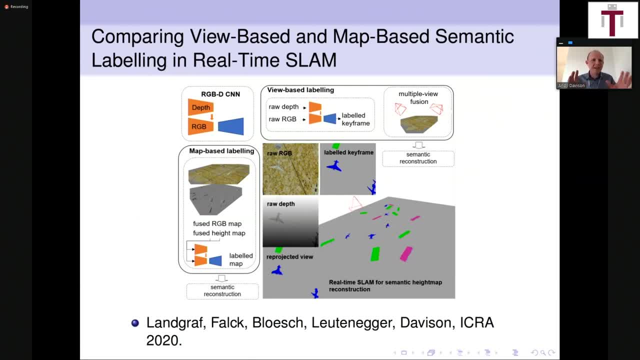 in the next month or so. So these systems that label scenes based on CNNs. I think there's two interesting ways to go about that. One is the view-based way that we took in Semantic Fusion. ou can label every view in a wesическая ylata style. it's just the same One I'd like to go about. 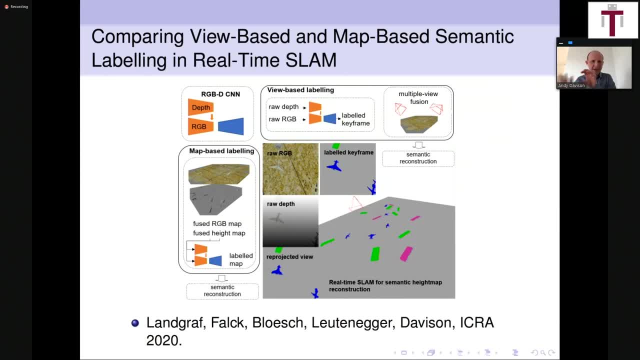 there's two ways to go about that. One is the view-based way that we took in Semantic Fusion: view in a view-based way, as as the camera moves around, and then try and fuse all of those labels into the 3D representation. Another possibility that we're seeing a lot of nice systems based on. 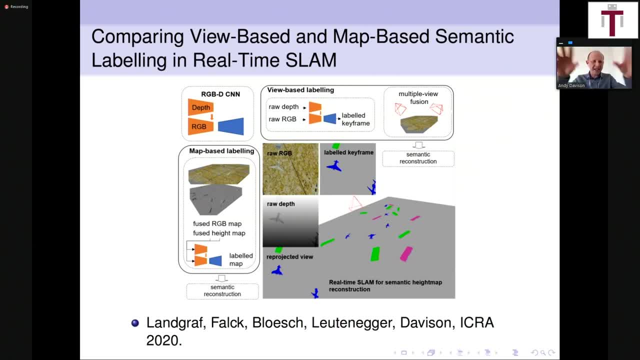 is build the whole map and then use something like a 3D CNN that can take in that whole 3D map and try and label it in place. So there's very interesting pros and cons between those two methods. One is immediate, it gets to work on the raw data, whereas the other one gets to see. 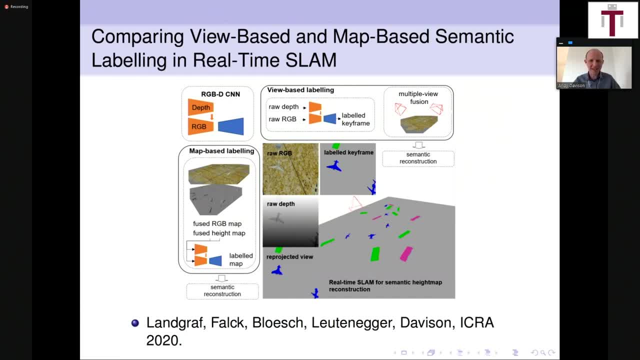 the whole map in one go and can take account of whole context and that kind of thing. The computational characteristics of those two things are also very interesting to study, So have a look at this paper here if you're interested in that. Okay, so we've got this range of systems that have gradually got. 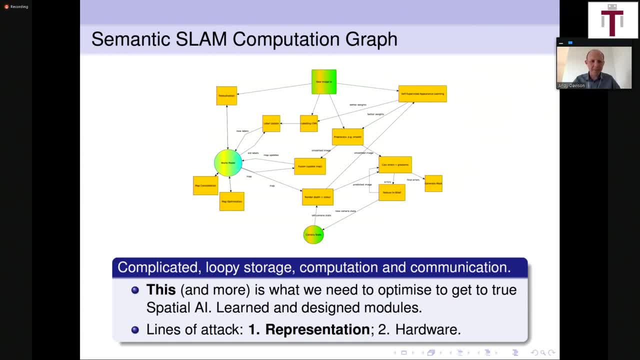 more and more popular. So we've got a lot of systems that are more and more popular. We've got a lot of systems that are more and more popular. So we've got a lot of systems that are more and more popular, More advanced. One way of thinking about what happened there is that we've essentially been 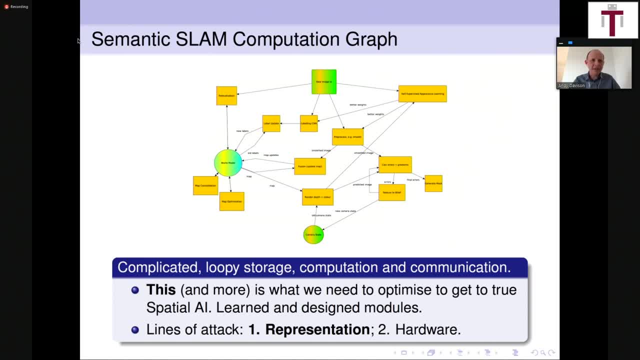 gradually throwing more and more computation at this problem, And we've seen progress because of that. So where does that actually take us? So is this useful steps towards this spatial AI goal that I was talking about? So I find this picture quite interesting. So this is actually a kind of more or less a mock-up that I did, But 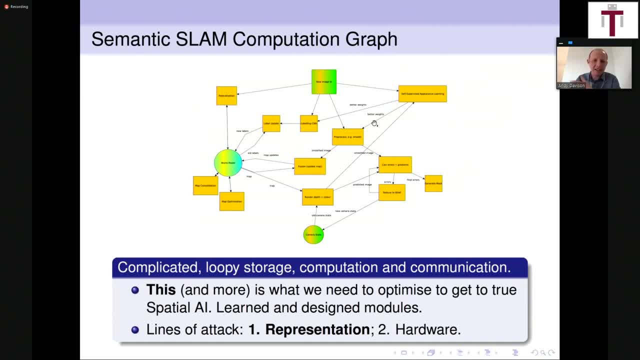 thinking about all of the computation that's happening in the system like semantic fusion. So it's a pretty complicated system. We've got data sort of represented in green and then blocks of computation represented in yellow, And don't worry at all that this is a bit small. 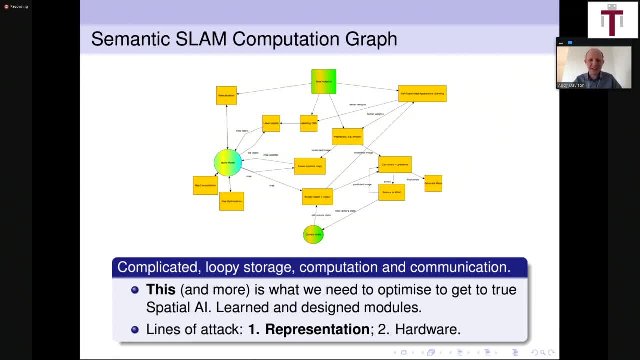 to read. All I want to get across is: this is pretty complicated. So there's labeling, there's tracking, there's fusion, there's map optimization, There's all kinds of things going on here. So how are we going to get this to run on tiny embedded? 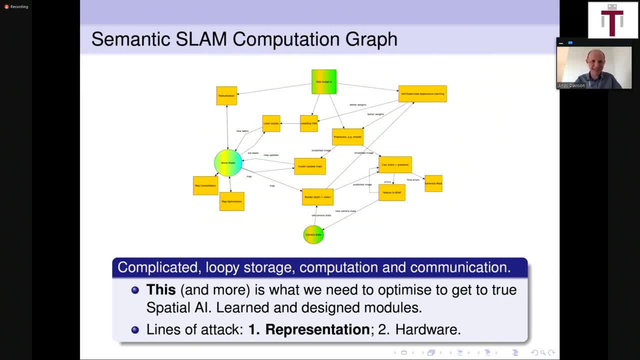 devices that weigh 65 grams and this kind of thing. That's what I'm really wondering: How are we going to kind of optimize this graph down to something a bit more manageable? So I think there are two kind of interesting lines of attack that we've been following in our lab and which I'm 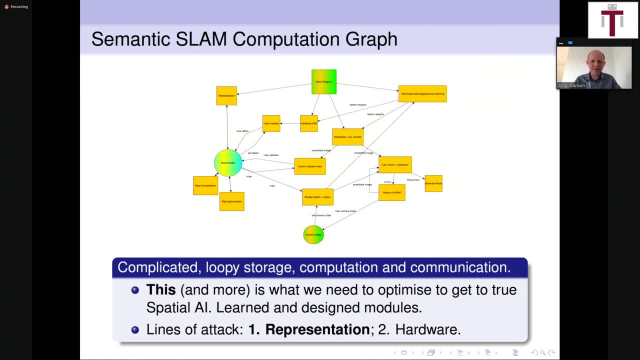 going to take you through next. So one is to really think about representation. So this really means, if you look at something like semantic fusion, we've got these huge representations of detailed things like. we've got image maps of labels the size of an image with hundreds of thousands of entries. We've got maps of circles. So I think 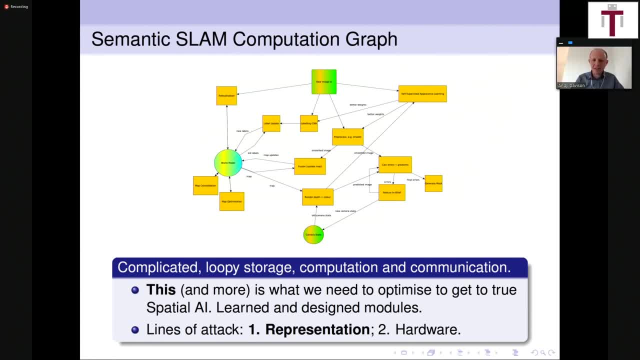 the map of the room that I showed you in Elastic Fusion earlier has something like 5 million circles in it, So we've got lots of big amounts of data moving around this graph being worked on parallel computation where we can, But the current implementation of a system like this is also some parts of this work on the GPU. 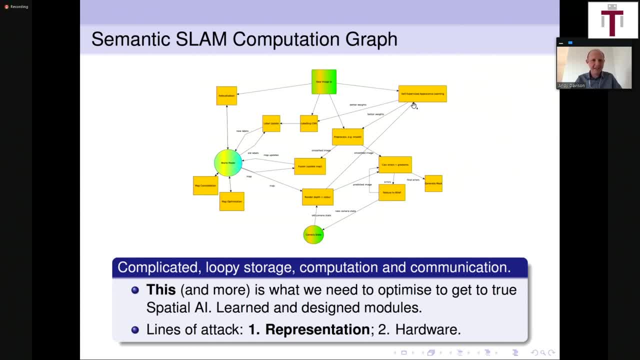 some of it's running on Encoder, some of it's running probably in TensorFlow or PyTorch. Other significant parts are still running on a CPU: a lot of data transfer and so on. So what if we could kind of simplify a lot of those representations? So can we turn the 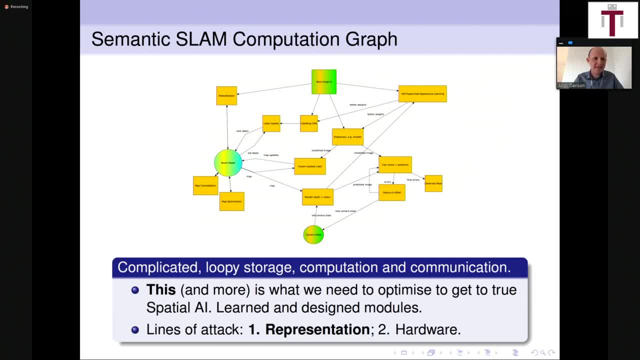 mix of these huge- you know, dense- blocks of data into much more simple things, then we seem to get to something which would be much more efficient. The other line of attack, which I'll talk about a bit later on, is: can we use custom computing hardware to help us with this? 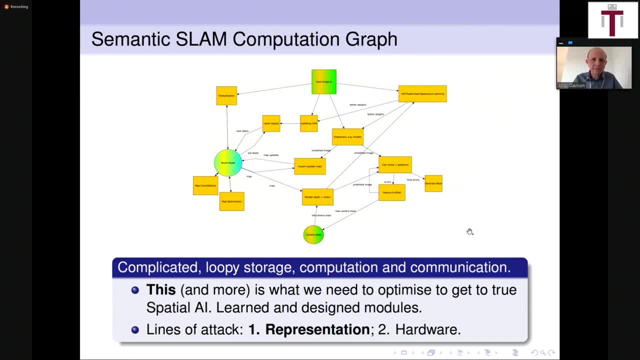 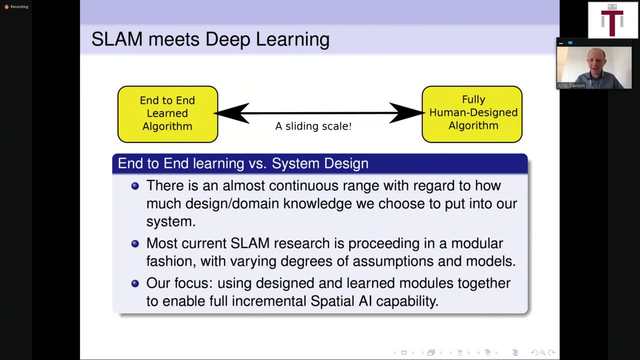 I'll come back to that later. So firstly, thinking about representation, we've done various bits of work in our lab, And most of this has increasingly been using elements of of machine learning. And yet we've been able to see that there is an interesting change in the same quality of the work that we've done in our lab, And most of this has increasingly been using elements of machine learning. 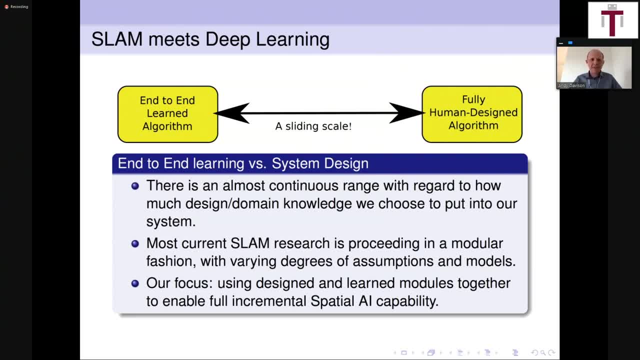 So we're really trying to say: are there, you know, representations or algorithms within our complicated SLAM systems which can be replaced by something learned which will have kind of simpler and probably more generally abstract and interesting properties? So that brings me to a general discussion, which I'll try to tackle briefly, about SLAM and deep learning. So I think everyone working in SLAM has been thinking a lot about this in the last few years, as in most fields of AI, of course. 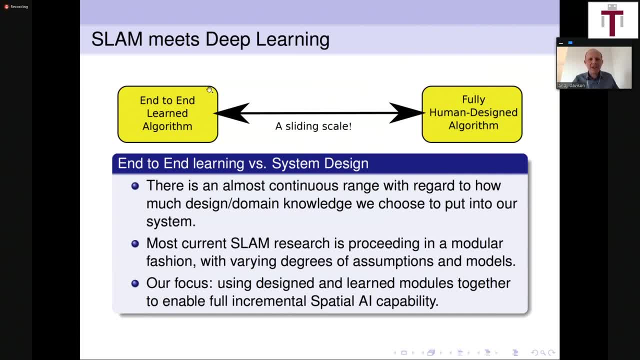 My point of view on it is that we have a kind of sliding scale here, almost a continuum between things we could do, where on one side we've got fully hand-designed algorithms and certainly the early systems, The systems that I showed you, purely geometric systems. they're completely hand-designed, you know, monoslam or elastic fusion and so on. 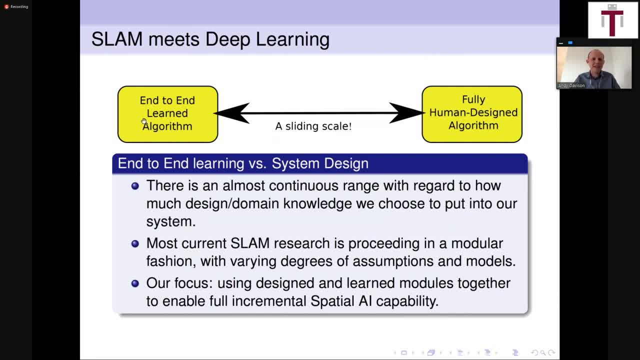 At the other end of the scale, we've got this possibility of fully end-to-end learned algorithms. So I think if you speak to someone, let's say a deep mind, they'll probably tell you or you know they might believe that you know why would we ever hand-design anything, any part of an algorithm? 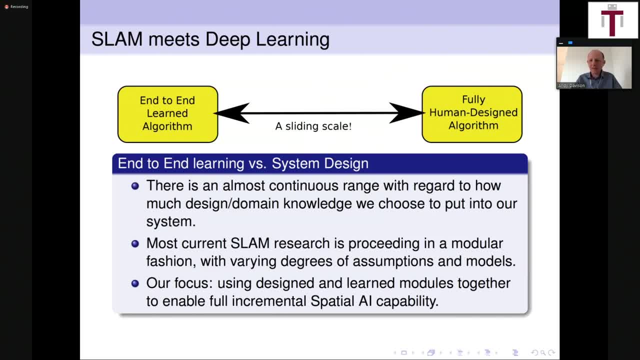 Why don't we just learn? Why don't we just learn everything end-to-end? And I'm not saying that they're wrong. I think in the long term that may well be exactly right, because every time a human designs representation, you put some limitation that an artificial system may not need. 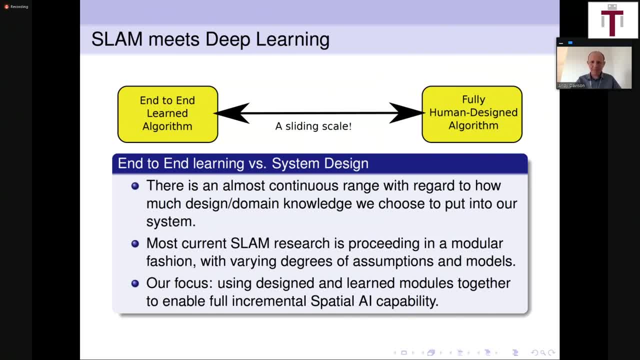 But I think that the way that almost all of us are proceeding in trying to build systems that work is a modular combination of hand-designed elements and learned elements, And I think there are two key ways to do that. Either we can start with our hand-designed algorithms. 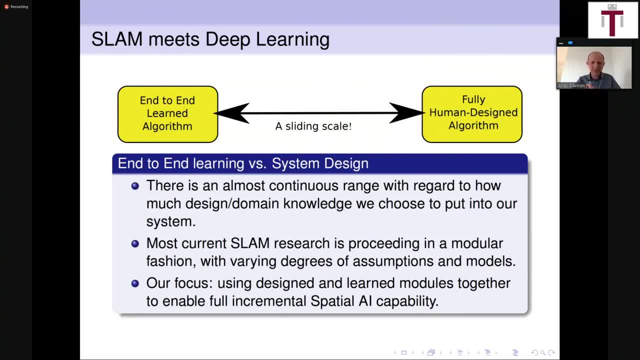 We can start with our system, maybe the one I showed you in the graph just before, and replace some of those blocks with learned things which work better but also maybe have some sort of abstraction and efficiency. The other is to start off with a big neural network and say this is my system, but gradually kind of impose structure on that network and say: is this not a completely general perceptron? 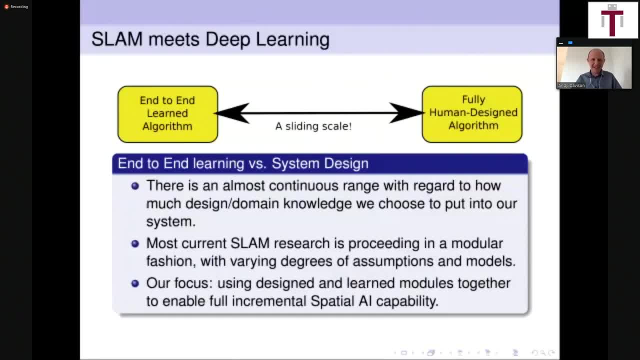 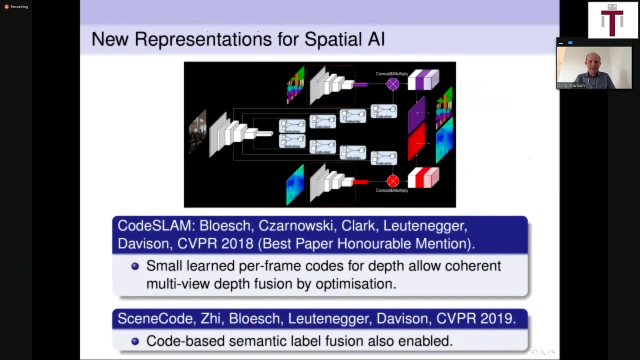 It's. you know, there's structure, There's things like spatial transformers and so on in there Which force it to do certain things. I see those things as very similarly related and will ultimately meet in the middle. Okay, so, having said that, let's talk about some of the work we've been doing on representation in our lab. 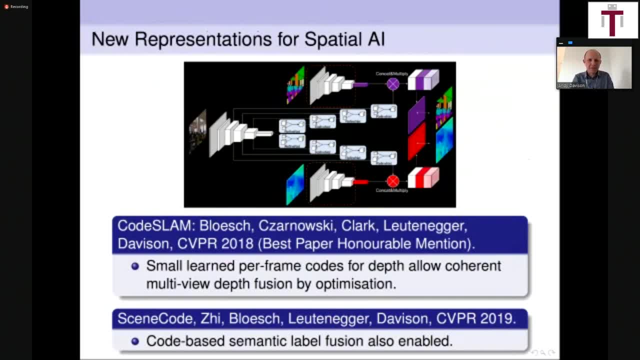 So the first sort of category of projects I'm going to talk about was started by a paper we had called CodeSlam back in 2018 and was followed up closely after by a paper called SceneCodeSlam. So don't worry too much about the details of this kind of network diagram I'm showing you here. 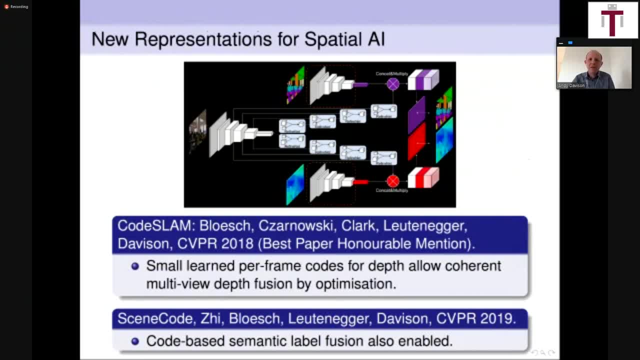 But the key idea is that we want to encode the variation in dense depth we can see from a single camera in terms of a way that what are the main variations there? So if you just think of a dense depth map, in principle You know, at vj resolution that has 300,000 parameters for the depth of every pixel. 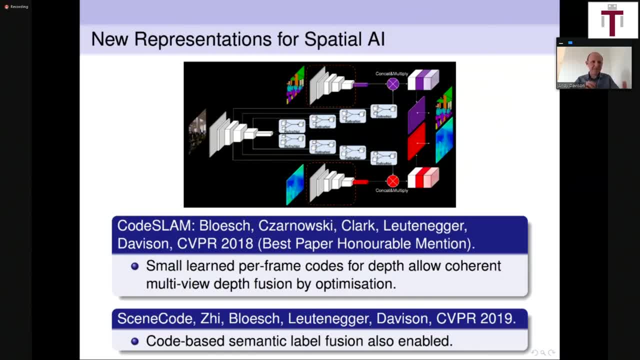 But think about how many people are stored. But if you point a camera around at real scenes there's actually a lot less variation than that. So most real scenes tend to be made up of continuous objects and surfaces, So there's a lot of sort of structure in the space. 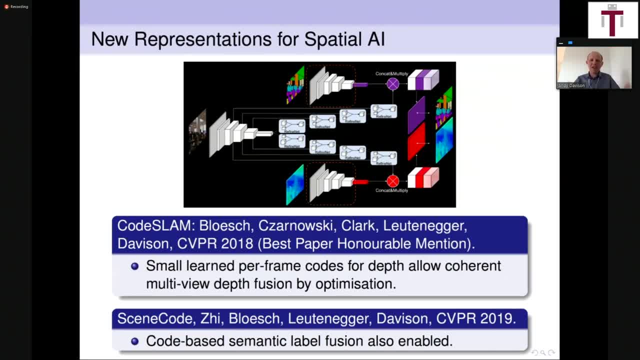 So in CodeSlam we do some machine learning. We have a data set of, in fact, synthetic indoor scenes that we train this on, And we learn an autoencoder which is able to go from a sort of small bottleneck to generating 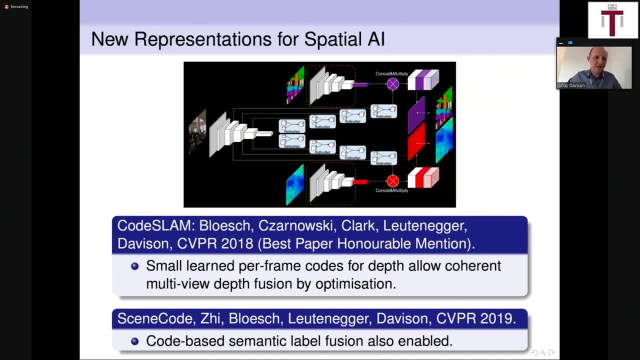 likely dense depth maps. So with a fairly small encoder of maybe 32 parameters, we can describe the variation that tends to be present in dense depth maps. So there's more details to it than that. But what that essentially enables is, when you have a camera moving around, a scene from 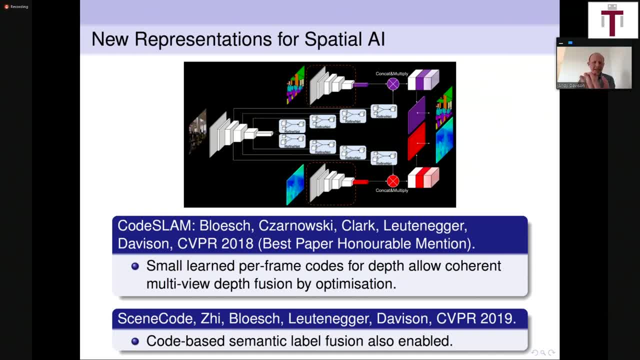 each single view you can make an initial depth map. So you can make a dense depth prediction. But as the camera continues to move, you can then optimize multiple dense depth predictions against each other. So by optimizing the codes of two of these dense depth maps, we can adjust them to try. 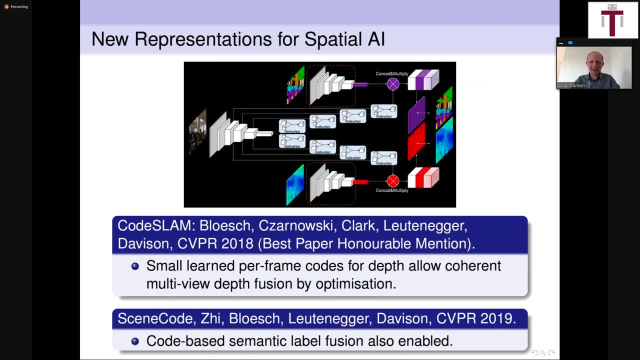 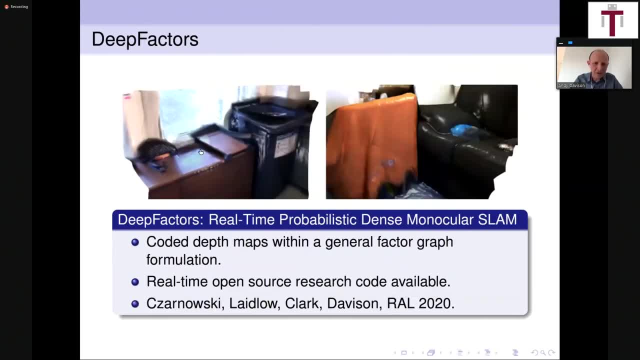 and bring them into alignment, But we will only be adjusting them within the space of things that we think are feasible, given our data set. So let me just show you a video here. So, in fact, we've recently published a paper called Dense Depth Prediction. 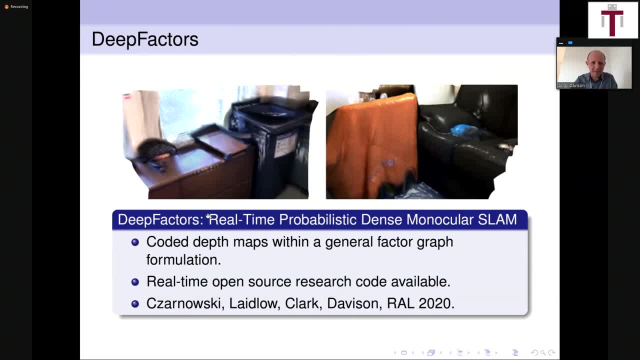 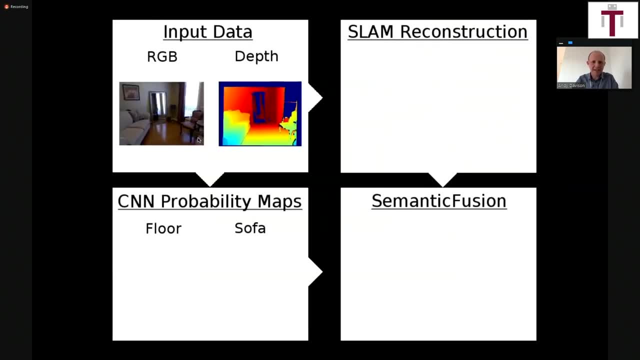 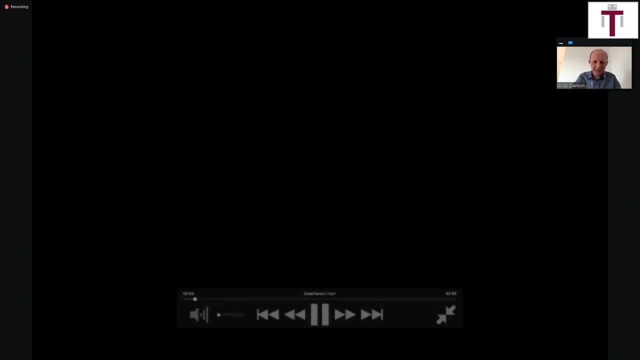 It's a really interesting paper. It's a really interesting paper. It's about deep factors and there's real time open source research code available based on this paper, which is an implementation and extension of the CodeSlam idea into a more general SLAM system. 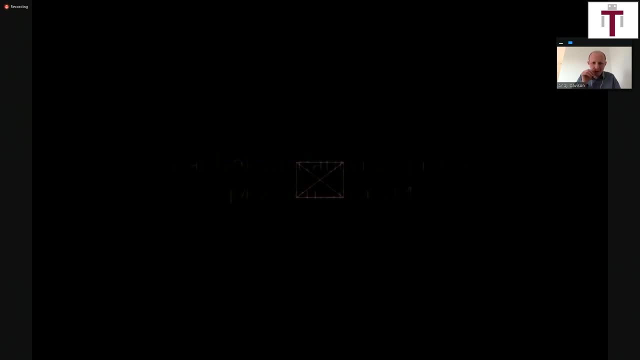 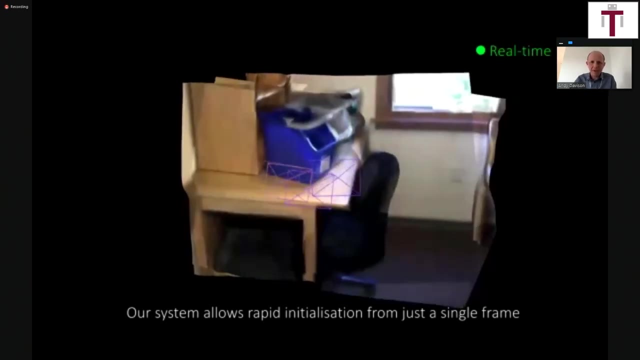 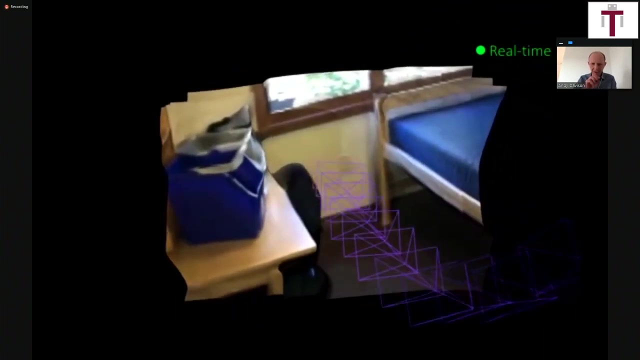 So just to give you an idea of how this works. So remember that in this system we just have a monocular camera, So there's no depth camera in this system. So as the camera moves around, you'll see that Every few frames we add in a new part to this representation. 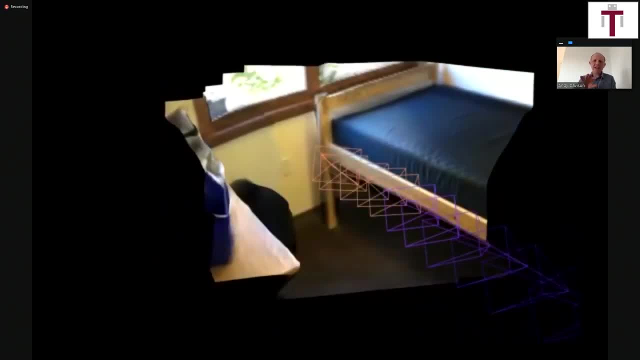 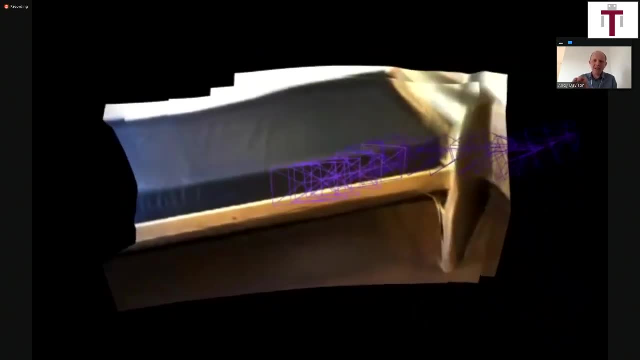 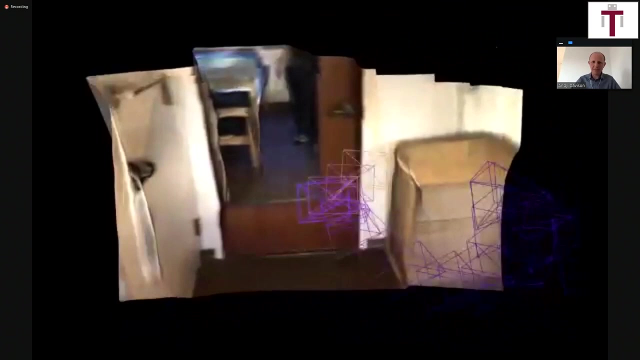 So we've got a new key frame. We immediately get a dense depth single view depth prediction from that frame, But then we're able to optimize it against the other nearby frames to try and produce a larger and more consistent overall 3D map. 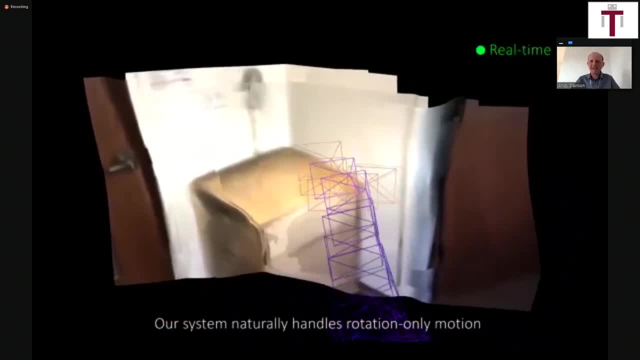 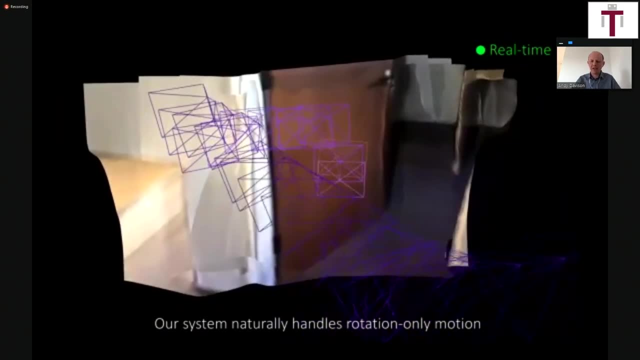 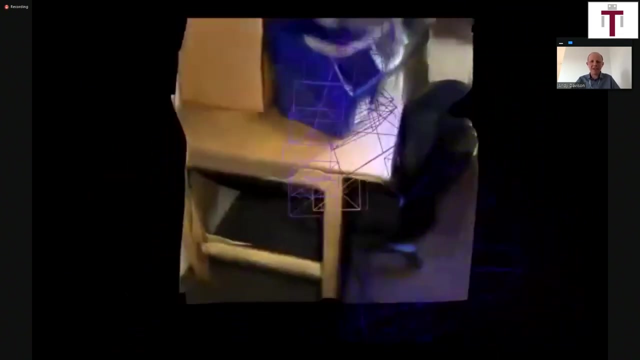 So here we're able to do jointly optimizable dense visual SLAM within this coded subspace, so just from monocular video input. So of course, subject to the things you would normally assume about a system that includes machine learning, that it will work fairly well within the scenes that are similar to. 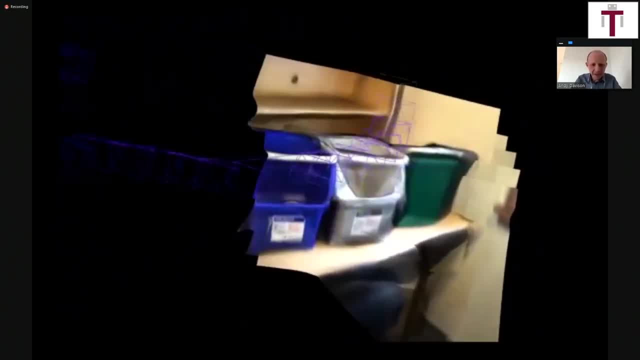 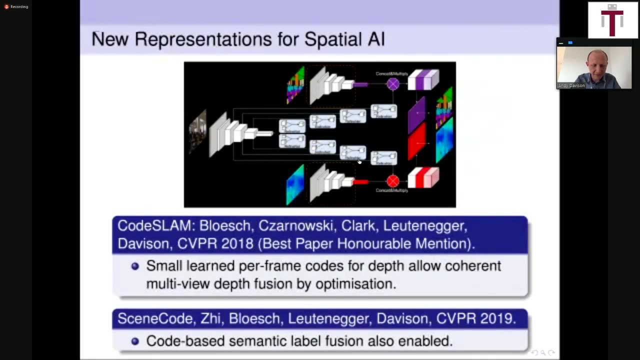 the scenes that it was trained in. But please have a look at that and try the code out. if you're interested, I'll just very briefly show you this and the other videos. So this is from the scene code system. So this is from the scene code system. 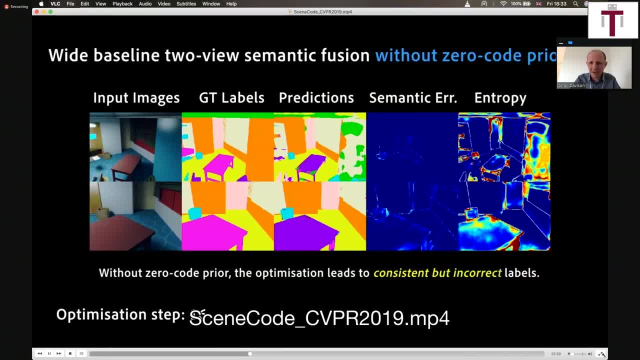 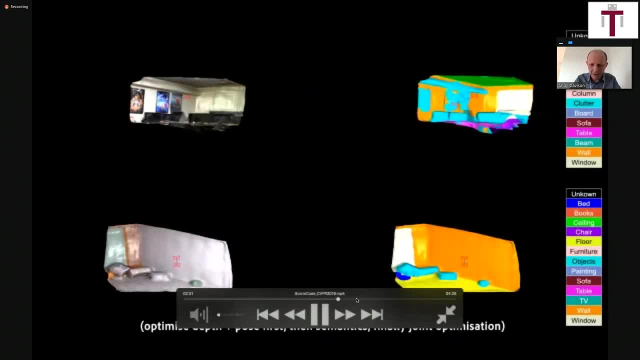 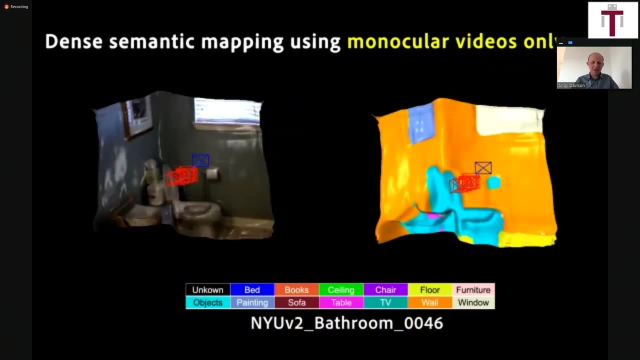 So this is showing that we can use very much the same idea of code optimization not just to deal with geometry, but also to deal with semantics. So here we have a video where our goal is to jointly estimate both the dense depth of this scene. 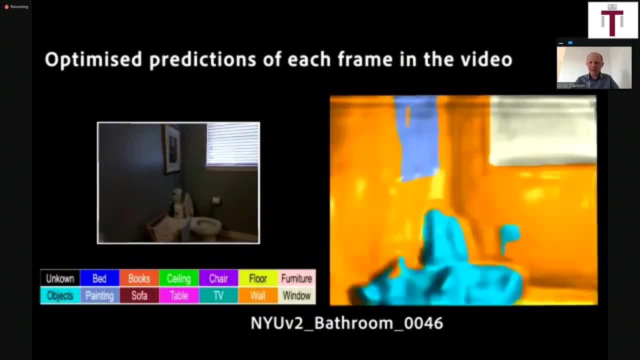 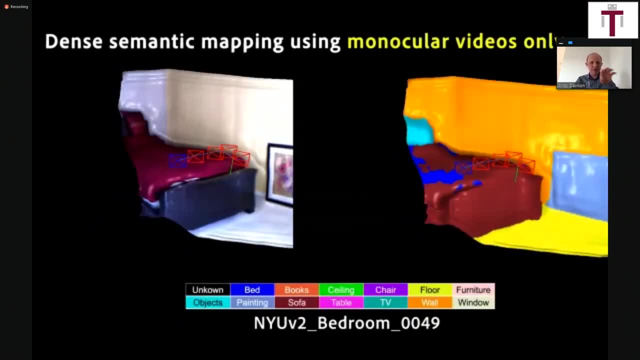 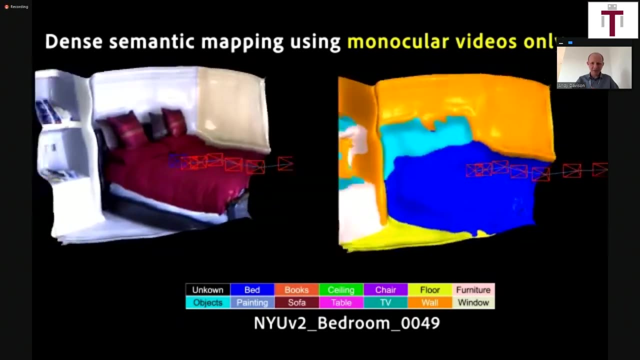 and also the semantic labels. But the way that we're basically combining multiple views now to do label fusion is not like in semantics. So this is the semantic fusion where we were just doing per pixel averaging pretty much, which gives us sometimes this quite noisy looking results. 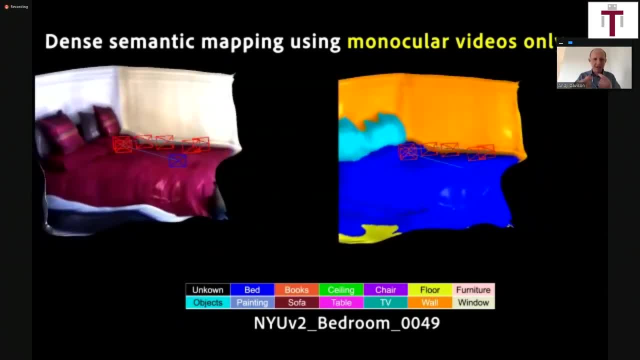 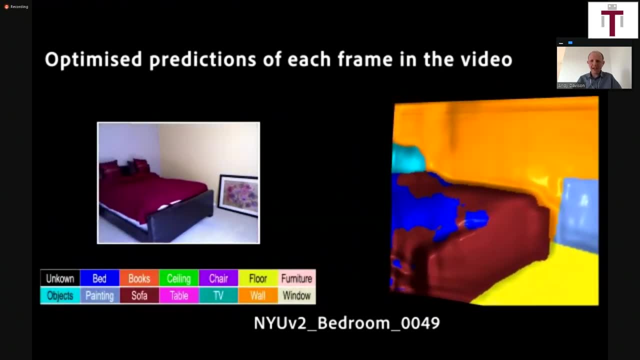 Here we're doing label fusion by code optimization, So the labels in each view are able to change, but they will only change within the space of feasible things that we are familiar with. So therefore they'll tend to change in this much more sort of smooth and coherent way. 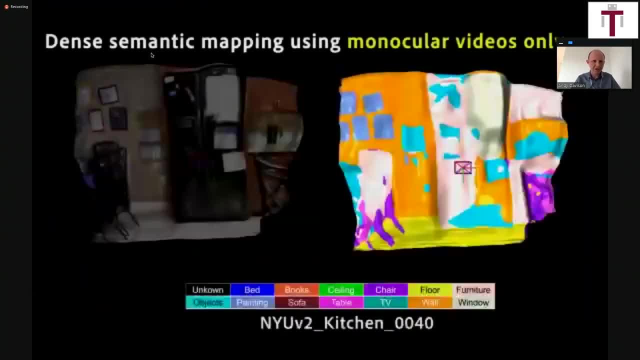 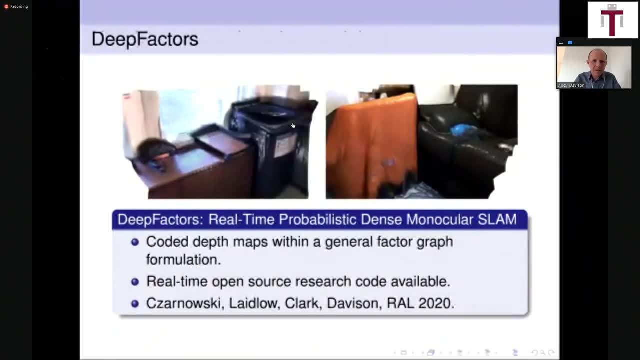 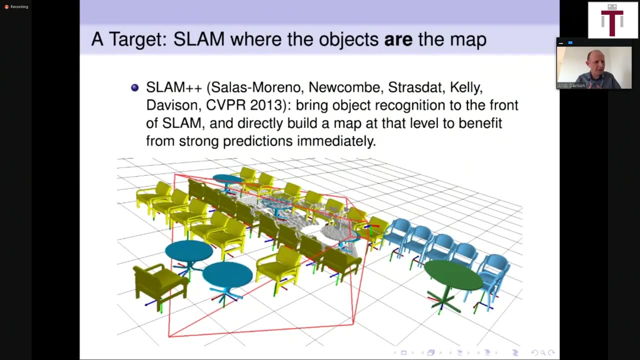 So it will tend to change the label of a whole region, such as an object for instance. So those systems use learning to kind of encode the variation that's present in a whole scene. But you can see that there are some limitations there. 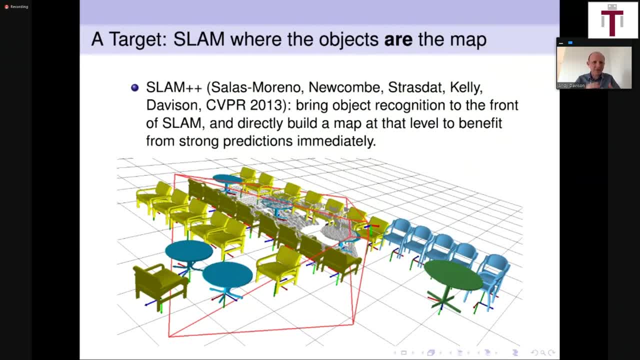 In some ways, maybe we're asking learning to do too much there, because a fairly small encoding cannot give us that much accuracy in representing a whole scene. So what seems to be the best way to do that is to use the same code that's being used here. 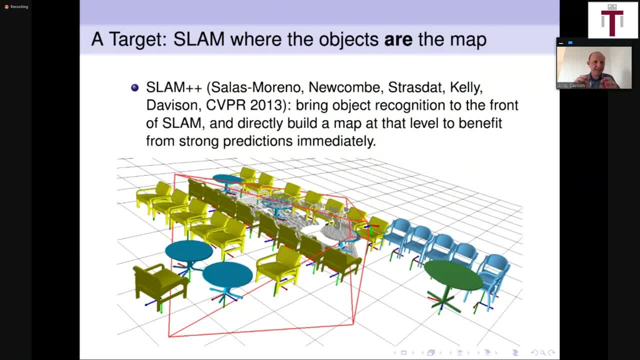 So that's the first thing. So the second thing is to use the same code that's being used here, And the third thing, the more sensible, is to focus learning down on things like objects. So, going back to about 2013,, we've been interested in this idea of can we actually build SLAM? 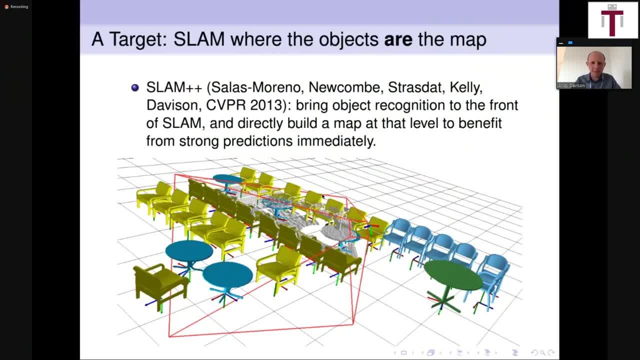 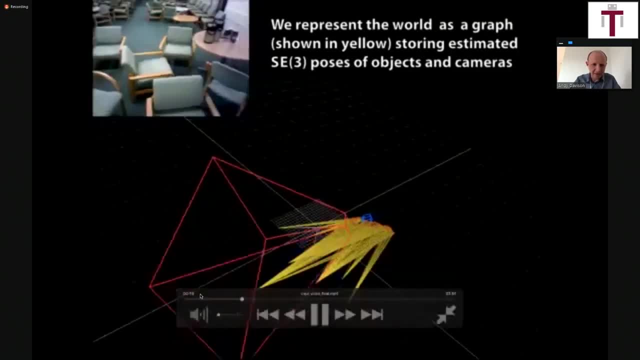 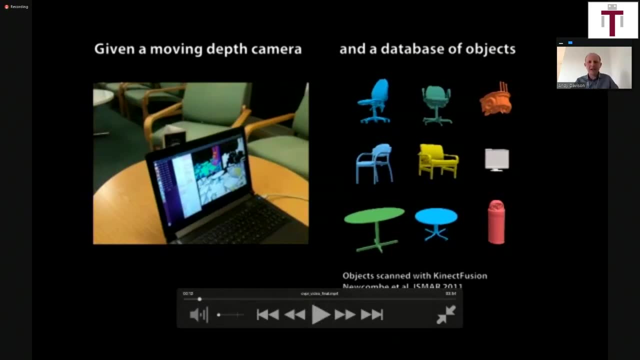 maps where the objects actually really are the map. So this system called SLAM++. it was this idea that we would come into a scenario where we're going to be moving a camera around and trying to map a scene, but we're not going to do bottom-up mapping of this scene and then try and fit semantics and 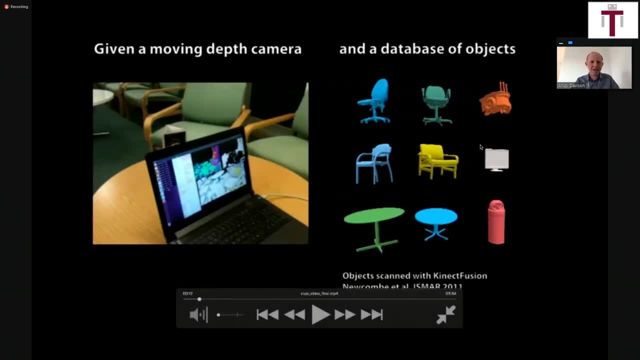 objects. later We're going to have a database of the objects that we expect to be present and we're going to try and fit those as soon as we can. So, as the camera moves around, the representation of the scene that we're building is a map that's directly built at the level of 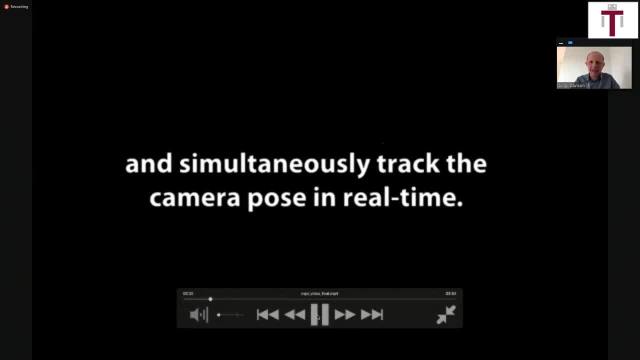 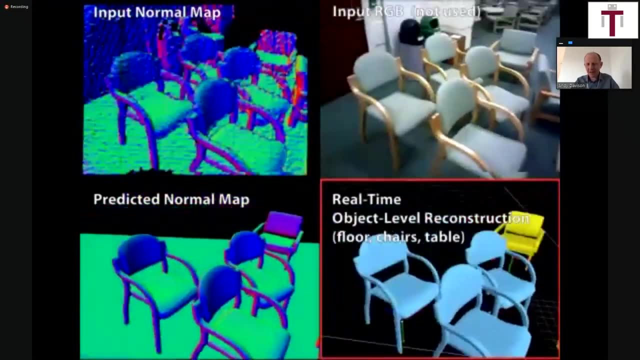 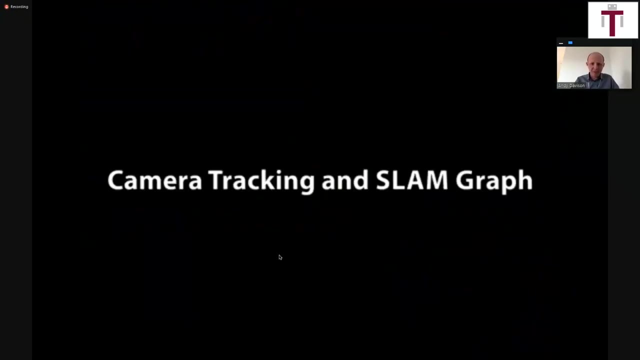 objects. So you'll see that the camera will move, and then down in the bottom right here you'll see objects kind of popping in to this representation. So here either an object is present or it's not present. There's no such thing as a sort of partially fused object. So this approach works. 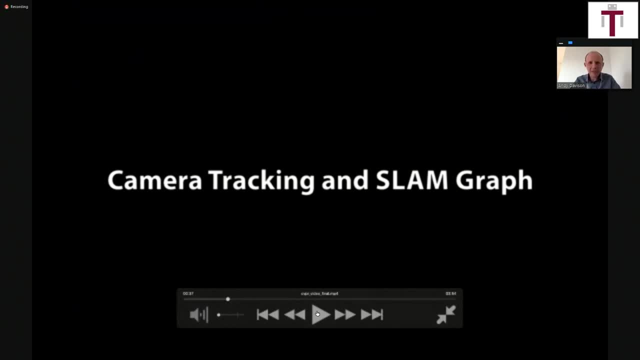 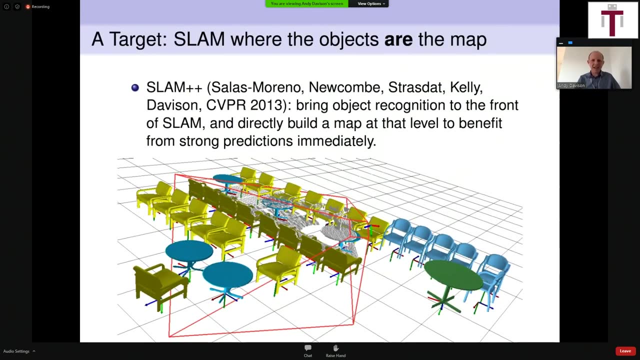 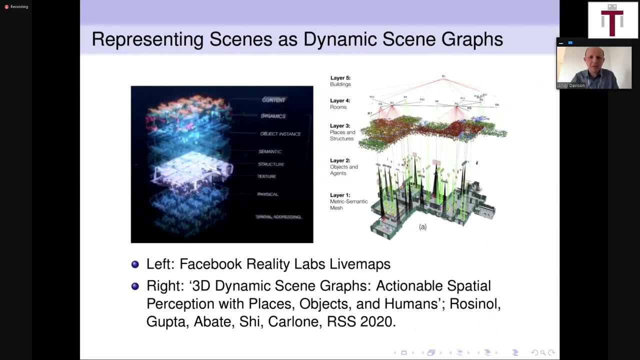 in the case where the scene obviously consists of a lot of instances of objects for which we have precise prior models. So here we have no ability to deal with objects that we don't know about in advance. So I'd just like to show this graph. So I think this idea of building maps out of these higher. 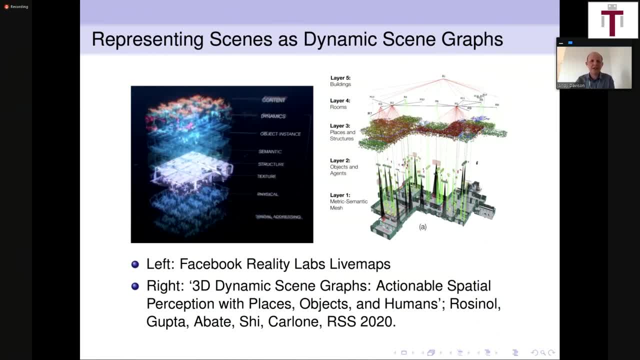 level, abstract kind of concepts like objects. I think this fits very much in with a lot of thinking that's out there in the community at the moment into building sort of layered scene graph type representations of scenes. So there's a couple of images here on the back from 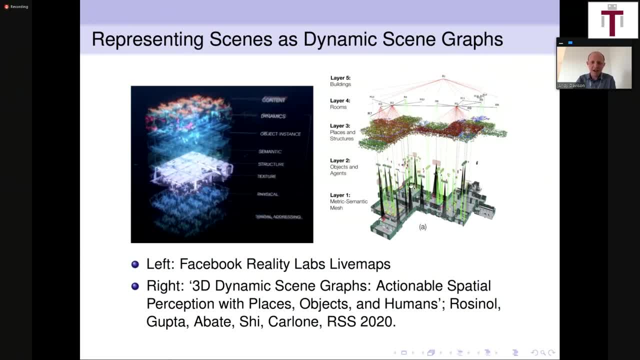 on this: on the left from Facebook Reality Labs, on the right from Luca Carloni's group at MIT on building what I think is really the right direction in terms of layered scene graph type representations. So in our lab we've continued to focus on object type representations. So let 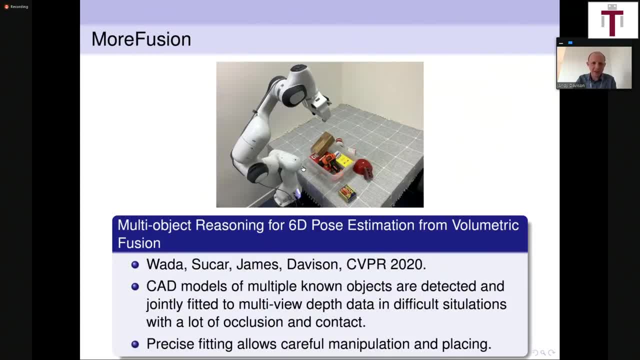 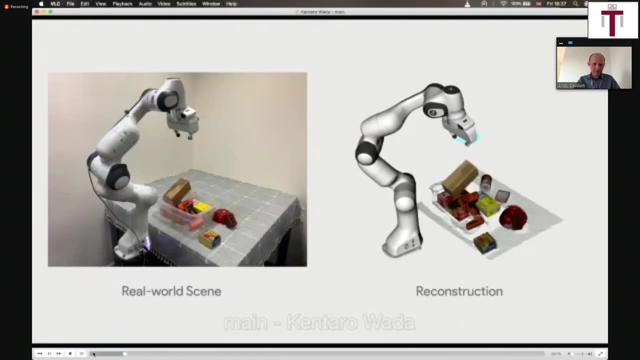 me show you a couple more things that we've done. So this one is called More Fusion. So this is a new system just about to be published this year at CVPR. So this is really the direct follow-up from the Slam++ version of our Feature imagination test tie gorgeous. 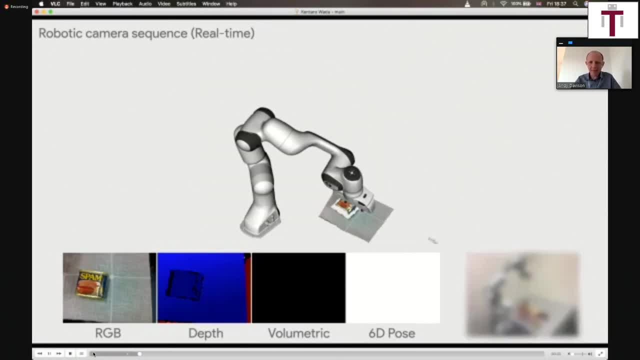 So I want to just move to the right place, Really our direct follow-up from from Slam++, in that we are coming to a scene in the situation where we do have prior high quality CAD models of the objects we expect to be present. But you'll see that here we're really turning our attention to what could actually be total, a reach specific to class. 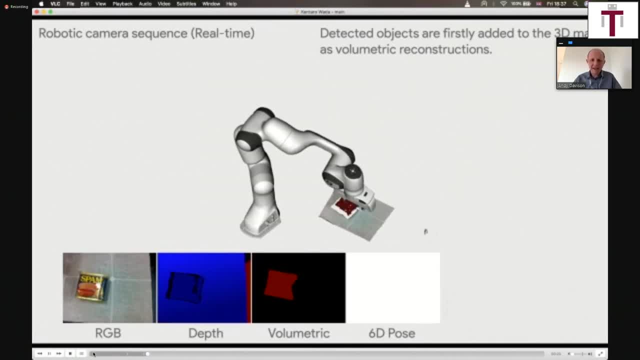 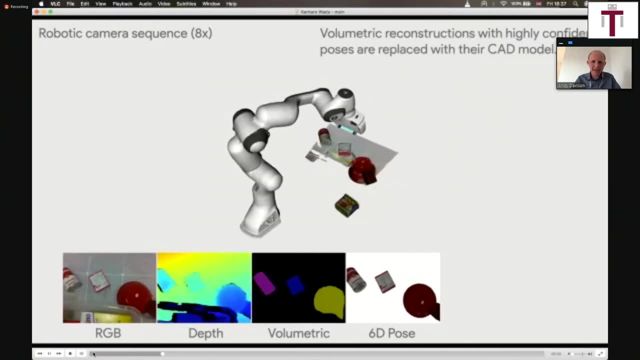 We're doing that now within a manipulation setting. So here we have prior CAD models of of this set of objects: v, fm, p, g fm. camera on the robot arm. the robot arm explores, it does some initial volumetric fusion of the scene. 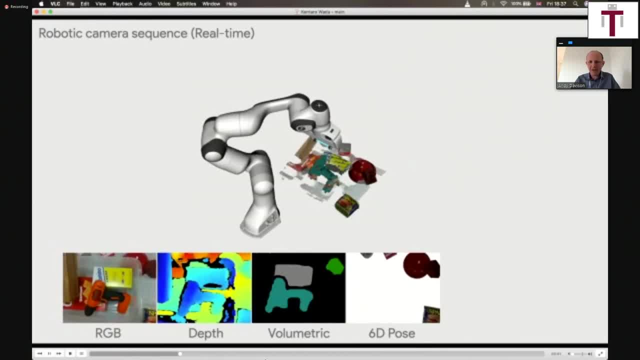 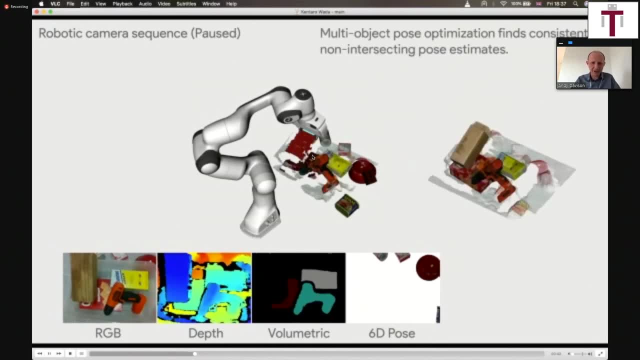 but then, as soon as it's able to, it fits precise 60 pose of object models to any objects it's really confidently identified. So here you'll see. it just found this drill in the center of the scene And then what you'll see on the right: 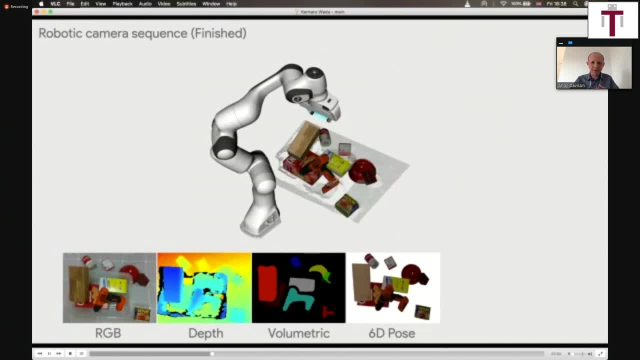 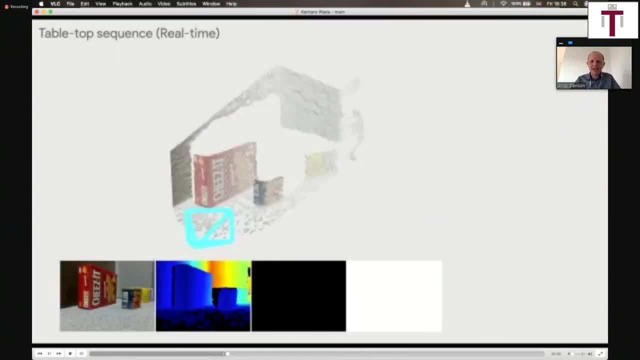 is, then it really jointly optimizes the poses of all these objects. So we want to deal with really difficult situations where multiple objects are in contact. they're occluding each other, So it's actually pretty hard to do single object pose detection in that situation. 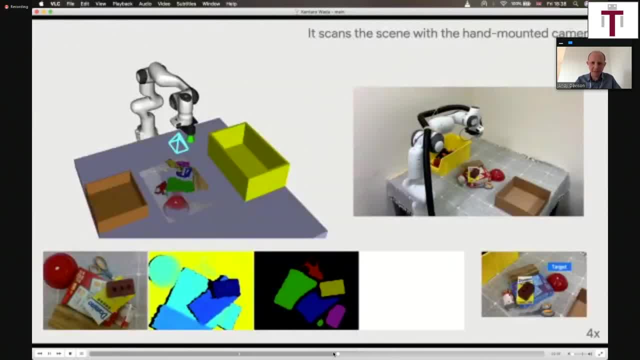 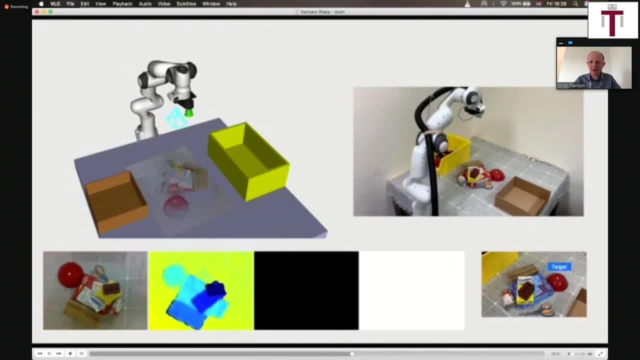 But if we jointly optimize the poses of all the objects, then we can do it. So here is now an application of that for a kind of difficult grasping situation. So here what the robot wants to do is actually move the rather large red box. 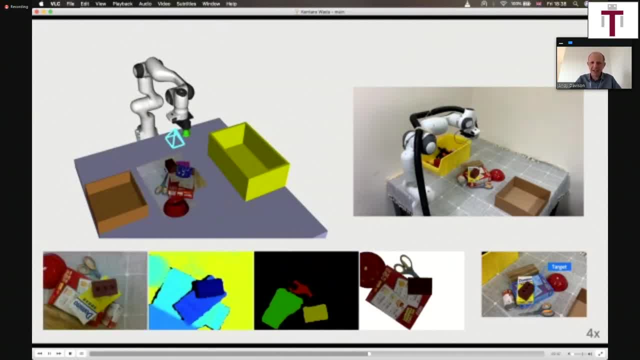 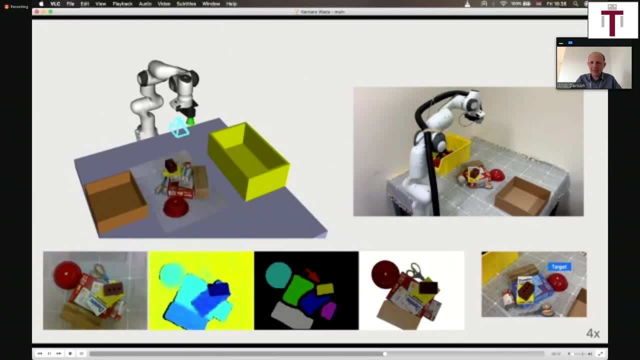 in the middle of the scene into the brain, So it's going to move the rather large brown box on the right. So first it's scanning the scene, it's fitting object models, it's jointly optimizing them And then, when it's confident, 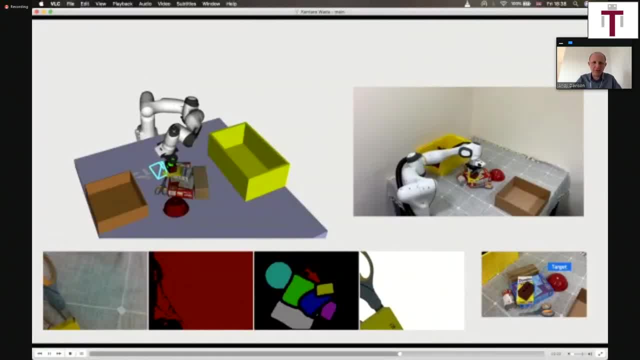 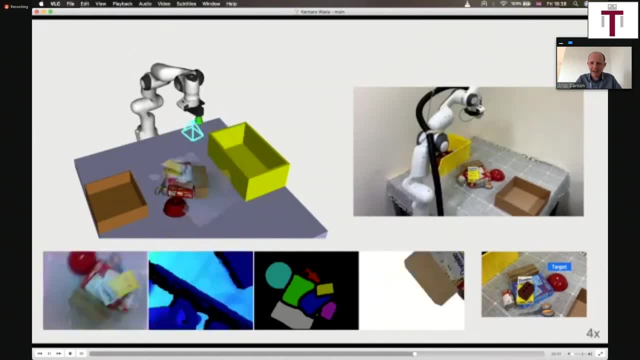 it decides on a plan of action And it realizes that to get to the red object it's going to have to move two other objects out of the way. So first it takes this object here, it drops it in the bin on the left. 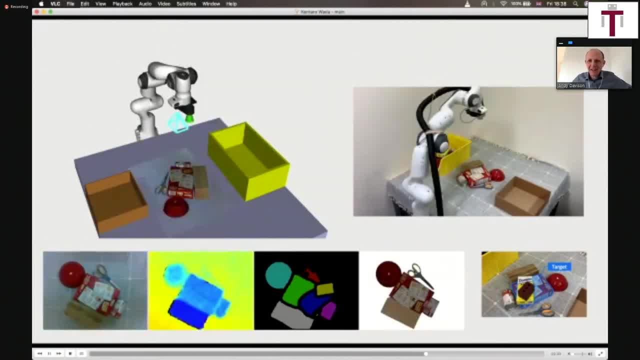 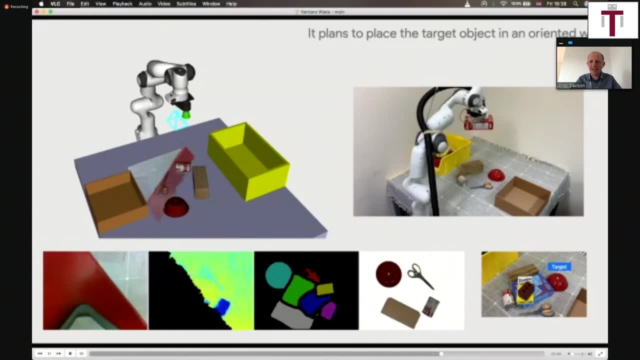 and then also this yellow box, And now it's able to get to the object that it's interested in. So it's moving and dropping, it's picking it up in a well-known pose and therefore it's able to then precisely place it. 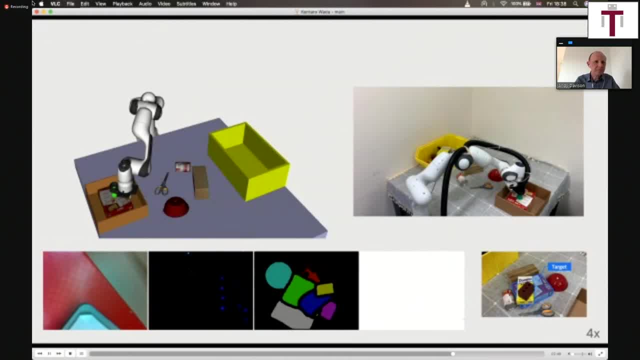 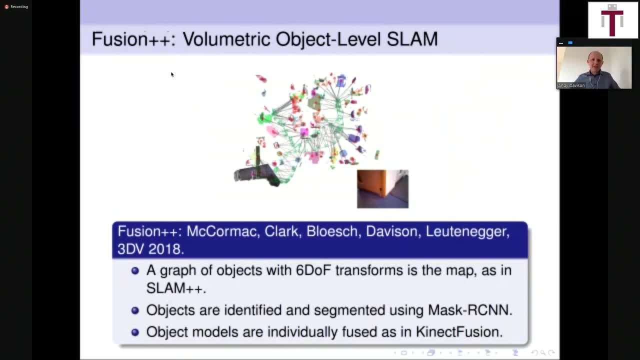 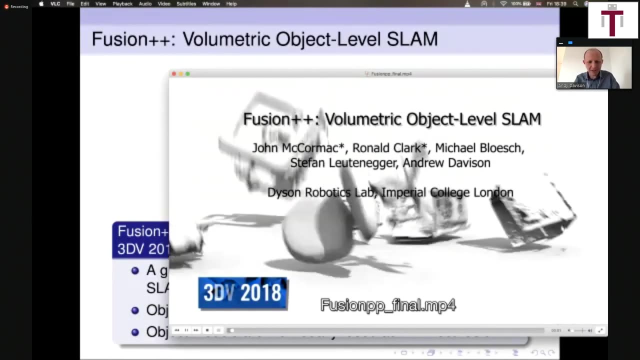 exactly where it wants it to be in the box. So another system I'd like to show you briefly. So it's very much along the same idea of an object-based SLAM system, but in some sense at the other end of the scale here. 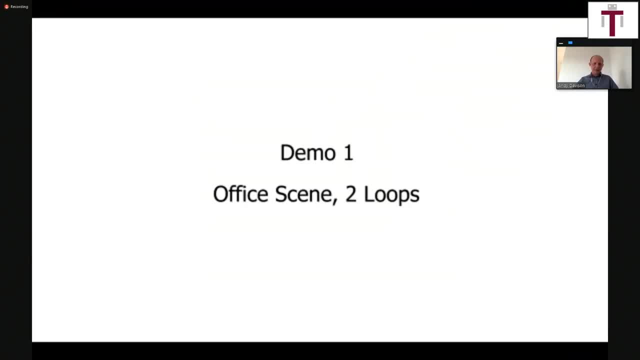 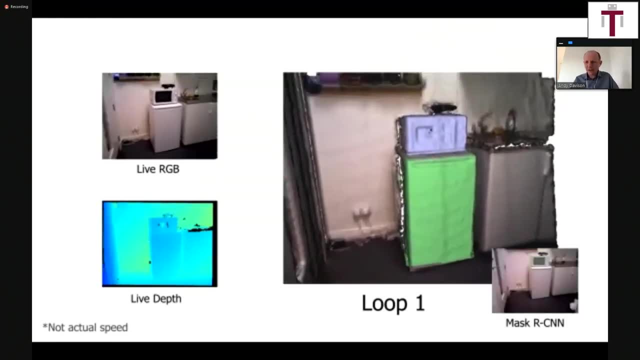 So there we were saying we had a precise CAD model of every object we were going to see. This is kind of the opposite end, where we don't have any prior CAD models, We do have a really good neural network, So we're using MaskRCNN. 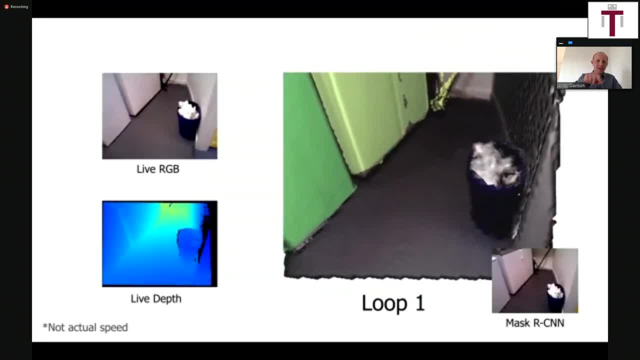 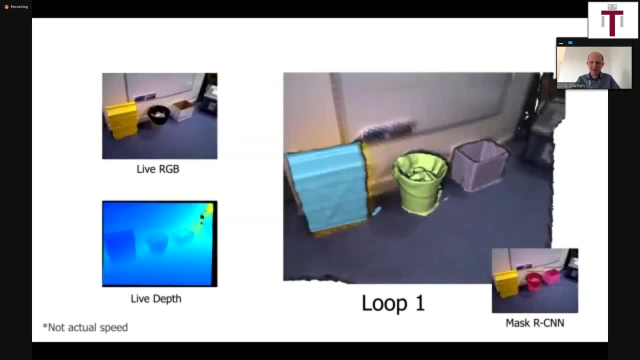 which is able to look at video frames and give us accurate masked regions of anything that it thinks is a separable object. What we do in this system is, for every one of these objects that we detect, we add it to a SLAM graph. 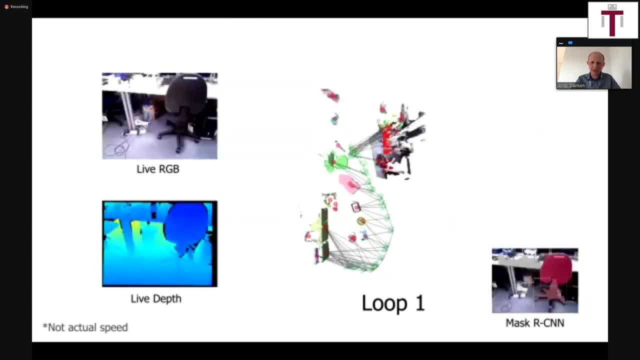 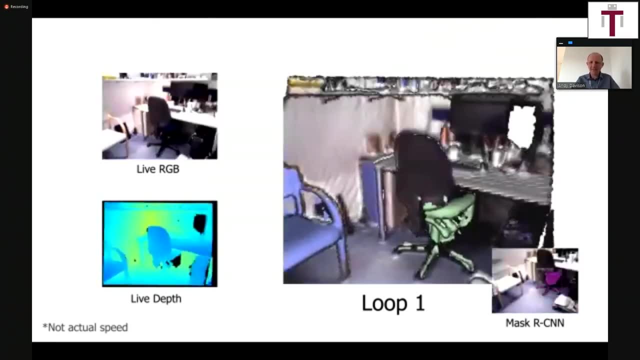 So that's what you can see coming out here now. So this is a graph of the positions the camera has been in and the positions of objects, And then each object we make an independent fused 3D reconstruction of it. So pretty much connect fusion running. 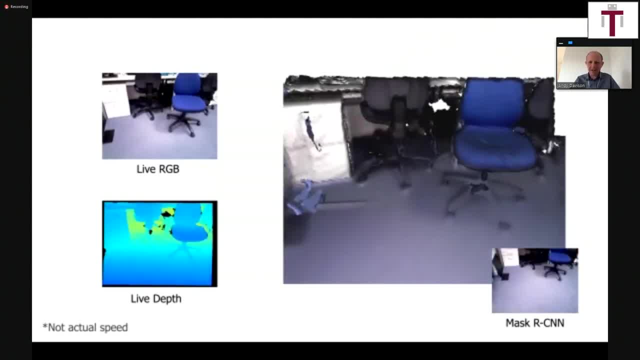 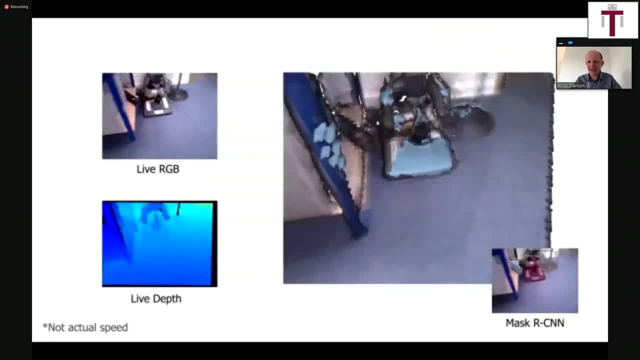 in a little volumetric region for each of the objects And then we've got each of these objects then really serving as a kind of landmark in an overall SLAM graph And we can do normal SLAM things like loop closure. So here we've come all the way around the room. 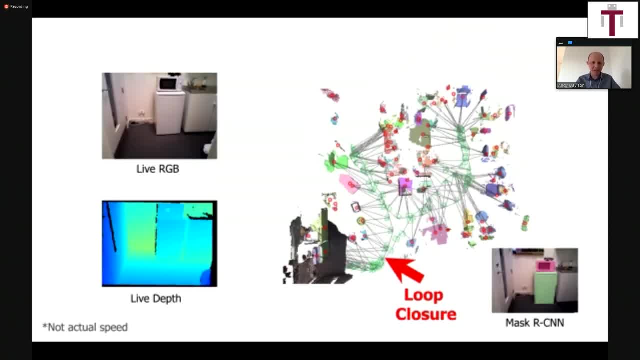 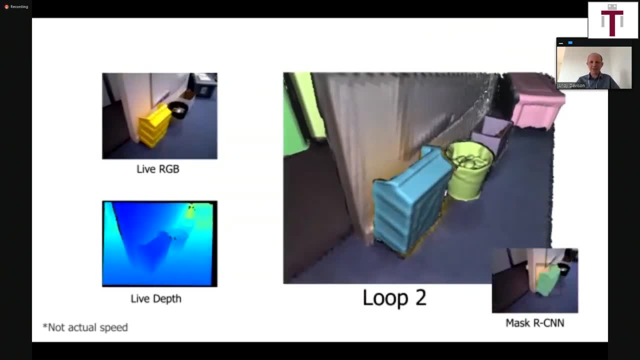 We find a set of objects that are consistent with a set of objects we saw earlier, We enforce those constraints on the graph And solve the loop. So this is a powerful system in that it can map all sorts of different objects in the scene. 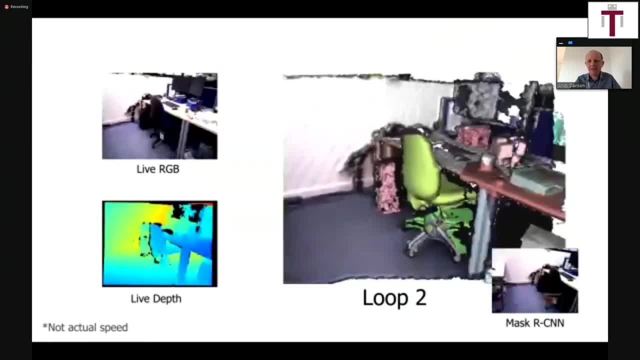 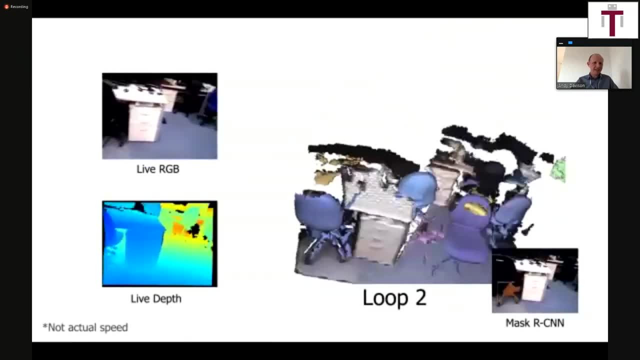 But it has the downside that you know, it's only using the visible information. So when it reconstructs an object like a chair, it's only able to reconstruct the portion of that that it can visibly see. So that's at the other end of the scale of reconstructing. 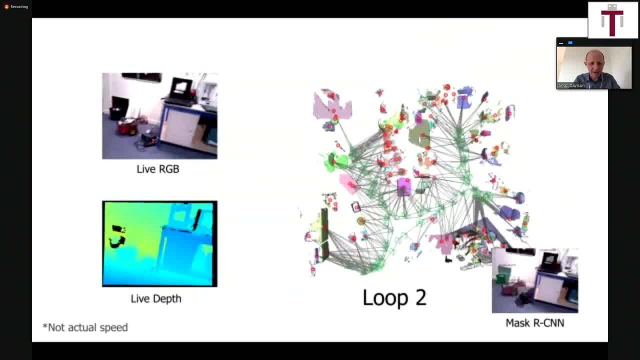 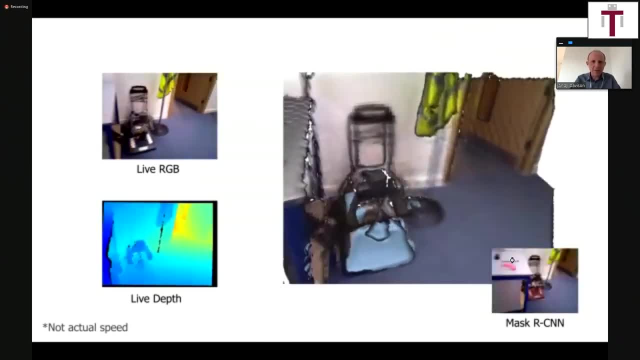 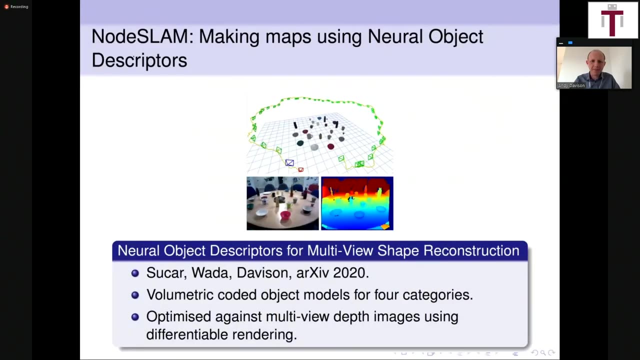 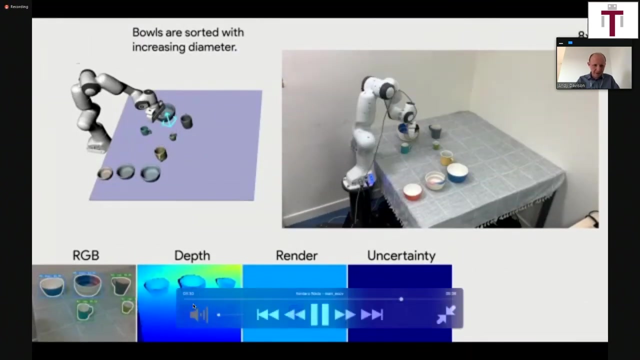 you know, of estimating the pose of a CAD object. So the most recent work we've done in this space is really trying to find us a space somewhere in between. So this system called Nodeslam that we've also just recently put online is- let me just find the right place in the video- 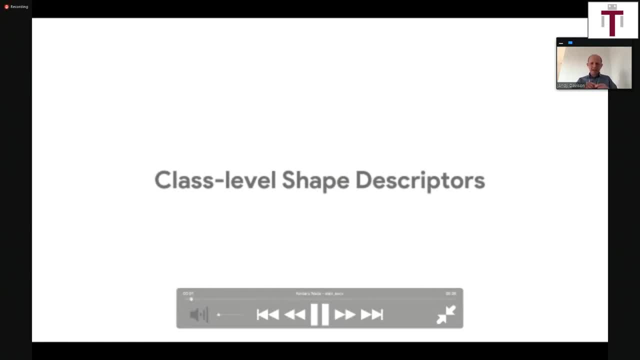 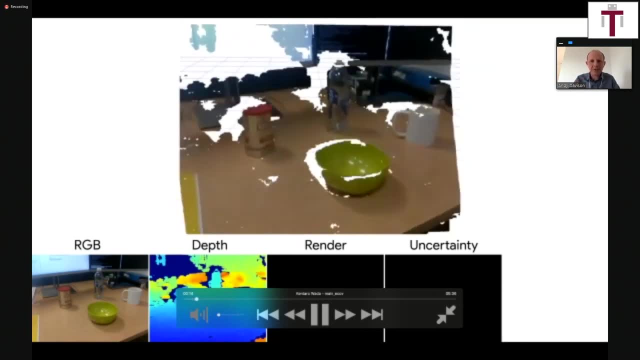 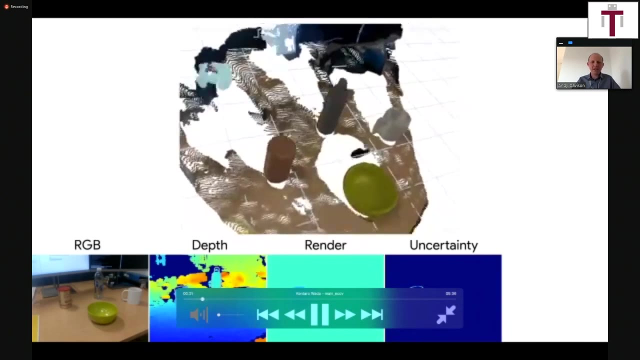 So we're saying that we're somewhere in between. So we're going to recognize objects in the scene, But for a particular class of object we don't have a precise CAD model. Instead, we have a kind of a reference model, kind of warpable shape model. so this is a model that we've, we've, we've learned using a deep 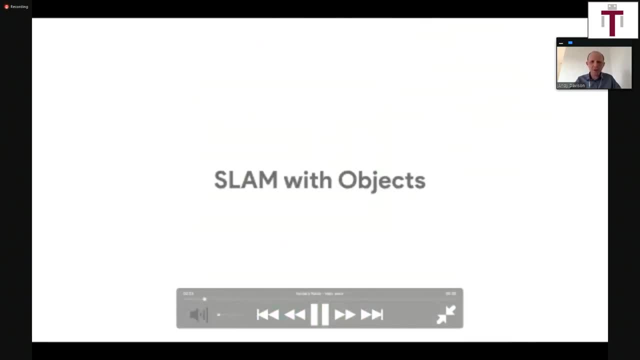 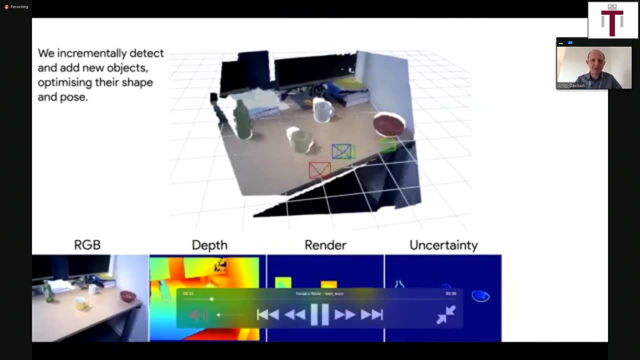 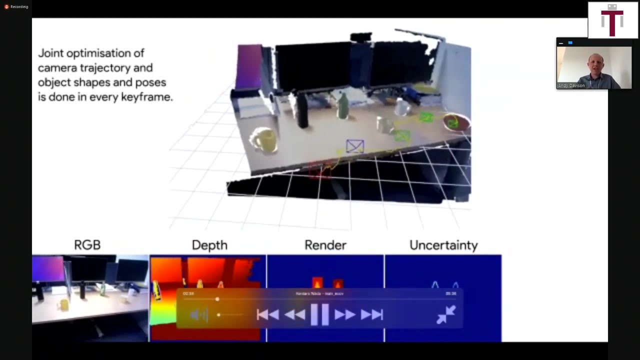 learning method. so it's a 3d volumetric autoencoder which we've trained on a data set of 3d objects. so we've got, you know, hundreds of cad objects of mugs and hundreds of cad objects of bottles and we've learned to kind of shape space model for each one of those objects. so now we can use those. 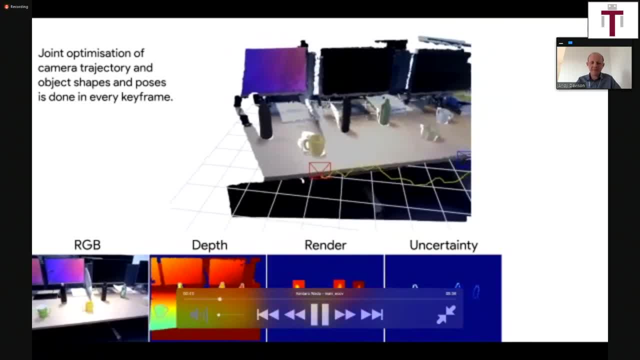 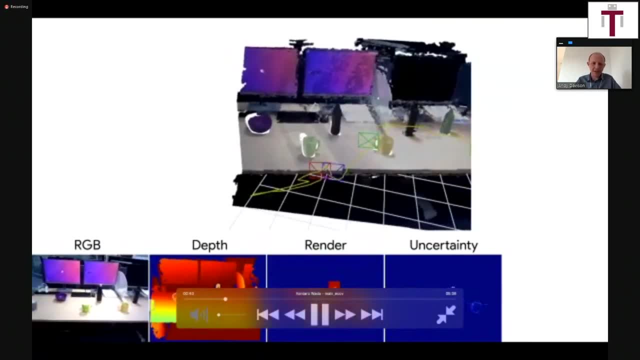 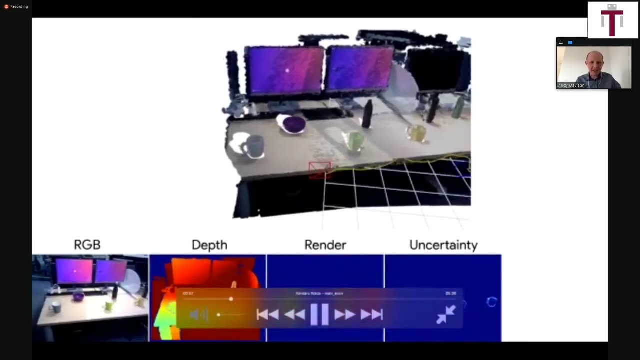 in in a slam context. so so there's lots of uh interesting work on on this kind of idea of coded object models going on, especially in in the computer vision literature. what we focused on here is: can we actually now use these sorts of models for quite useful things in? 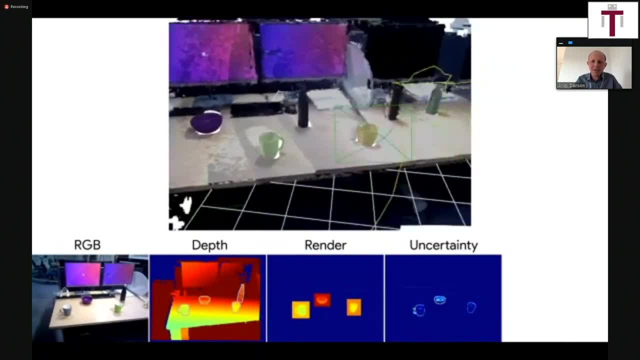 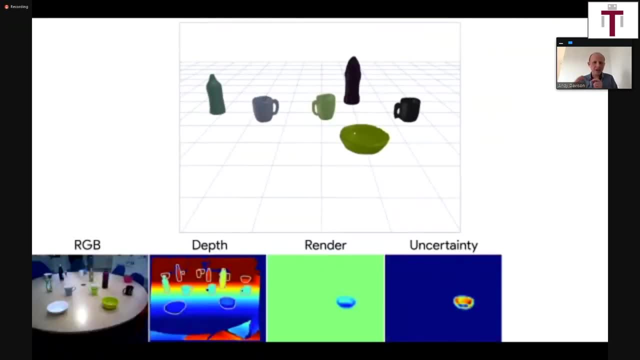 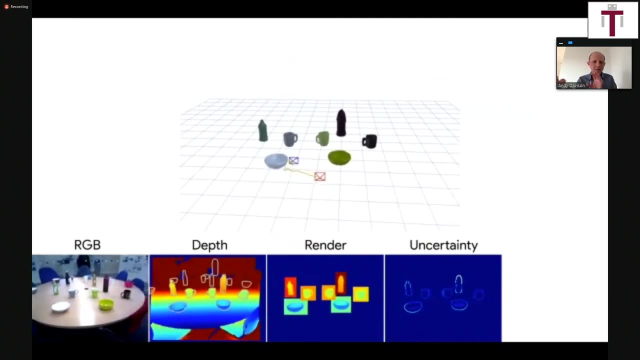 in a slam context. so here you'll see that each of these objects in in the scene the first time that we observed it. we basically optimized over the coded parameters of of the shape model of this, of of that particular class of object, until the, the reprojected shape of that. 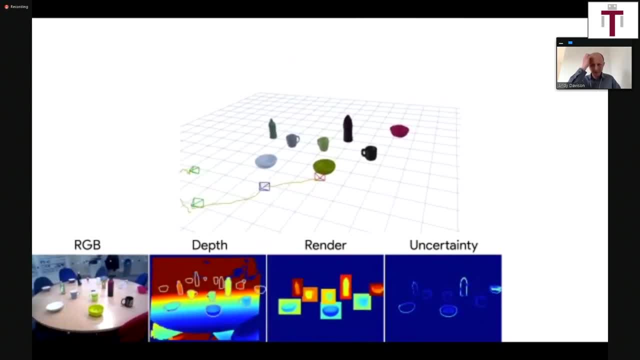 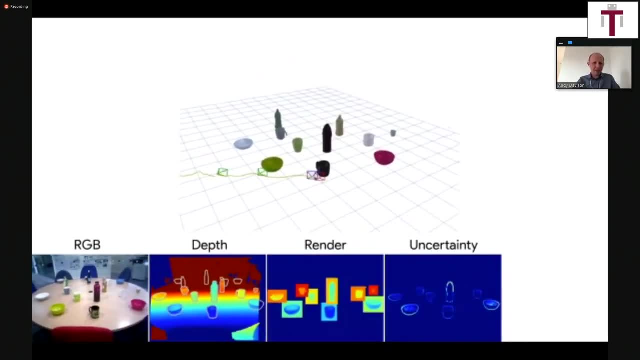 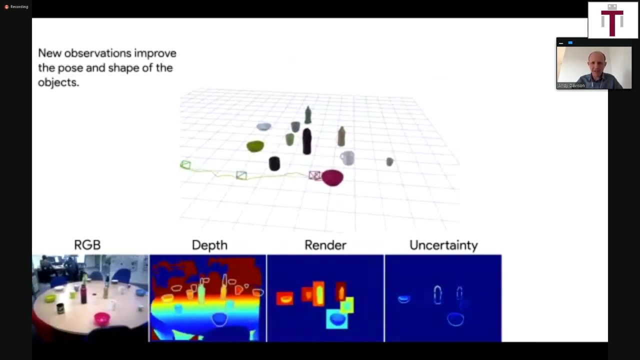 object matched well with the depth information that we've got. so just from one view of one depth view, we can get quite a reasonable estimate of the shape of the object. from multiple views we we can improve that even more. so this is now a full slam system where we are, on each new depth 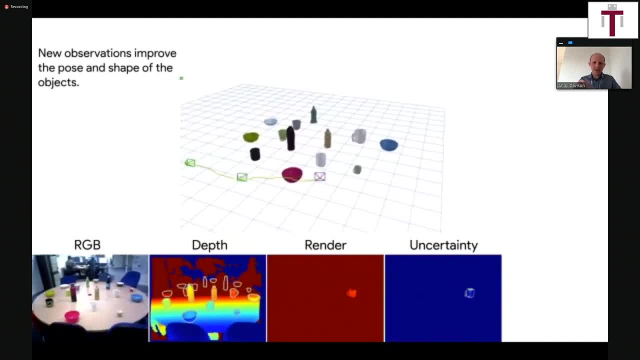 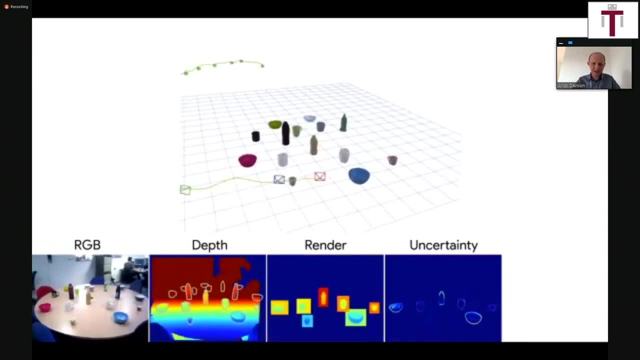 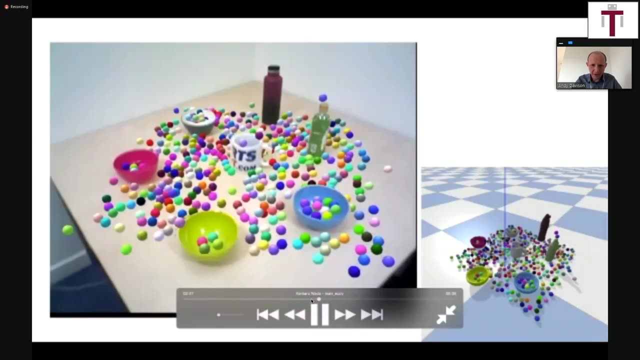 frame where we're jointly optimizing for the position of the camera, the positions of the objects and then also these shape parameters of of the objects, and let me just skip forward a bit to show you an application of that. so we've also um just go to here. so we've also looked at robotic. 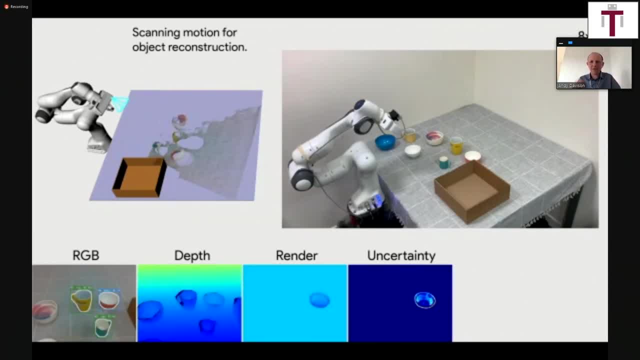 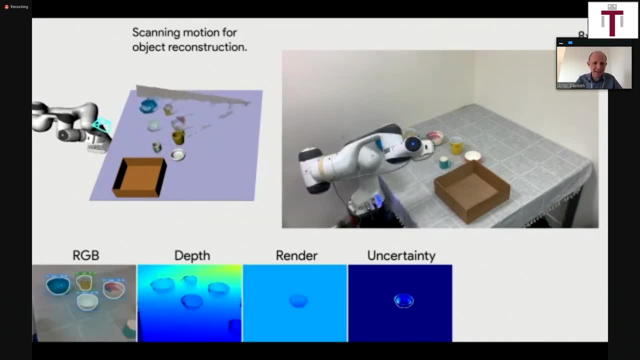 pick and place using using this system. so here we've laid out a few of these objects on the table. we've got a depth camera on our robot arm. the depth camera scans the scene. in the top left you can see it gradually fitting the object models to the scans. once it's fitted the models, it can then do some. uh, you know simple. 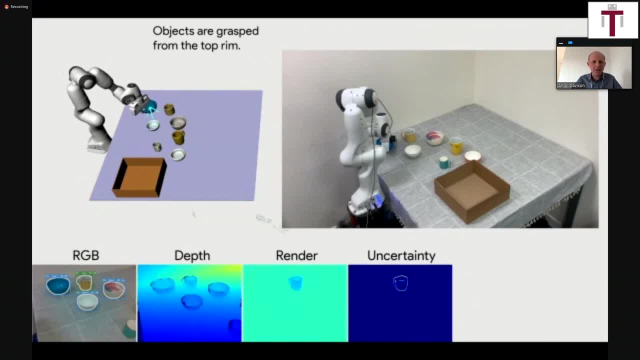 planning and action and here what it does. so it knows that there are four bowls in the scene, but it's able to accurately enough, get an estimate of the size of the bowls, that it picks them up in order of size, biggest to smallest, and then is able to place them in that order to stack them. 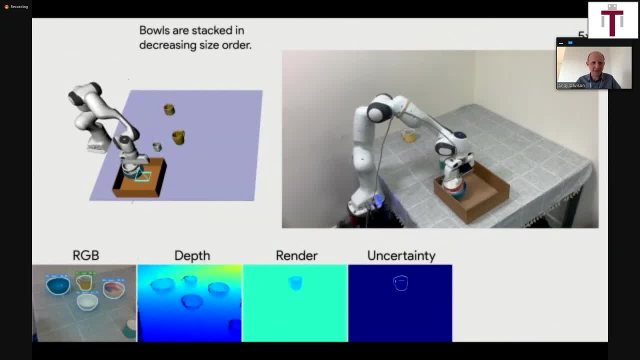 precisely in the box. so again, this is an example not just of picking up an object and dropping it, but picking it up in in a, you know, in in the situation where we've got a very accurate estimate of the shape of that object and therefore we're able to place it very precisely. 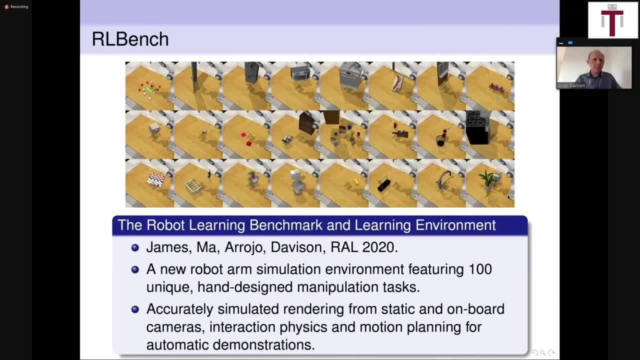 so we're really interested in in this um, you know, object based representations of a scene and and, increasingly, in how those can actually be used for useful robotic things such as, uh, manipulation, uh, the last thing i'll show you in in that kind of area is is work from, uh, the dyson robotics lab called the rl bench, so this is a new um. 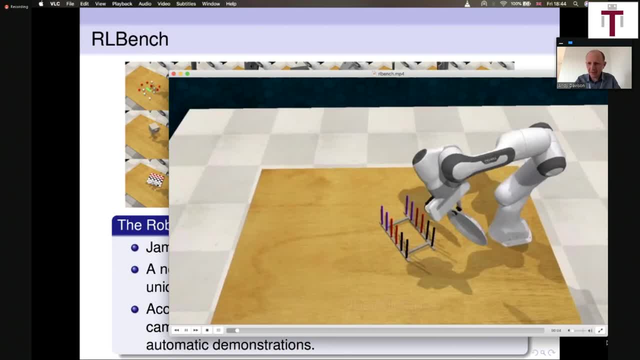 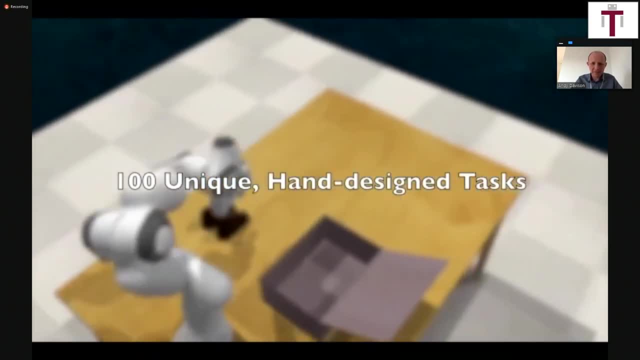 benchmark um simulator or data set, which we've- uh, just recently put online. so this is. this is also available as as open source software. so we're interested in enabling robots to do many different things over the years. so, moreför all, we're planning on have amazing Ble如. 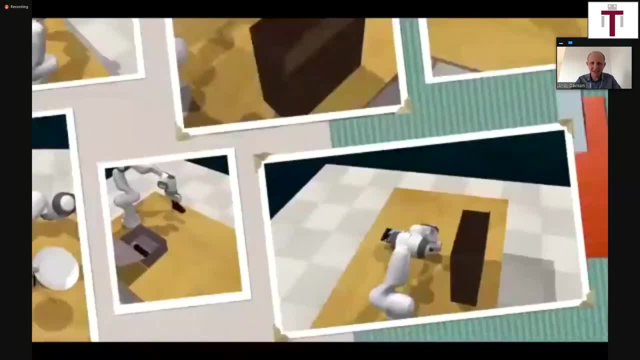 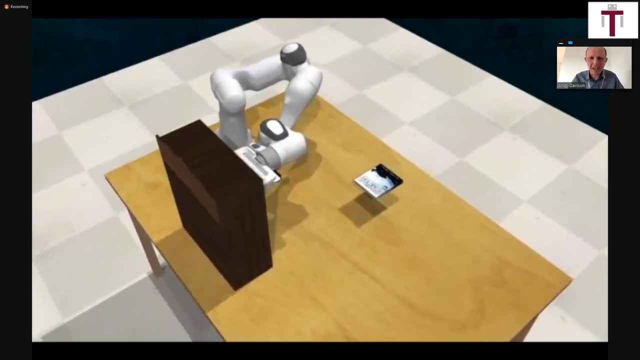 make a few developments in our duas. so this is is a data set where the these are hand designed tasks for many of the things we might imagine a robot arm might want to do, like placing, placing objects, you know, opening things, closing things, putting things on top of each other. 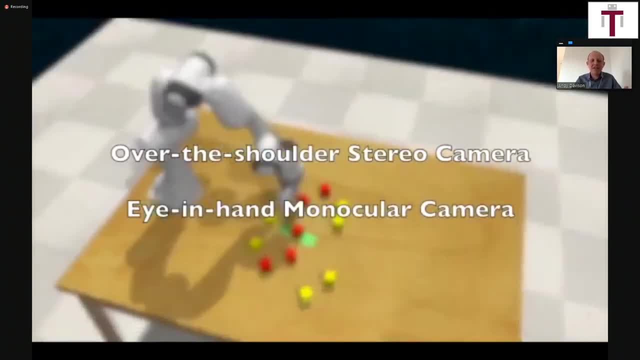 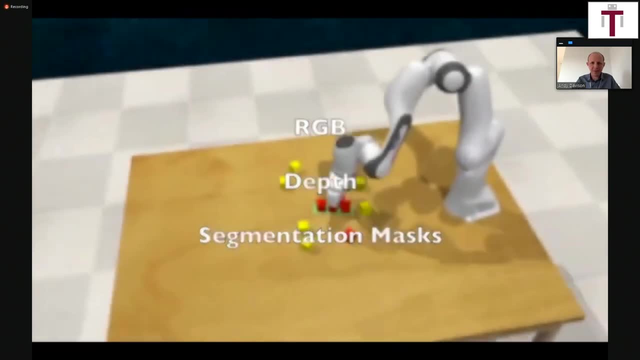 um and wi. within this simulator, you can really do what you want. so so you can run, run the simulator. it includes simulated cameras of various kinds, both kind of off-boarding and on board uh. it includes simulated cameras and various. at each point in the process we've done experiences of off-boarding and on-board uh making IoT objects. that can use all of the elements that we've delivered on- avait have initially developed this about both см. use them and make aMicro with the sdU poderia, so on the site of the robot, an arm. so this is a we've got atthow which we're. 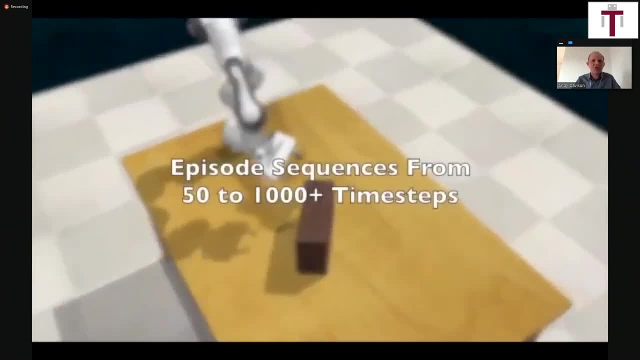 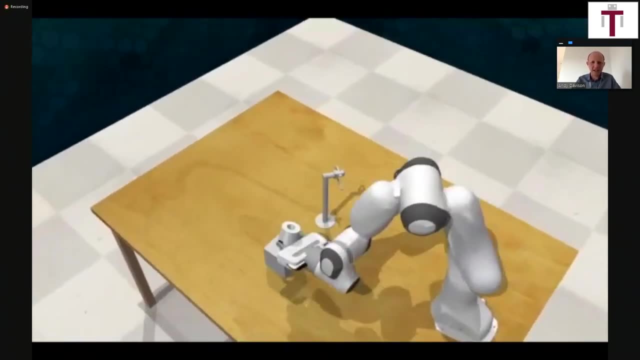 simulation of physics. So, for instance, you could train reinforcement learning agents to try and solve these tasks, And some people are trying to do that. But what we really wanted to do with this data set was make it deliberately pretty much out there in terms of what anyone's doing in. 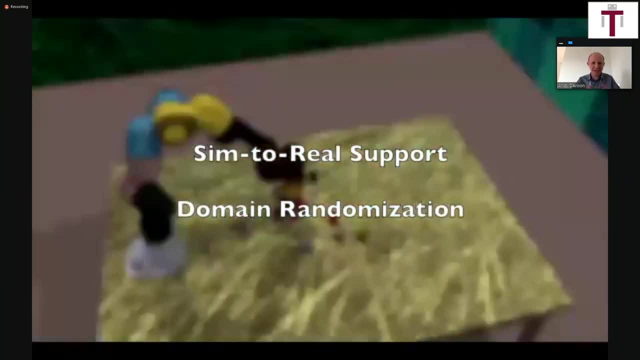 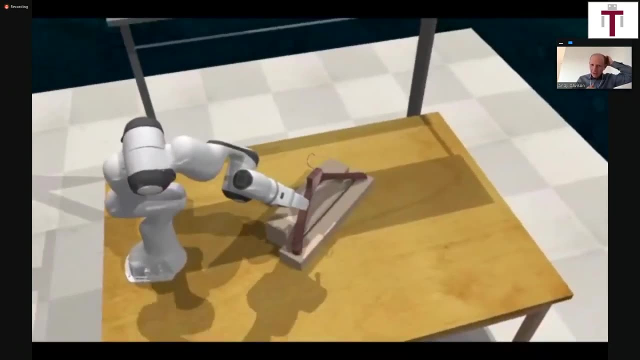 reinforcement learning. This is an example, by the way, of domain randomization, So that's something that's been found to be very useful in a lot of reinforcement learning. So you know, no one has shown reinforcement learning able to do these wide range of things, And you know reinforcement. 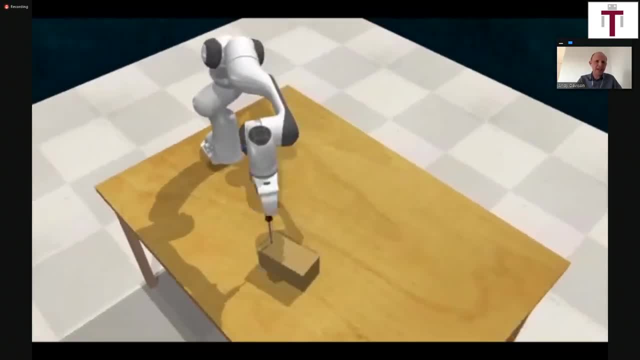 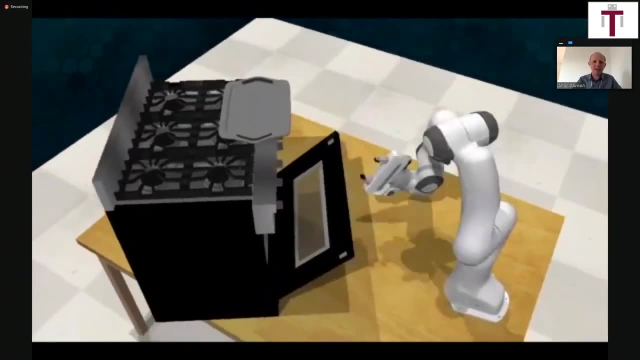 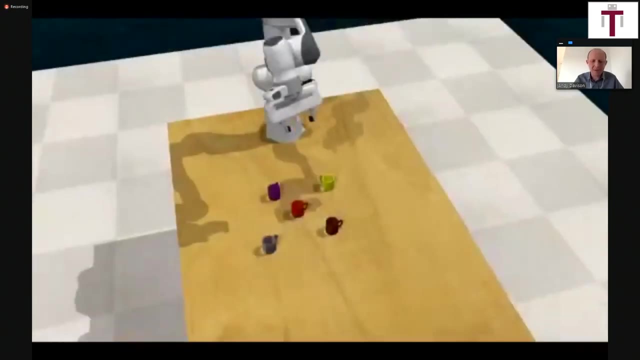 learning, I think has mainly been successful for fairly sort of local and repetitive kind of tasks. So I would argue that maybe something more like a spatial AI, SLAM-like object-based representation of a scene may be the sort of thing that may enable AI to solve tasks like this. 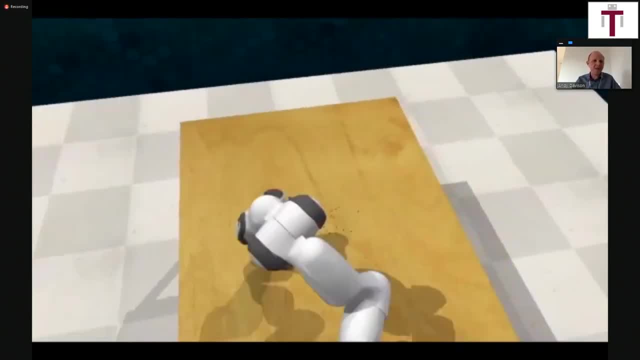 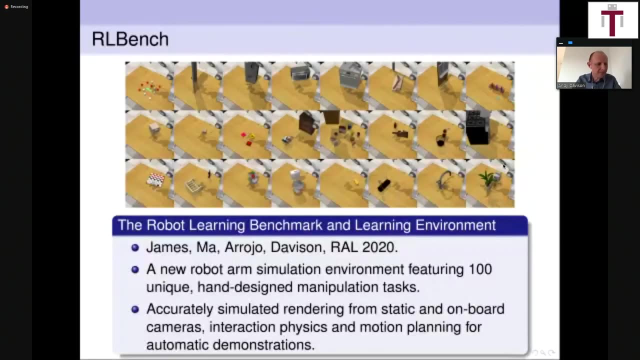 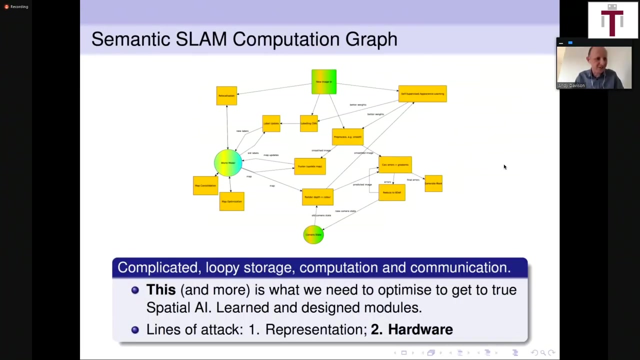 So by putting this data set out there, maybe we can motivate more people to be interested in those kind of those kind of methods. Okay, so I mentioned earlier on that, given this rather complicated looking computation graph, we needed angles of attack in order to really make this computation feasible. 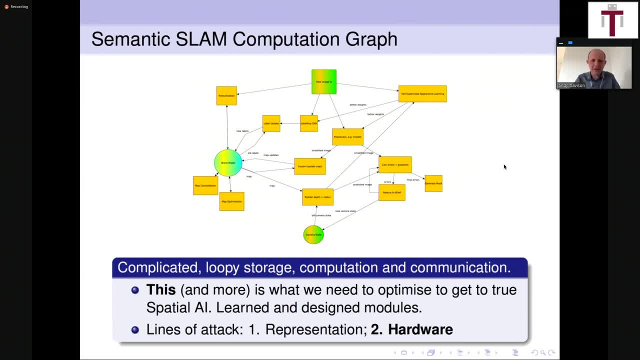 especially on embedded devices, And the first thing that we really looked at was different sorts of representation that might turn some of these things into things from you know, huge blocks of data into rather smaller things like codes, for instance, representing objects or scenes. The other kind of key approach I've been very interested in: 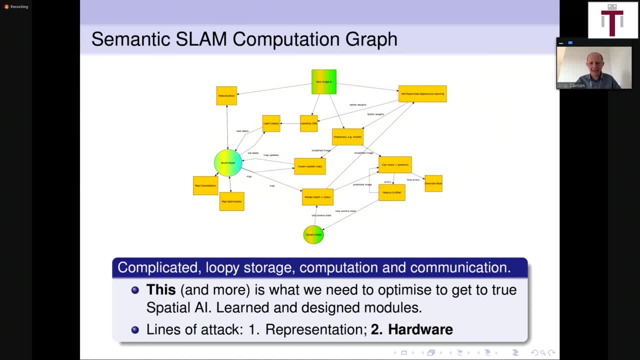 is the last few years is: can we use new things happening in hardware to help us with that? So hardware as it relates to SLAM and spatial AI, So I'm not really talking here about actual robotic manipulator hardware, about the sensing and perception hardware and, in particular, the computation hardware that would be. 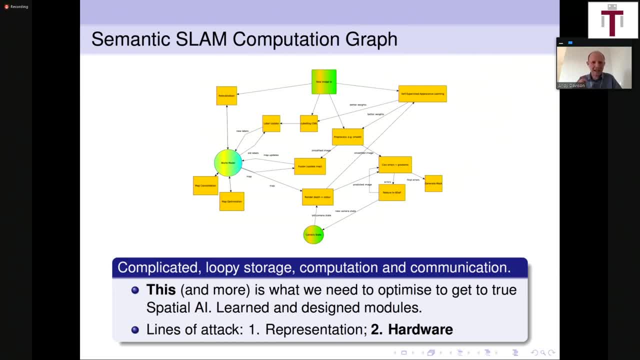 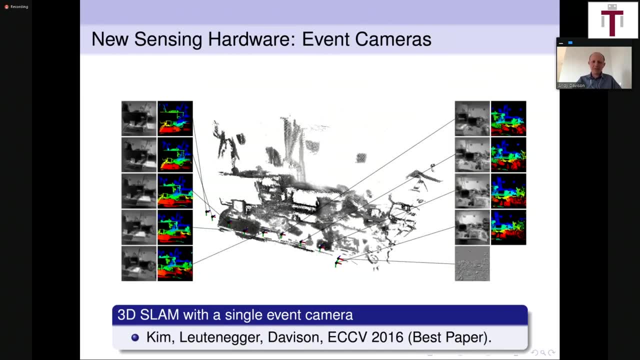 involved. so the main areas of interest are sensors and and computer processors. so first of all in in sensors. that uh, so i've been very interested in, in what's been going on in in cameras. so, as alberto mentioned earlier, you know i see computer vision as a, as a broad area and i would have 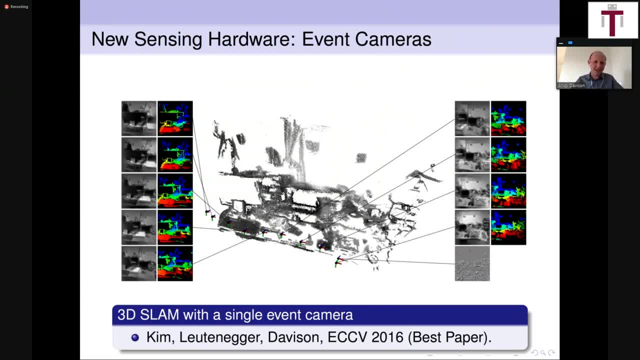 always included. you know, whether it's a single camera, a stereo rig, a depth camera, it's all part of computer vision, but that isn't isn't an area subject to ongoing change, and the most exciting thing that i've seen in the last few years is is event cameras, so this is probably something. 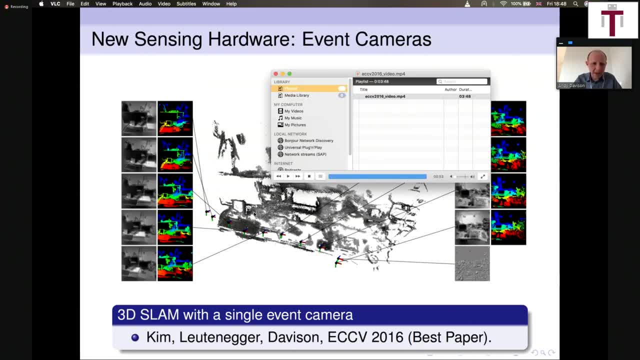 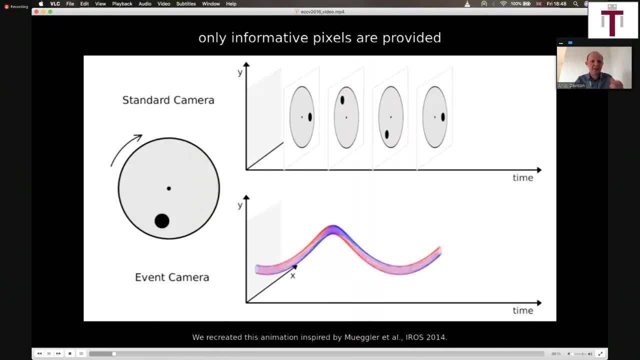 that a lot of you, uh uh, know about. so this, this is um, an image sensor that, rather than capturing frames, it captures per pixel. uh, asynchronous differences. so so the report from a from a depth, from an event camera is, is a is a sequence of events which is each pixel telling. 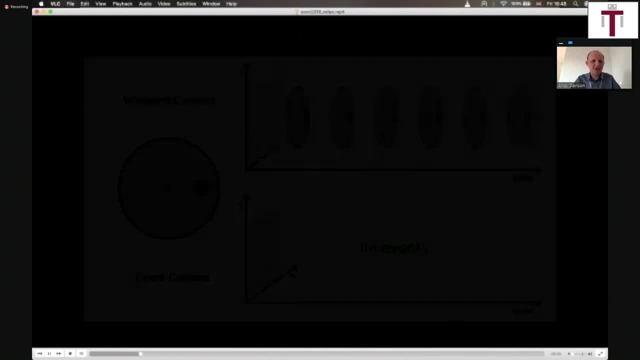 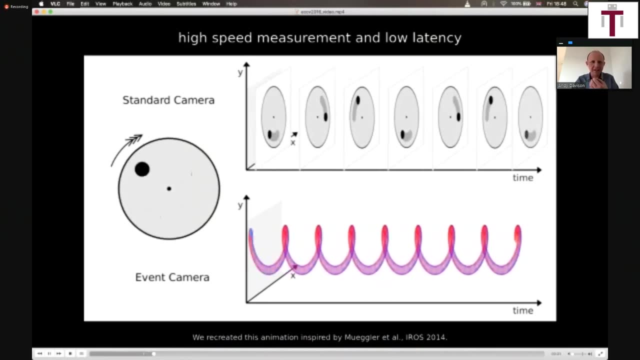 you with an accurate time stamp when it's changing its its brightness. so as soon as i heard about this, i was immediately excited, you know, first of all because you know the data rate from a camera like this is much more scene dependent. so if there's nothing changing in the scene, then there's 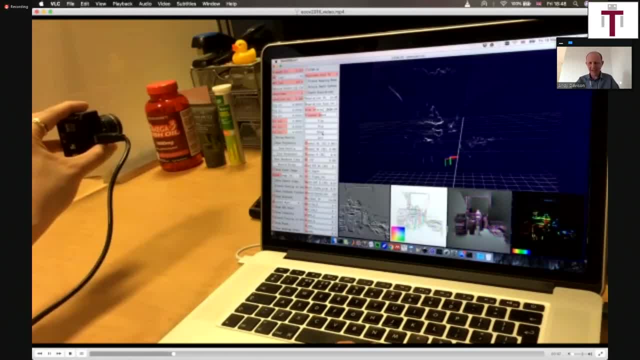 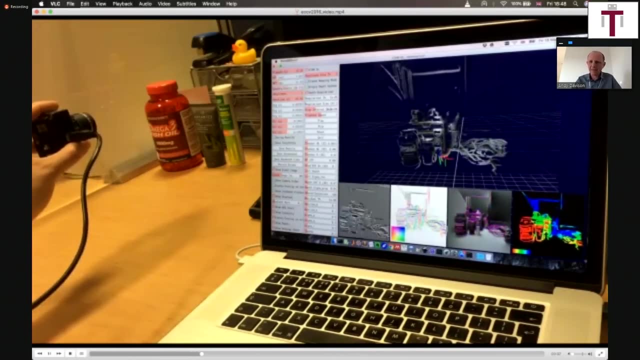 no events and if there's a lot changing in the scene, there's a lot of events. um, so we worked on slam, like competencies, using these, these cameras, and i'm not going to detail on on this, but we, you know, we, we managed to it to achieve uh, you know, monocular uh 3d slam with, with a single event camera. so here there's. 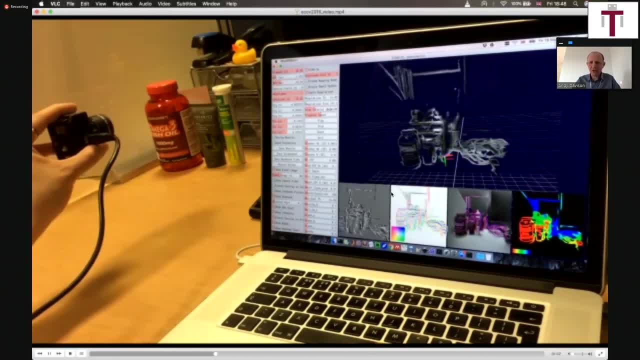 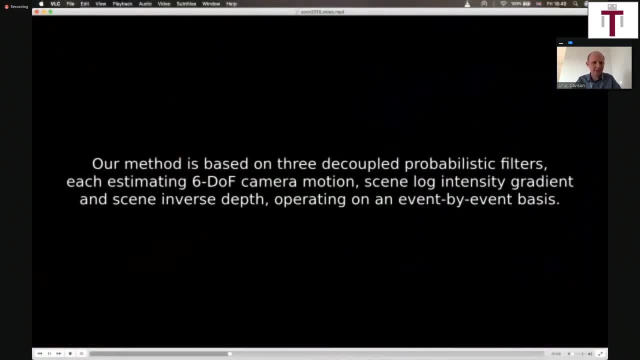 just a single event camera being being waved around and we're jointly estimating um the color. so it's the intensity reconstruction of the scene, which is not something that comes by default from an event camera, the 3d motion of the device, uh, and and the depth of the camera and the depth of the 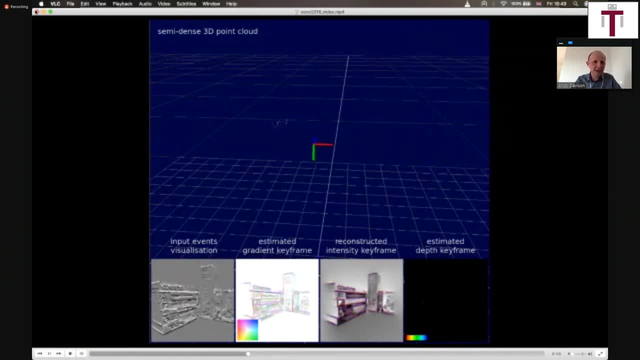 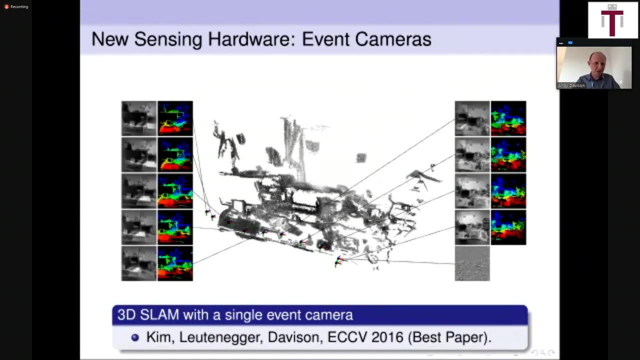 depth of the scene and that, so that work is is is very much ongoing. there's lots of- uh, several labs now doing really, really nice work in in in this area, but for me it's it's all about this: um, you know, i i think about this in terms of a computation graph and this idea that this event camera does. 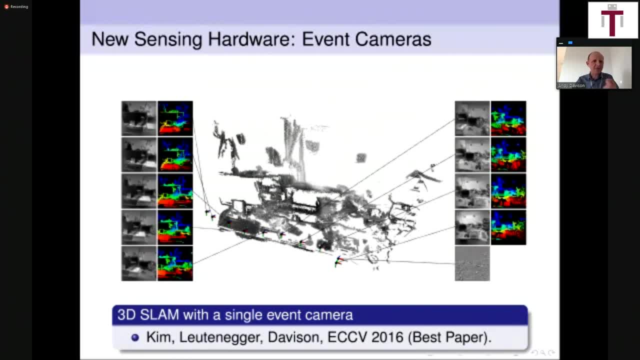 write in hardware, on, on basically the sensor chip. it does a very important job for you so you don't need to pipe video data down to a cpu because it's done some abstraction right there on the chip, and i think that's the start of a more general thing that's going to. 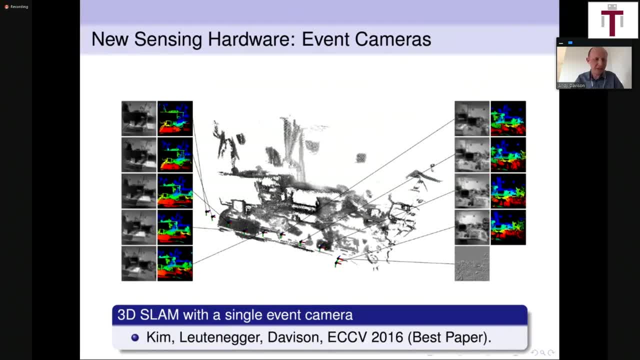 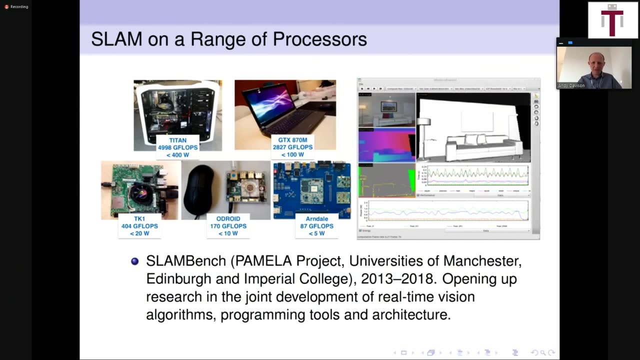 happen where cameras will become programmable devices that are able to do a lot of processing right right there, kind of within the chip. um, so the other big area in hardware is processors, and this is something i've also been really interested in and really starting from, you know, going back, 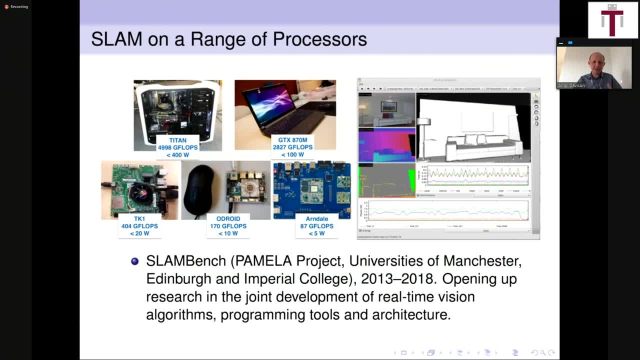 10 years where i saw gpus coming into computer vision and what a massive difference that made. i mean, i think everyone's really interested in that and i think it's an interesting topic, but i think part of it is with gpus and how it ��s a little bit more complicated than that and i think we did a brilliant job working on 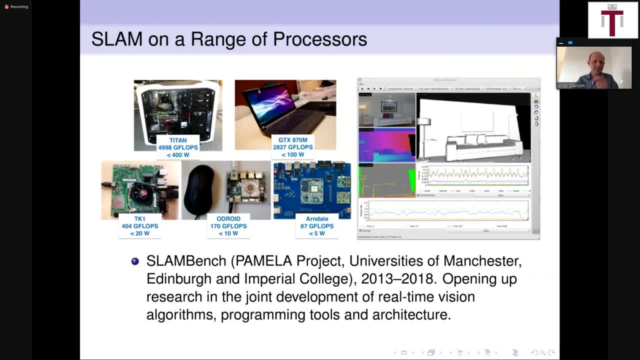 this and we have this idea called a traditional global computer, charles earth Plaza card, if anyone is familiar with that now with with deep learning, that you need gpus to do deep learning but you also need gpus to do to do dense slam, so the sort of computation where you want to do something at 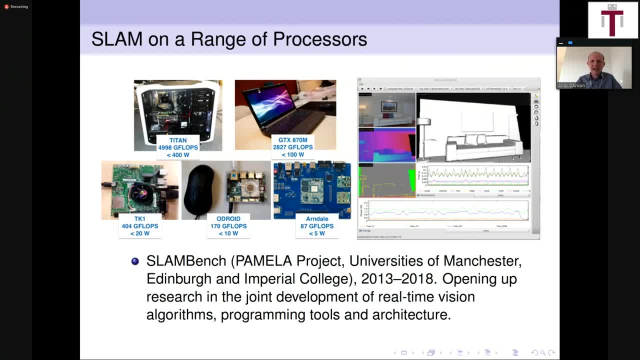 every pixel on every frame and it's very parallelizable. gpus are really good for that. so we different sorts of processors. So from a huge sort of desktop machine in the top left there with a big GPU, down to a tiny embedded board. So can you pick apart a SLAM algorithm? 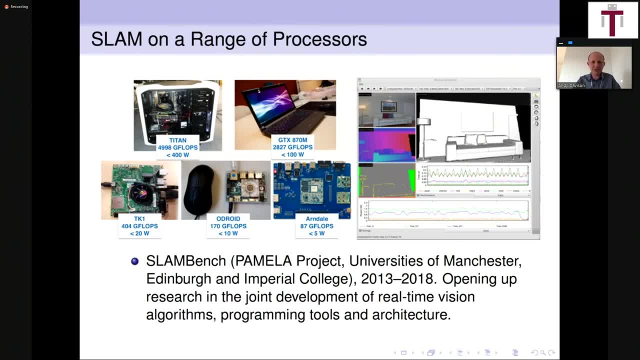 Can you really think about which bits work well on which sorts of processor And can you facilitate the sort of research on co-design of processes and algorithms? And of course, an obvious question there is: can we build a chip specifically for SLAM that's as efficient as possible? 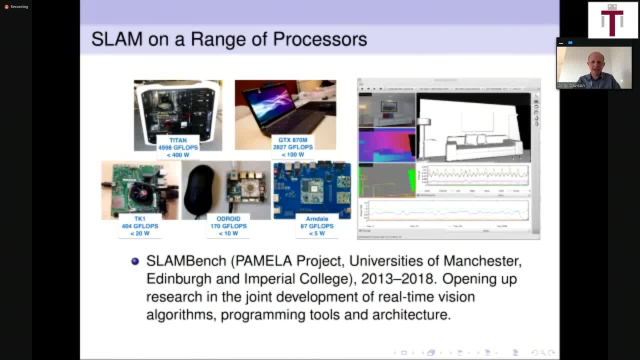 And that's a really good question And there's been lots of nice work and some concrete projects on that particular idea. My kind of current thought about that is my thinking about SLAM is too broad at the moment to do that And I think when I was taking part in this project- 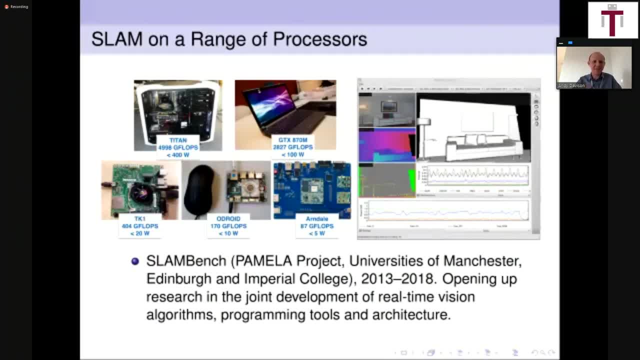 people wanted to pin me down and say, OK, what's the algorithm, And then we'll go and design the hardware. But I was always a bit like, well, there's a lot of possibilities And I'm not sure, So I wasn't really willing to commit at that point. 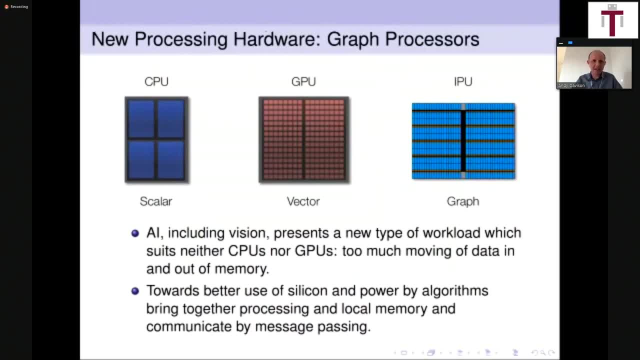 But then I heard about interesting things that were going on in kind of commercial hardware and, in particular, graph processors. So the main workhorses of AI at the moment are CPUs and GPUs. Of course, these are processors that are very useful. 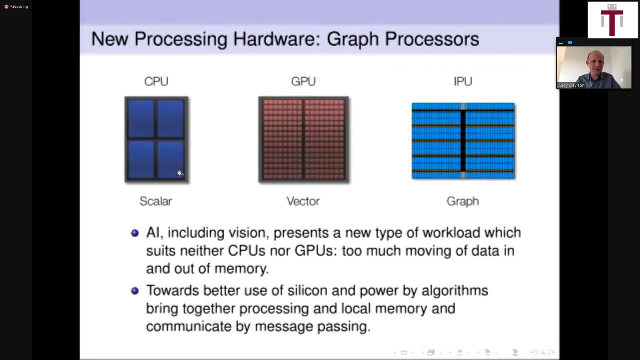 but they're not really designed for AI or vision. CPUs are designed for general purpose compute where processors. So, if you like, GPUs- are designed for graphics. They've been successfully adapted for various things in vision But, as I pointed out earlier, we can. 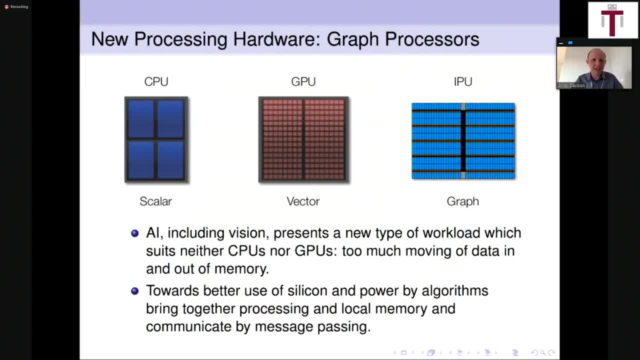 use them for parts of a vision system, but very far from all of it. We generally have to have CPUs still around too, So a graph processor is a new idea, And in particular, there are many related ideas here, But I'm going to focus on a company in the UK. 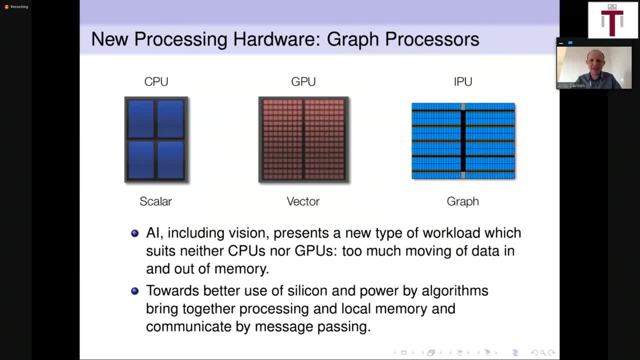 called Graphcore, that's got a product called the IPU And it's a new chip. And it's a new chip that's been developed in the UK called the IPU or intelligence processing unit, which is a new processing chip which is designed. 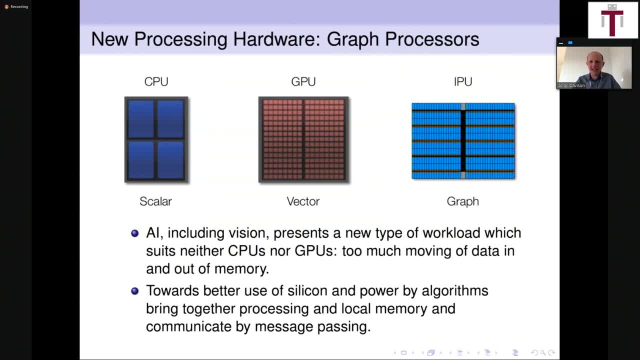 to particularly enable what they think are the important workloads in AI. So what a graph processor is? it is a massively parallel chip. So an IPU has about 1,200 processing cores on it, But they're quite different from the cores on the GPU. 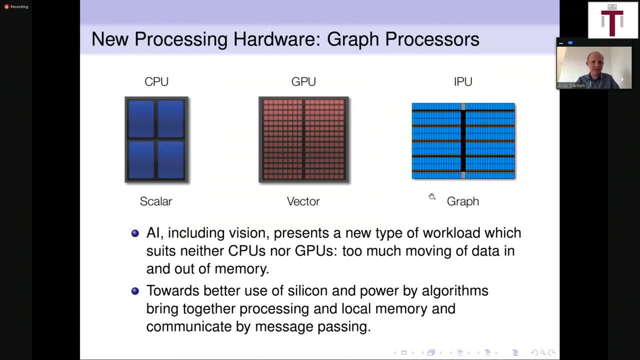 They don't all have to be doing the same thing in lockstep parallel, And they're able to have very high bandwidth and almost arbitrary connectivity for message passing between them. So what they're really good at is processing graph-like workloads, so, ad hoc. 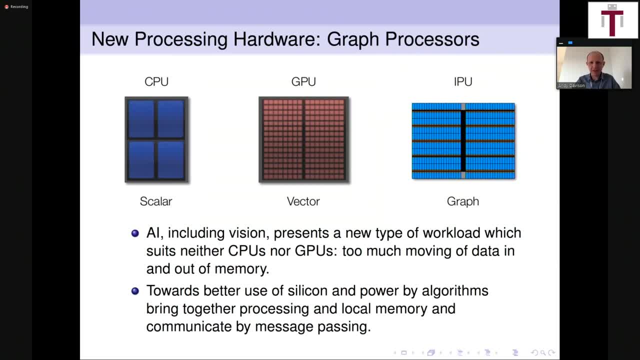 kind of arbitrarily shaped graph-like workloads And really the sort of processing where the computation and the storage is really kind of mixed together. So for an IPU to work well, you don't want it to be pulling any data from external memory. 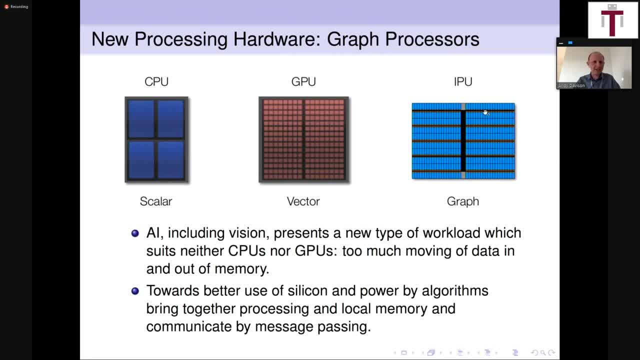 You want anything that it's interested in storing to be stored in a distributed way, kind of alongside all of the cores of this processor, and then to talk to each other by passing messages. So that's very interesting. I can immediately see this can reduce the sort of data flow. 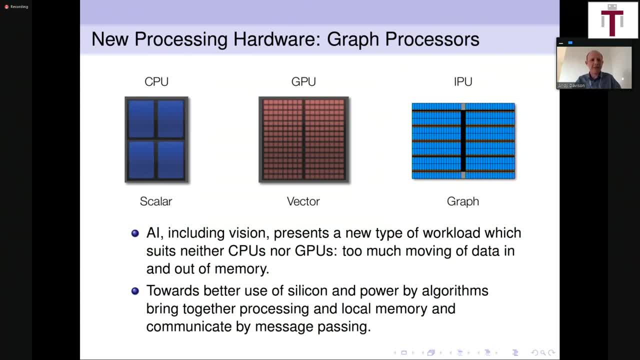 So the things that make processors use a lot of power are generally moving memory around bits times millimeters. is what you want to reduce A graph processor by really thinking about joining jointly, reasoning about processing and storage can really tackle that And yeah, there's a lot of technical detail. 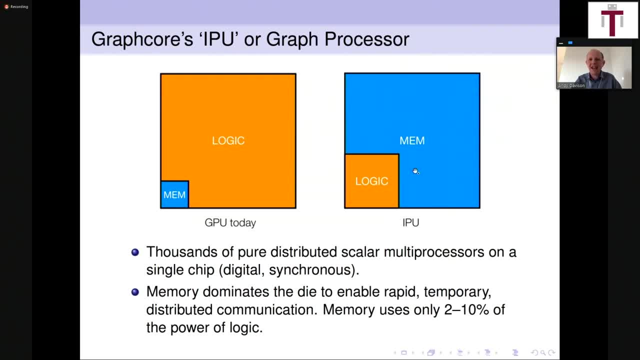 but an IPU devotes a lot more of its area on the chip to memory, which is all about communication and local storage, than logic, which is about fast compute. So the actual cores on an IPU are not individually that fast, but they're very, very well interconnected. 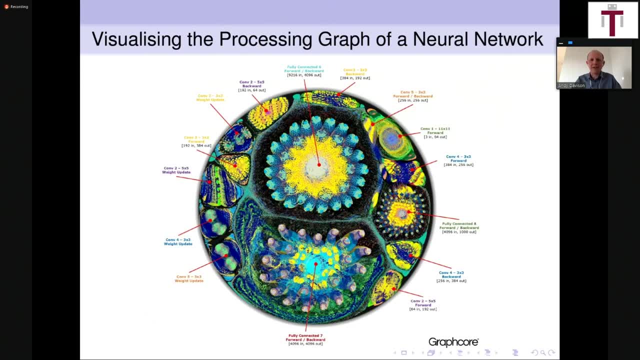 So that enables new styles of algorithms. So when you compile something for an IPU- and this is a visualization from Graphcore- you have a computation, and they're particularly focused on optimizing neural networks. So this is, I think, AlexNet actually. 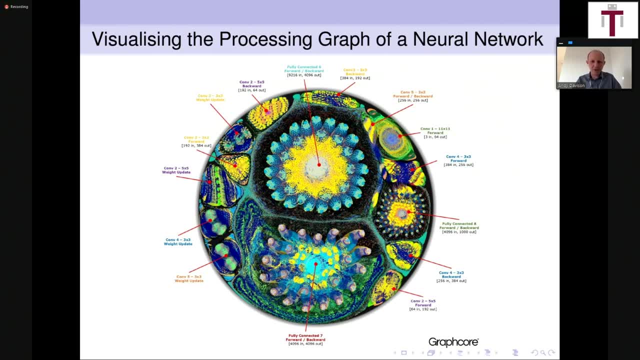 You take all the computation involved in training or using AlexNet and you think of all the elementary sort of computations and data movements that have to happen and you compile it down onto the grid of processors on an IPU And this is a kind of cute visualization. 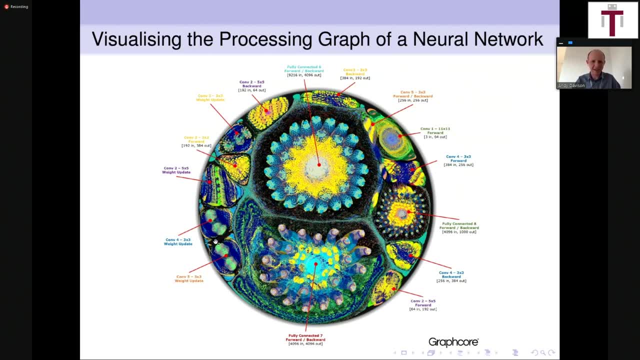 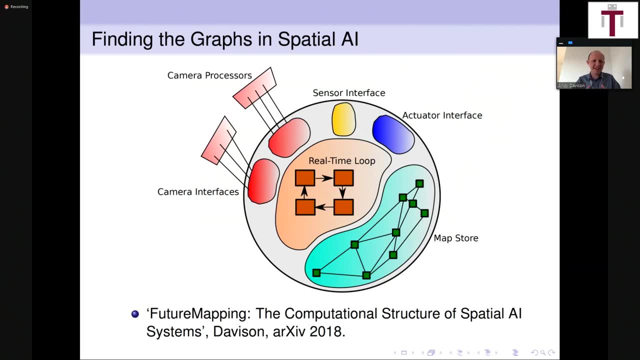 that shows something about all the connectivity and you can identify the kind of regions in the neural network. So having seen that, I started to think: well, could we do spatial AI in a similar way? So this is really preliminary thinking and there's a lot more detail in this paper I mentioned earlier. 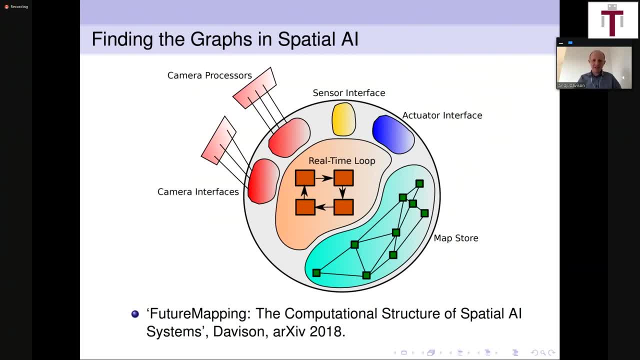 if you're interested. But let's think about all the computation involved in a spatial AI system. We've got a real-time loop doing things like tracking and labeling. There's clearly a graph-like structure there. We've got cameras which are kind of sending data. 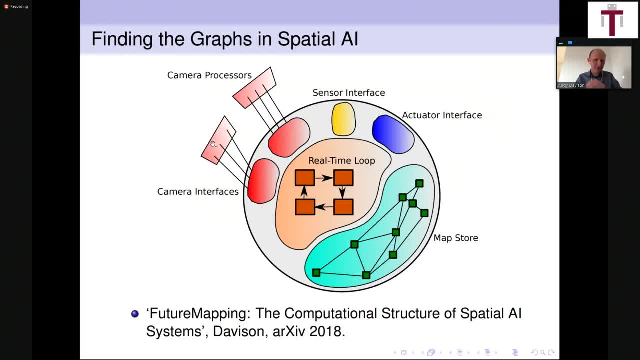 There's clearly sort of graph-like structure there in the regular pattern of pixels and so on. And then we've got our kind of map store, and anyone who's worked in SLAM for a while knows that graphs of how different nodes and factors connect to each other. 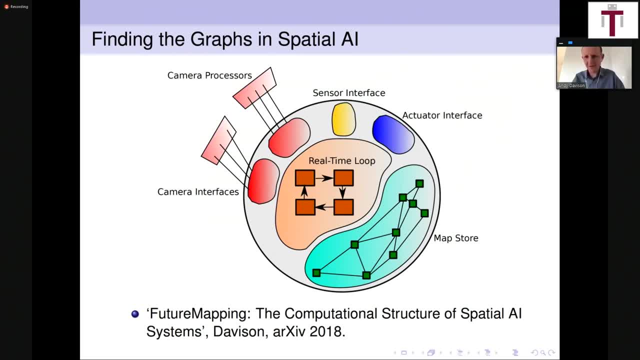 are really the best representation for For SLAM. So there's graphs everywhere in SLAM, So can we really map those graphs onto a processing chip and then use that to implement, possibly, some steps towards this very efficient vision of spatial AI that we think we need for products? 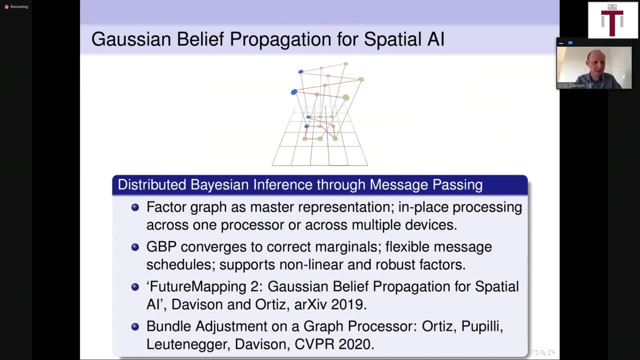 So we've taken some first kind of concrete steps in that in the last few months and we've got a paper to appear at CVPR which is called, which is called Bundle Adjustment on a Graph Processor, And there's also another long discussion paper. 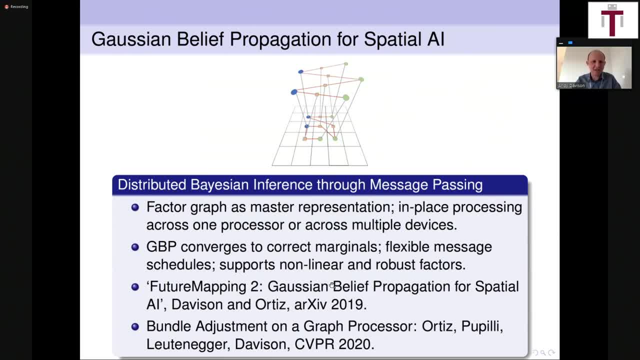 about the general idea of a class of algorithms which I think is really suitable for this, which is belief propagation. So certainly not anything I've invented, but something which I think might very much come back into interest because hardware has changed So we've been able to show concretely in this paper. 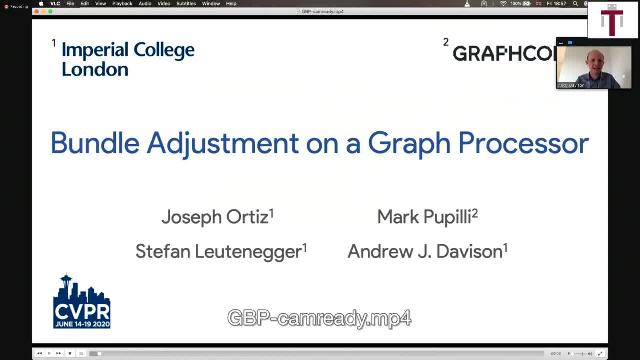 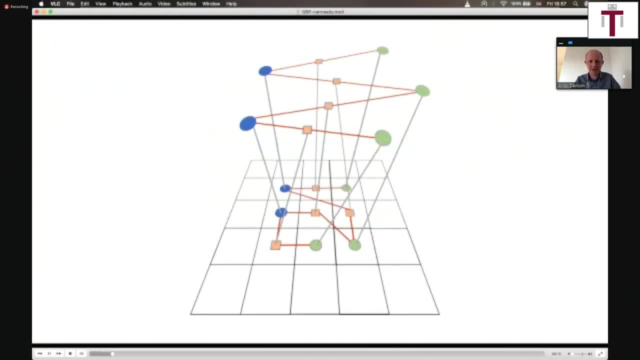 we'll show at CVPR that we can implement a classical computer vision algorithm, which is essentially the core SLAM problem of how do we jointly estimate the positions of a set of cameras and a set of points on an IPU chip, by using Gaussian belief propagation. 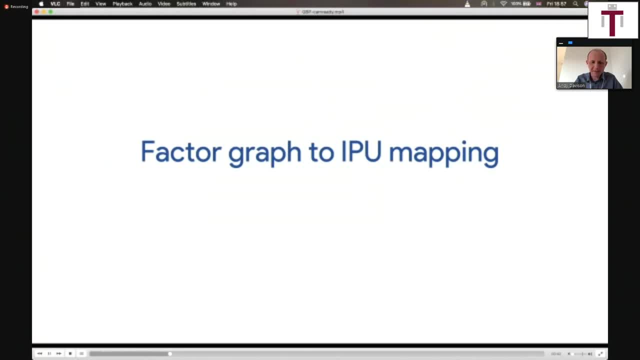 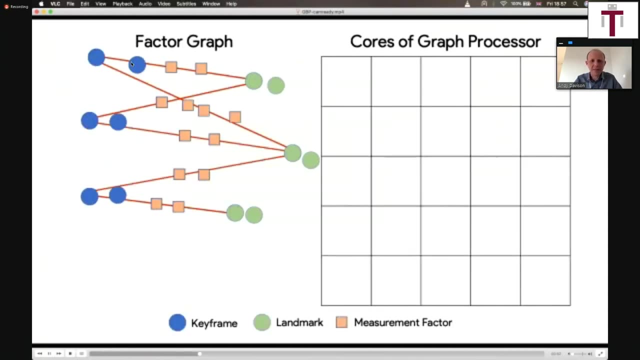 So if I just skip to the right part of this, If you're familiar with factor graphs, so on the sorry. on the left, here we see the factor graph for a bundle adjustment problem and we map each of those nodes, variable nodes or factor nodes. 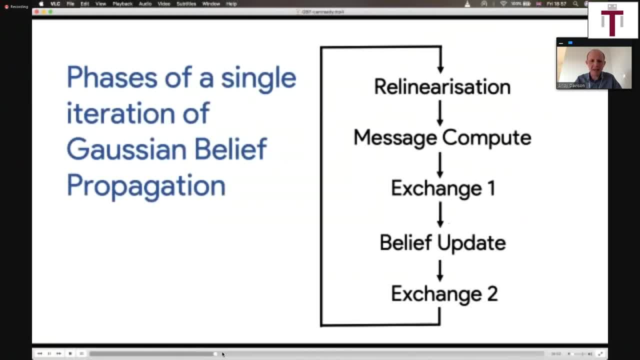 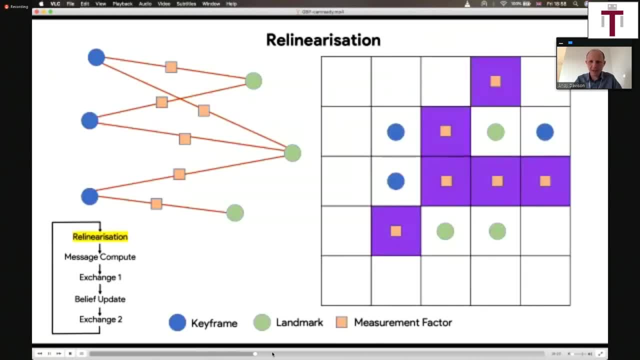 onto tiles of our IPU And then we were able to perform the optimization that we need to do in bundle adjustment by message passing. So we're going to send messages around between these tiles in some pattern and show that we can achieve optimization of globally consistent things by purely local computation. 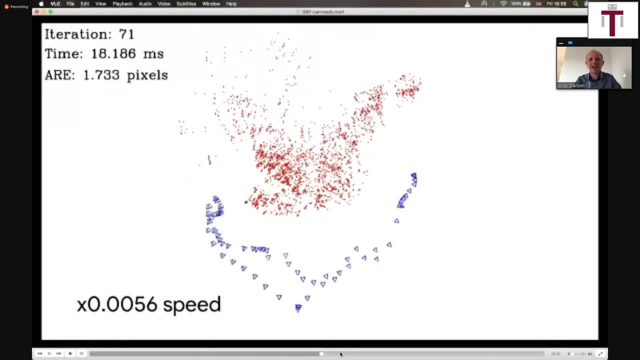 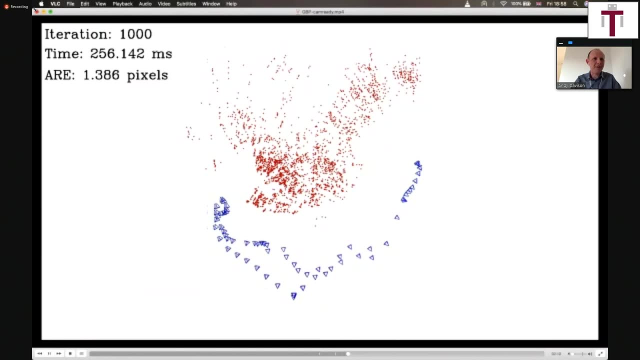 and message passing and show that we're able to do that very fast and very efficiently. And in some very preliminary results that are in this paper we show we can optimize a reasonable size bundle adjustment problem 20 times faster on an IPU than you can on a CPU using Ceres, the standard CPU. 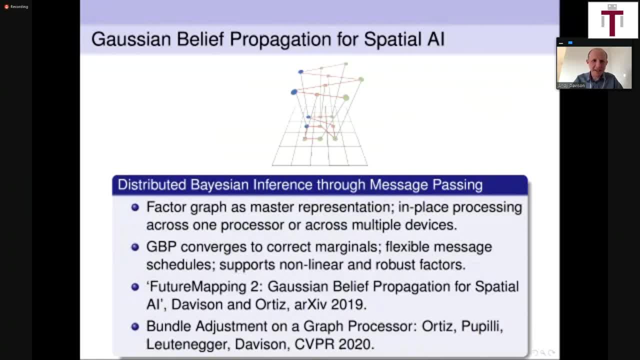 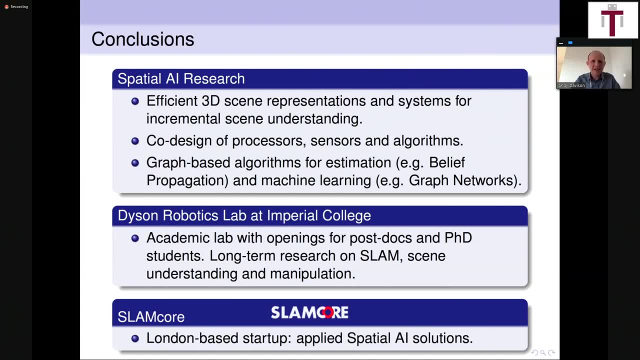 algorithm for that. OK, So I think I'm pretty much out of time, So let me just finish with this. I think we've come to some conclusions. So spatial AI research: I think it's a fantastic thing to work on and I think we'll be working on it. 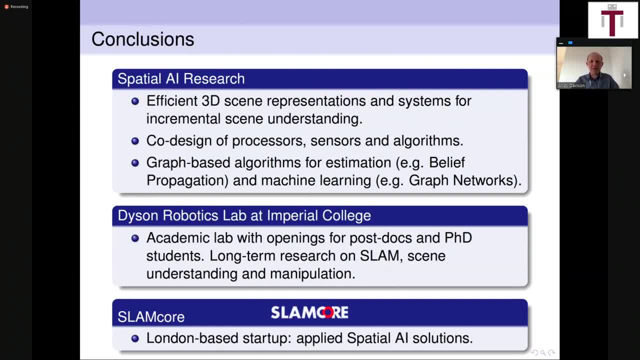 for a number of years yet. So it involves computer vision and robotics, deep learning and representations, but really focused on how can we put all of those things together to enable incremental, efficient scene understanding, taking into account also, ultimately, how we will lay these things out on hardware. 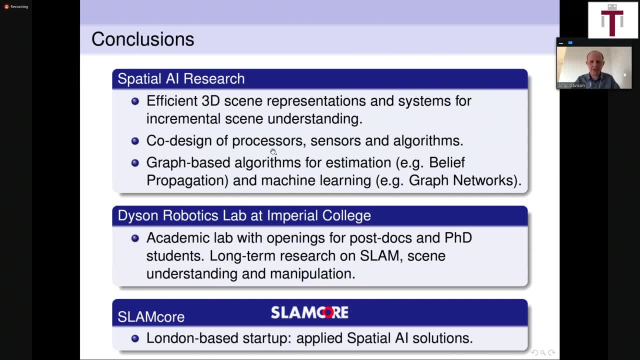 And then, of course, the design of processors, sensors and algorithms- I think is super important- And, as I've mentioned, graph-based algorithms for estimation, such as belief propagation, and also graph-based machine learning, something I haven't really worked on much yet, but I think is clearly. 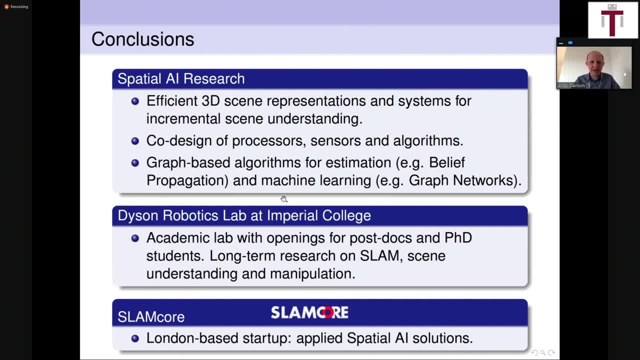 going to be a key part of this. So I'd just like to mention my affiliation. So I'm leading the Dyson Robotics Lab at Imperial College. I'd like to thank all of my colleagues there and also my collaborators at Dyson who support us. 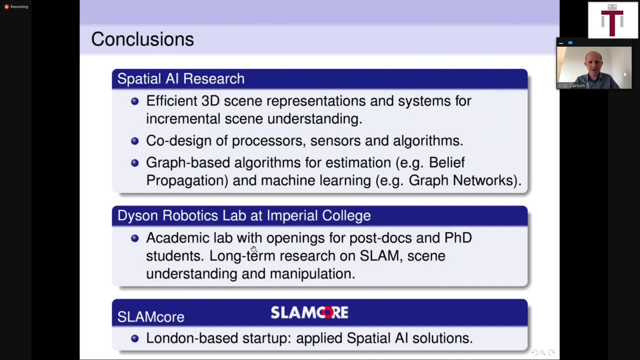 So this is an academic lab with postdocs and PhD students And we really do long-term research, academic publishable research, on SLAM scene, understanding and manipulation. And finally, to mention SLAMCORE. So SLAMCORE is a London-based startup. 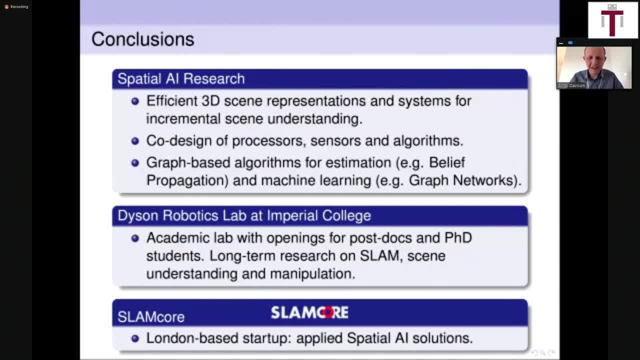 which I co-founded with other previously academic colleagues, And we work on applied spatial AI solutions. So thank you very much. Thanks, Andrew, for the inspiring talk. I loved the entire talk. I loved the amazing results and videos, of course. 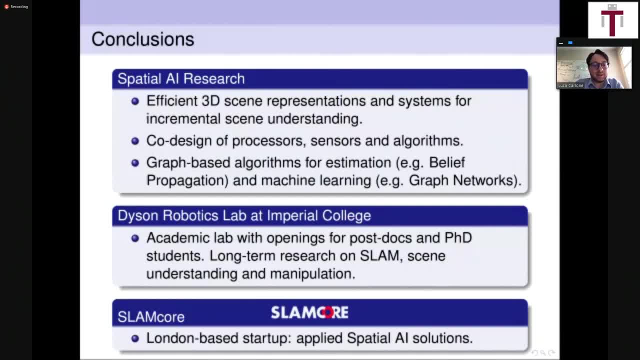 But I also really, really appreciated the vision and the broad perspective that you gave on the entire field of perception, which I believe is a great service for the community, So giving this kind of vision and understanding and perspective. So I'm sure that in other circumstances 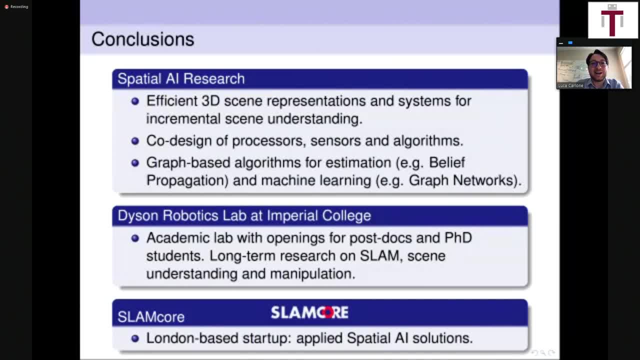 we would have a standing ovation here, But for now we'll have to settle for a virtual round of applause. So thank you so much for giving this presentation. The plan for the final portion of the event is to have an interactive discussion with Andy. 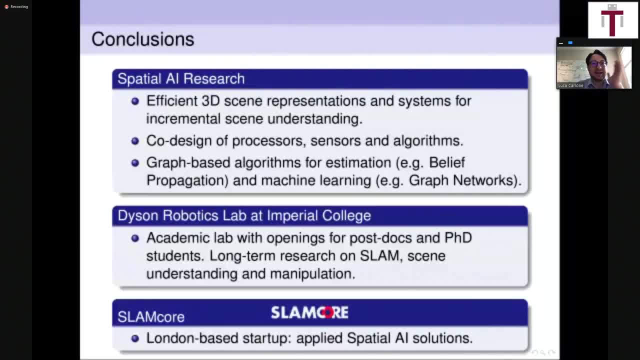 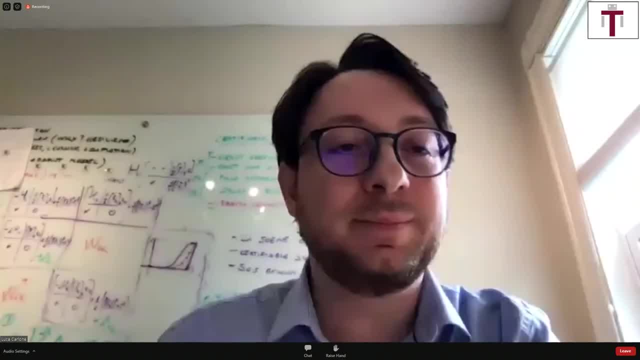 And this will happen with the help of our panel. I'm Luca Carlone, I'm assistant professor at MIT And I will be moderating the panel together with Jeanette Vog from Stanford. Thank you, Hi Jeanette, Hi everyone. 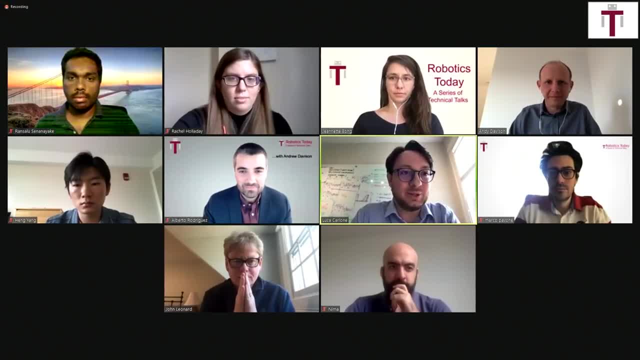 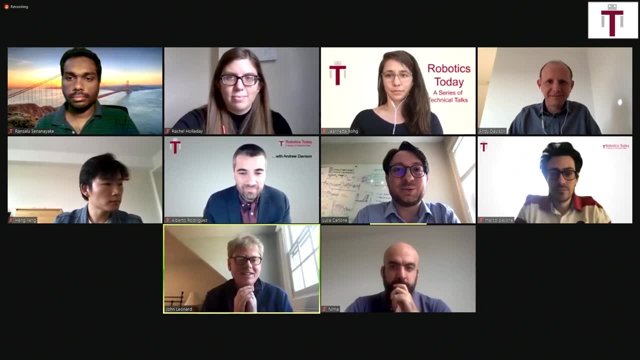 So joining us today. we have our guest panelist, which Alberto already introduced. He's John Leonard from MIT- John, thanks for joining My pleasure- And also we're going to have Marco Pagone from Stanford and Alberto Rodriguez from MIT. 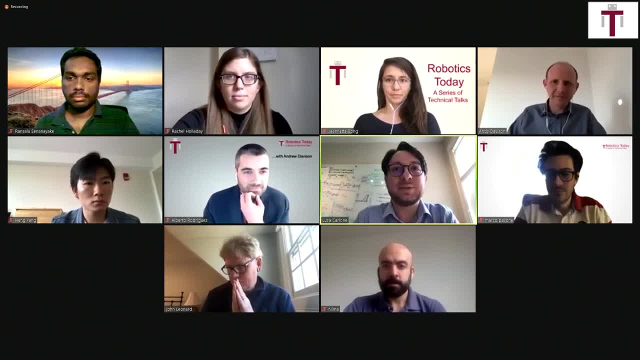 Moreover, we'll get some help from our amazing collaborators, including Heng Yang from MIT, Ransalu Sinanayake from Stanford, Mima Fazeli from MIT and Rachel Holloway, who will help us collect questions from the audience. 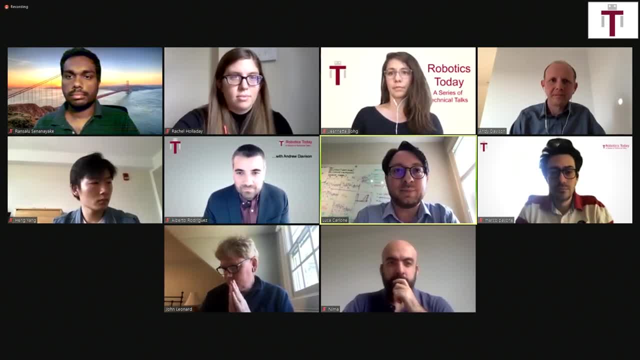 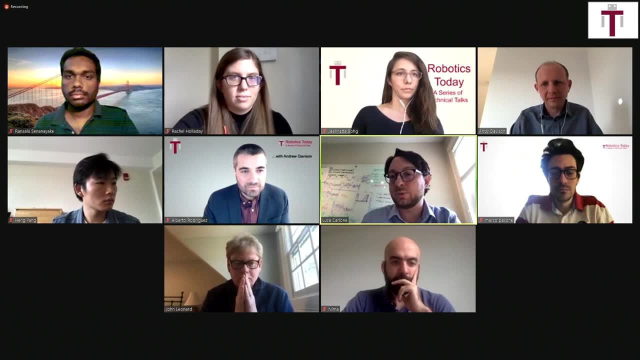 So I invite the audience to post comments using the interface on the event website- And I see that there are really many questions flowing- And I also invite the panelists to use the reason function to ask questions on our site. So, of course, I have a number of questions and curiosities. 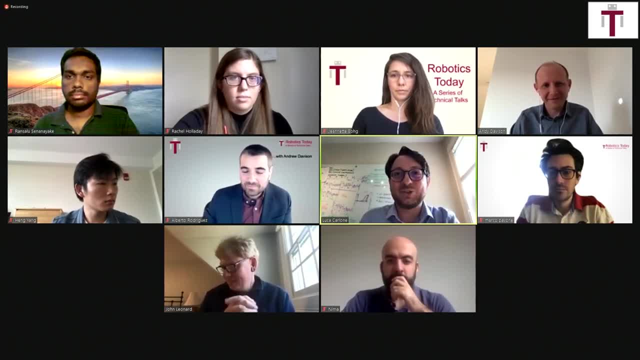 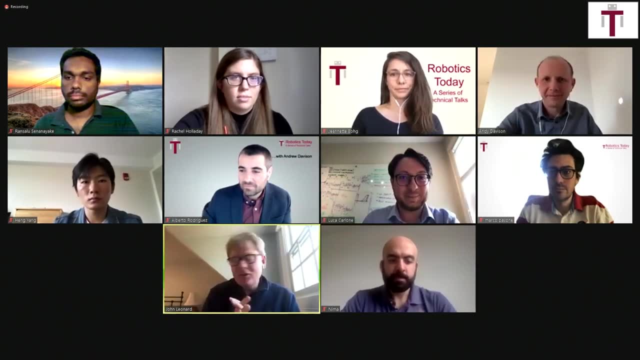 that I would like to ask Andy, But I will actually invite John Leonard, as our guest panelist, to start with remarks and questions. John, take it away. Thanks, Marco. Thanks Luca, Andy, wonderful talk. I have dozens of questions myself. 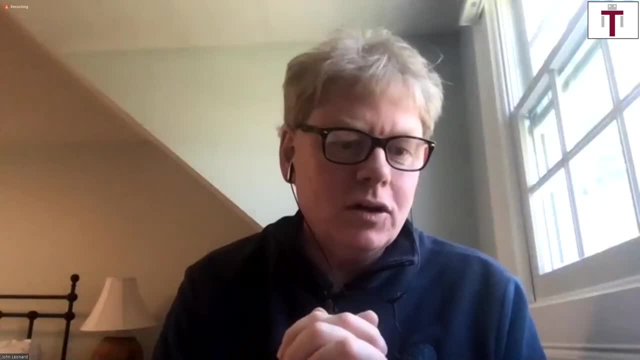 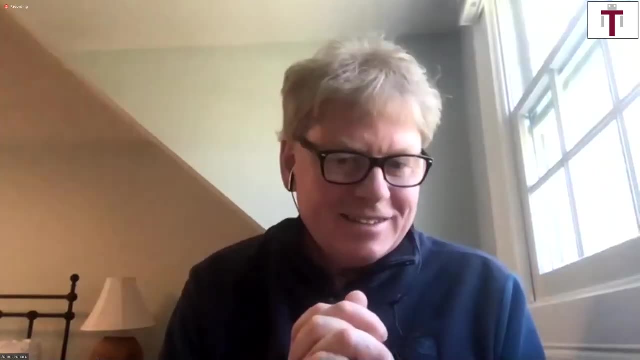 I'm so excited to see this sort of- really this three decades worth of work. I remember- I think it was in 1999, I was an assistant professor And Andy sent me an email. He was a postdoc in Japan And we started a conversation that's now gone for 30 years. 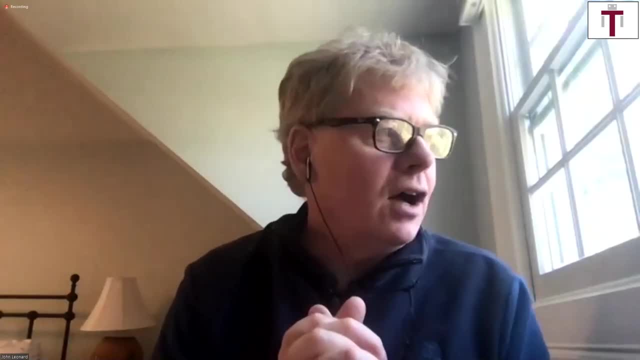 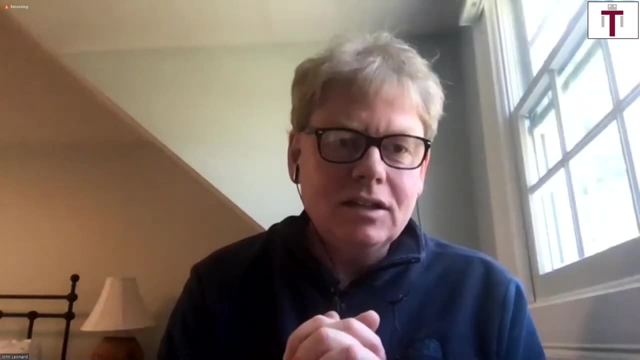 And I'm reminded of Amara's law, which says that we tend to underestimate the impact of a technology in the short term, We tend to overestimate it in the short term, but underestimate it in the long term, And I think that's kind of really. 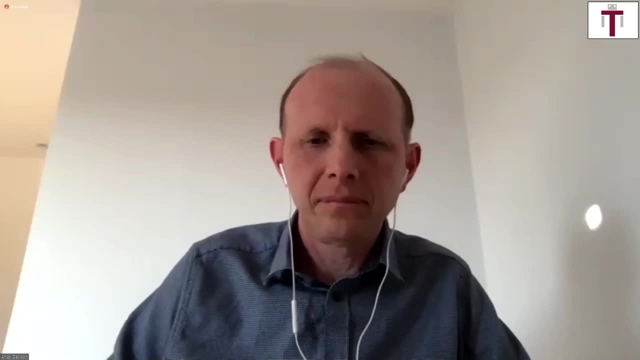 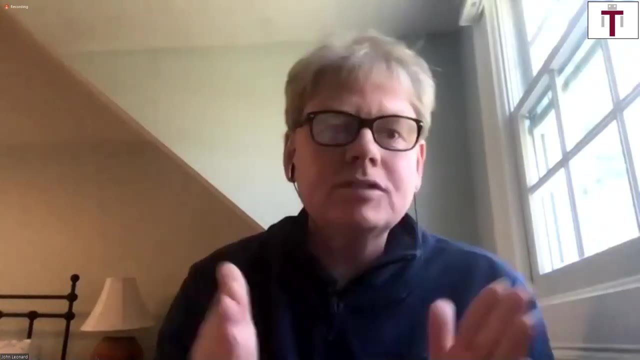 where we are with visual SLAM and spatial AI, that I think in the very long term, decades from now, this technology really can be ubiquitous to make life better for lots of people, And we've come such a long way. but there's. 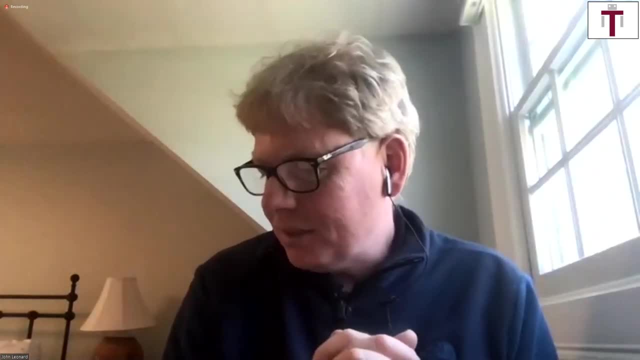 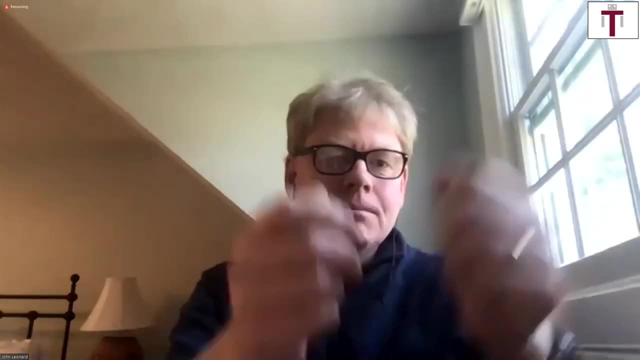 a long way more to go And, picking amongst the many sort of topics I might ask, I'll go to the question of robustness. I've always dreamed of having apt-get install SLAM, so that say, someone working in manipulation maybe. 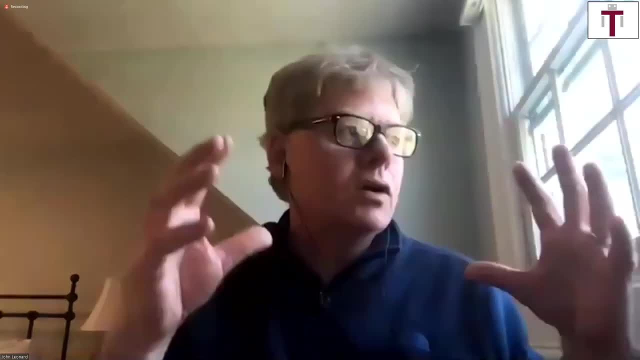 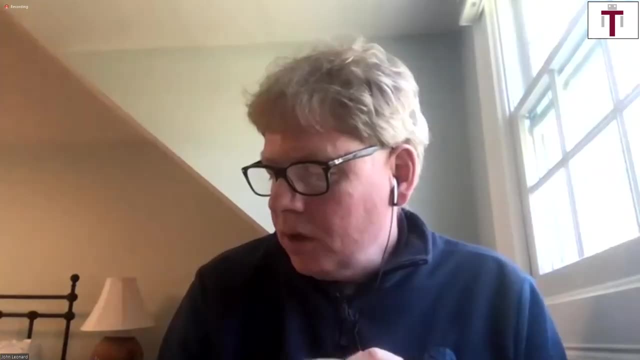 mobile manipulation. they might just have this competence, this competence of knowing what is where in the world, that spatial intelligence, That's something they could just kind of take for granted and trust. And so I'm guilty myself. In the lab we make wonderful videos. 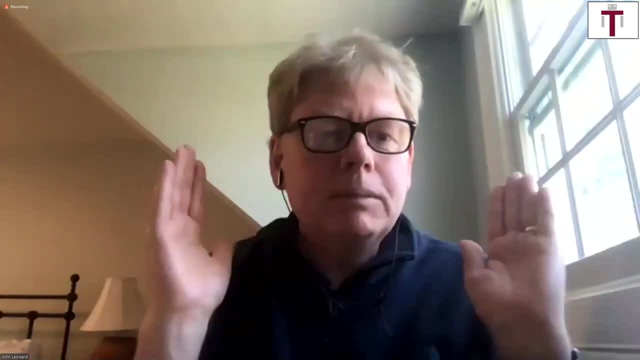 But how do you make a system where you could just be blindfolded in your lab and you would say: John, I'm going to press go and I'm going to leave or close my eyes, And you knew it would just work. 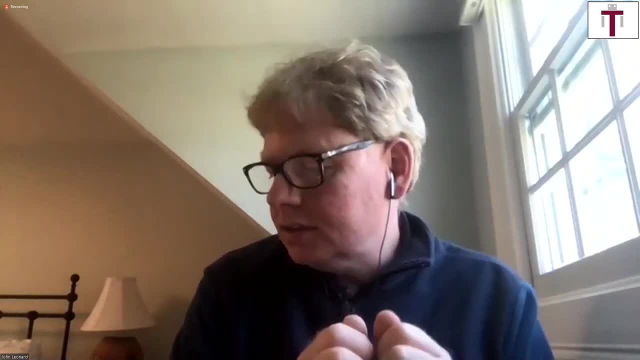 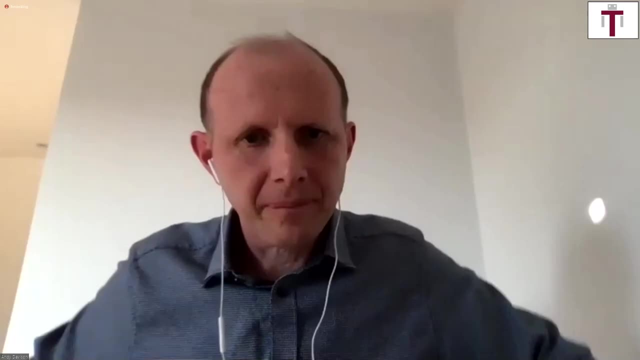 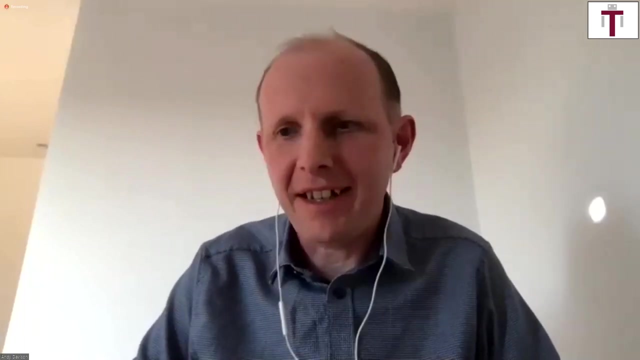 Where is the elusive robustness where you could truly trust 3D? you know, object-based SLAM For, say, manipulation? Yeah, great question. So, of course, yeah, I agree that there's such a massive gap between the thing you see in a paper. 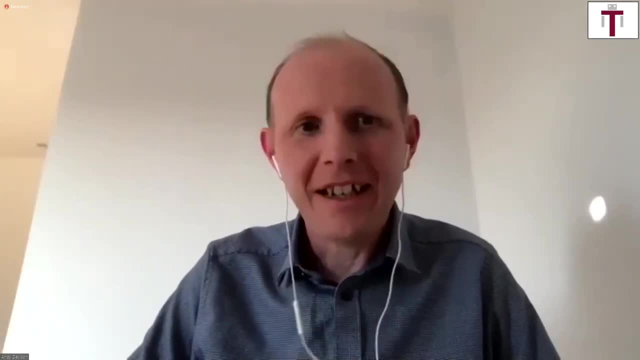 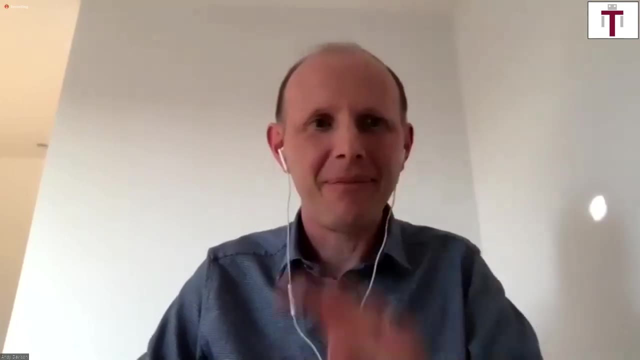 the cool video of the style that I've showed In my lab. I've generally tried to go one more step than that, which is the live demo, So I've always been very keen on going to a conference, To your great credit, which I'm a big fan of. 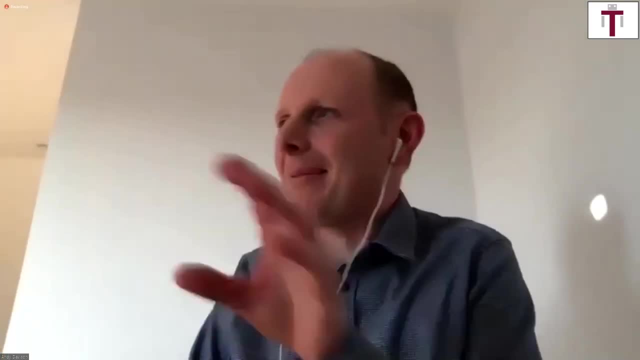 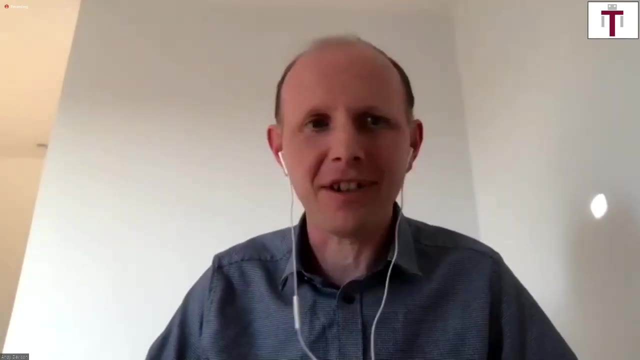 With a laptop, With a laptop and wave a camera around and show something people can actually interact with. But there's another huge number of steps beyond that to actually real product And of course I've experienced that with my work with Dyson. 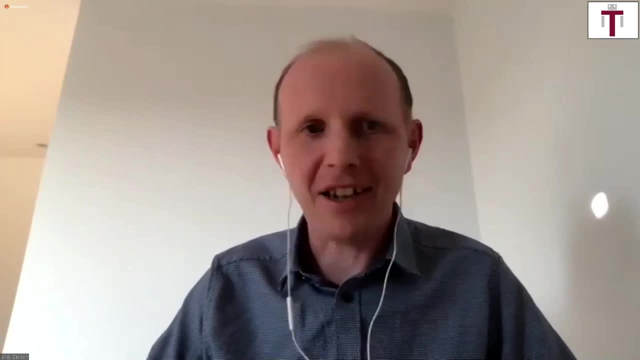 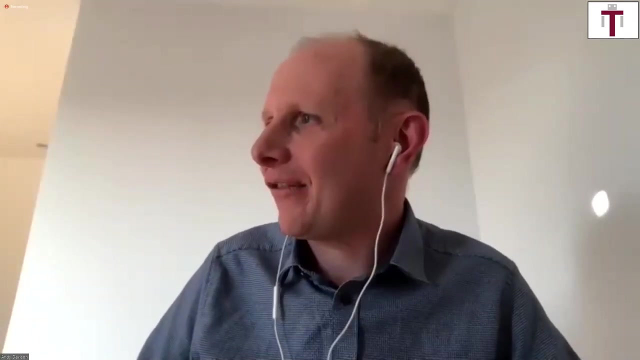 So just the amount of testing and just basic engineering that needs to be done, And I still haven't seen any indication that there's any magic bullet there. I don't think, But there's some massive amounts of testing, finding all the problems and edge cases. 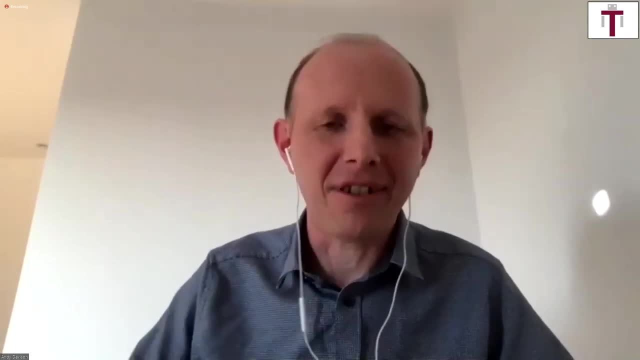 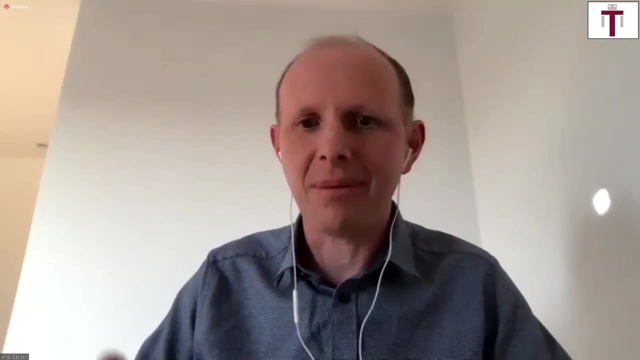 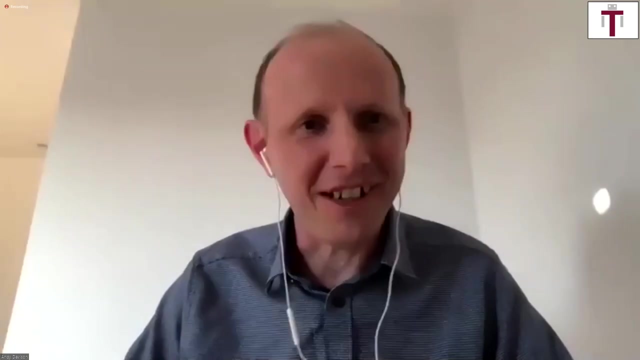 So of course, we have some hope that things coming in, such as learning, can be very important parts of improving robustness. So, as we probably all know, this general idea of image correspondence is probably always the data association, as roboticists call. it is always the hardest part of the process. 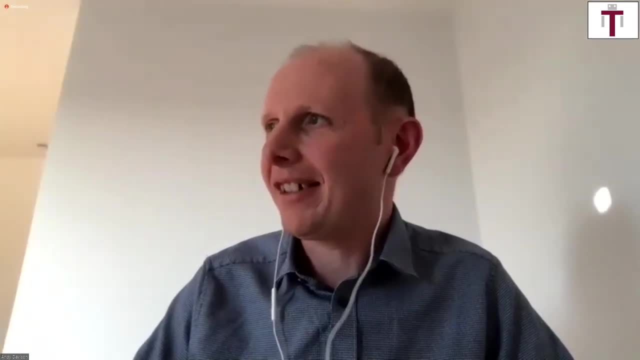 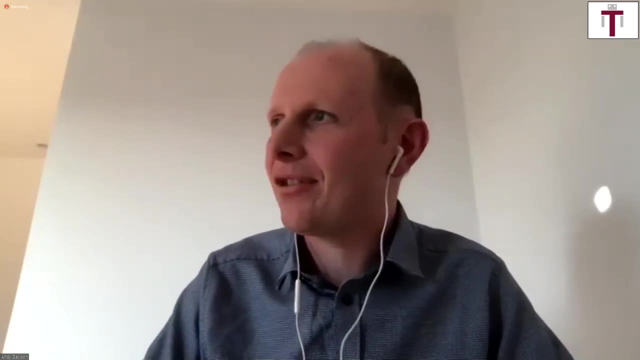 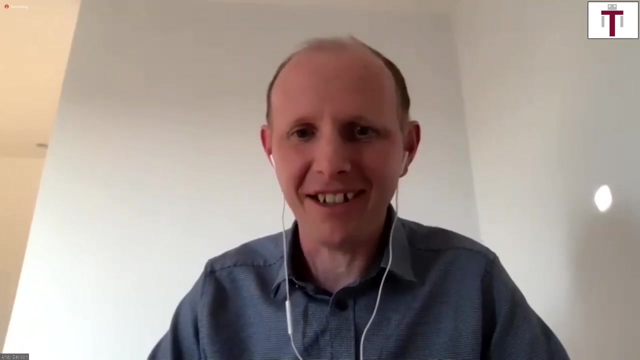 Yeah Of SLAM And clearly we see now that learned mechanisms are able to do a lot better in that. But now maybe we're in a bit this trap of how do you know that your data set that you've trained on fits the place that you're actually going to test in? 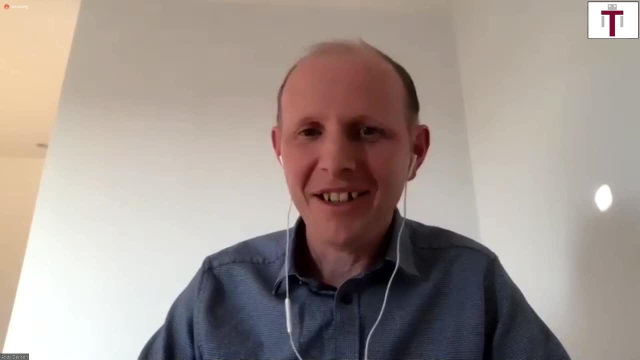 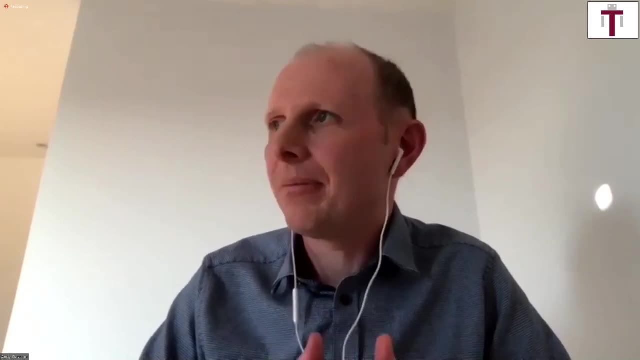 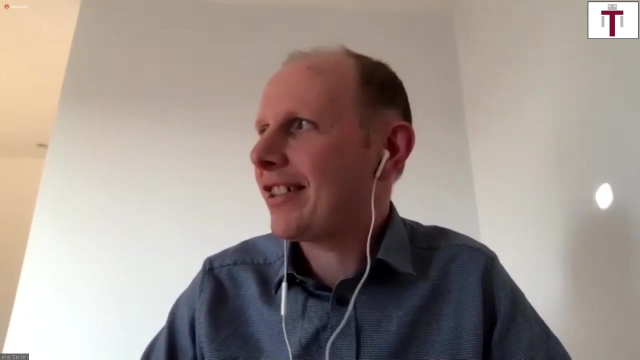 And that's something that I've actually got a bit frustrated with recently. So actually, some of the things I'm most excited about at the moment are going towards sort of unsupervised or self-supervised learning. So actually, for instance, if you want a neural network, 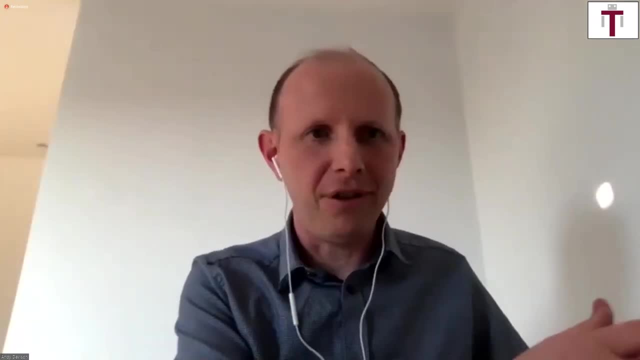 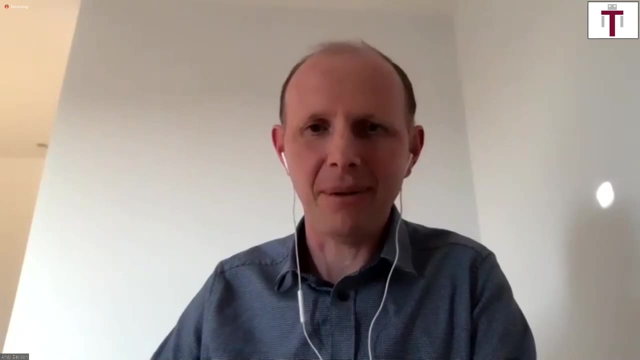 to segment the objects in a room. yes, you could have a neural network and you've trained for semantic labeling in some other scene and you can test it, But it may not work that well. I think what you really want to do is get data in the space. 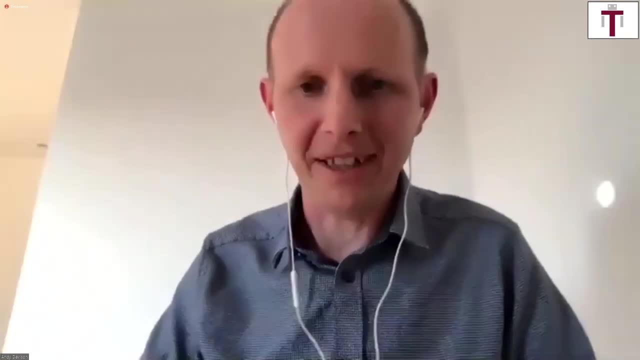 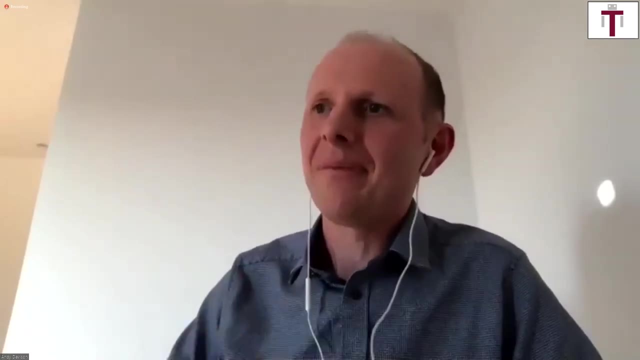 that you're actually in and learn as best as possible in that scene. Of course you won't have high quality labels necessarily, But I think you can go. You can go an awful long way with unsupervised learning, And then maybe there's a fairly small amount. 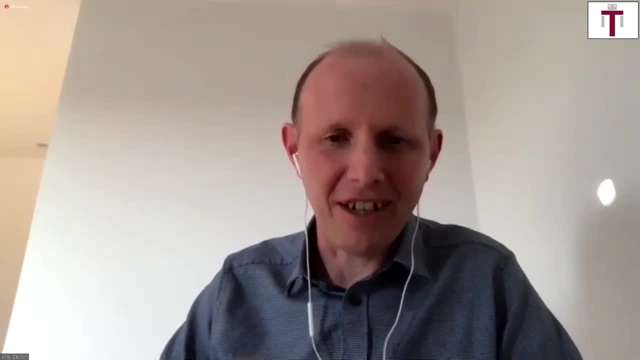 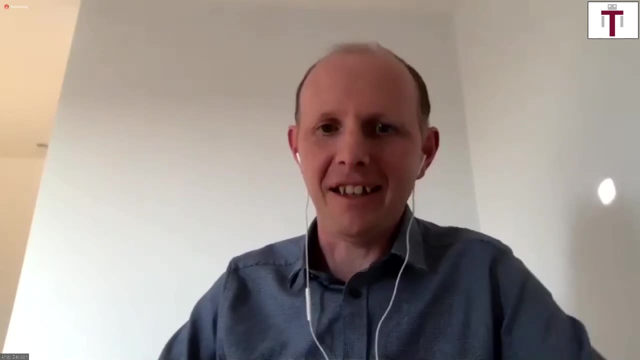 of labeling needed at the end to actually relate to what unsupervised learning has learned, which is more or less clustering, and relate that to labels that a human would understand. I agree with you: Just a quick follow up and then I'll turn it over to others. 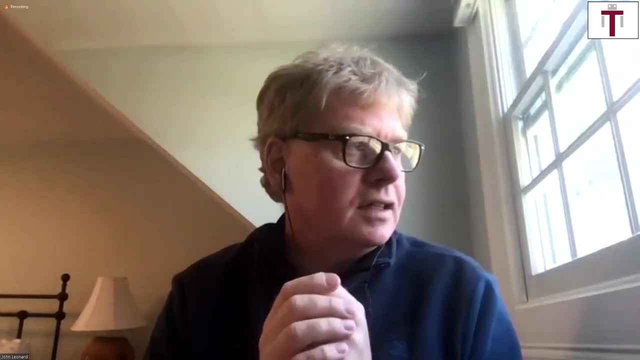 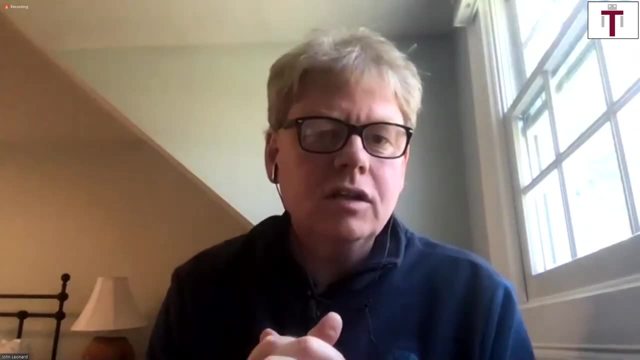 In his 2019 ICRA keynote, Yoshua Bianchio quoted Butoh saying: nature doesn't shuffle the environment, And I think something that we can offer the machine learning community is that- this self-supervised vision, or just that- an agent that's controlling its own motions. 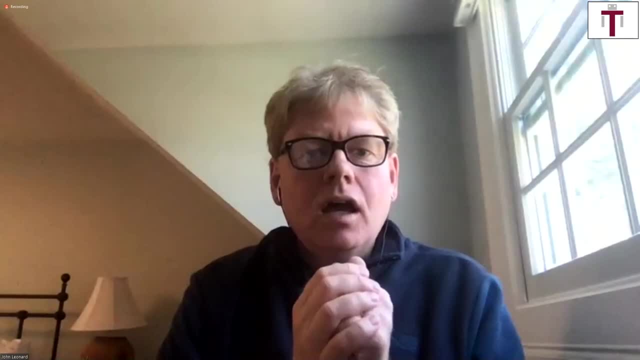 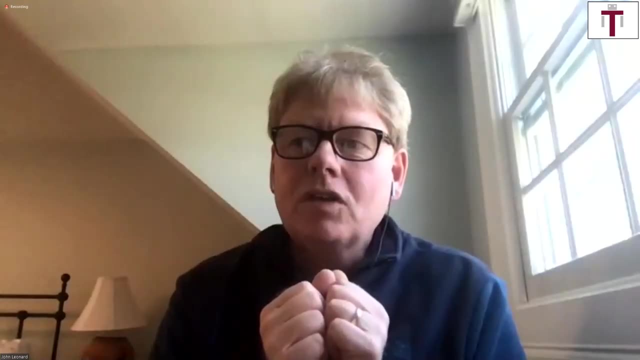 and moving through the world with a notion of space and time. it's a bit like having the cards in a playing in sequence versus ImageNet just pulling randomly from the internet. disparate And I think that notion of spatial context, that is the path. 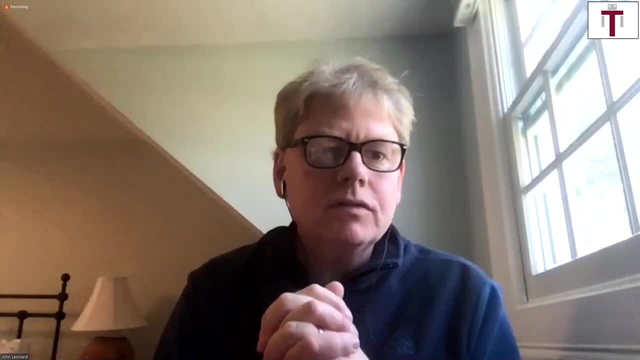 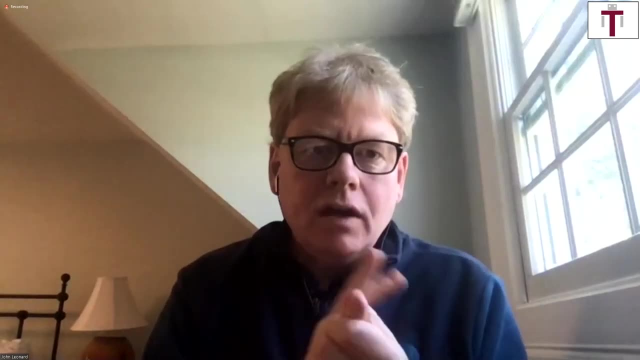 Because, even though machine learning has obviously made incredible strides, I worry about where we are on the ROC curve And I think we're very far from very high probability detection and very low false alarm systems that we could use, for example, for autonomous driving. 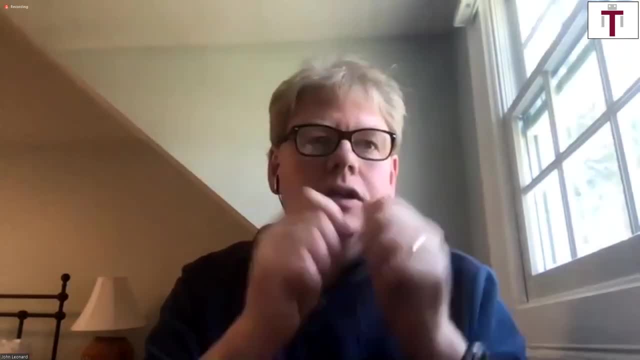 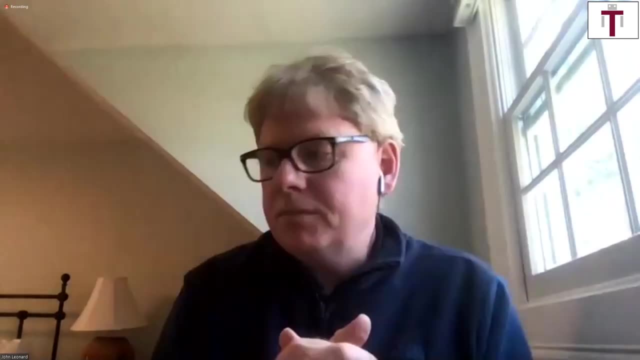 in highly dynamic environments And so the robustness that I want is sort of the perfection point on the ROC curve where we really know we can trust it. But I think a lot of these methods you've mentioned about object-based representations and new types of processing the message passing 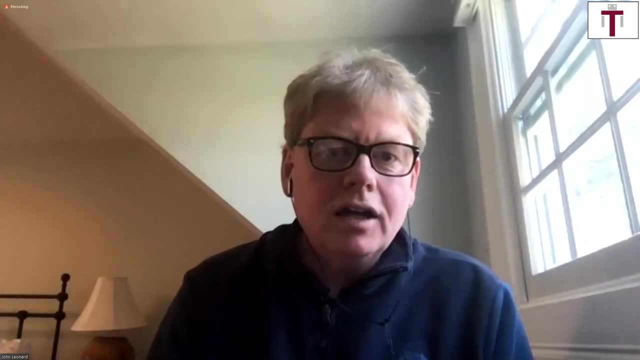 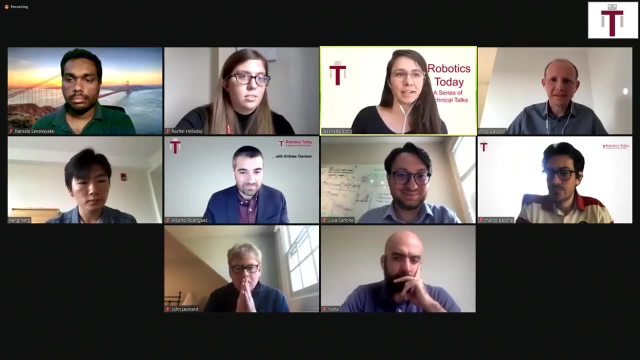 it all fits into. I think we've got much more great work to do, And thank you, Thanks. Thank you very much, John, for your question, So I think we're going to now take on some of the great questions- And there were actually many- from the audience. 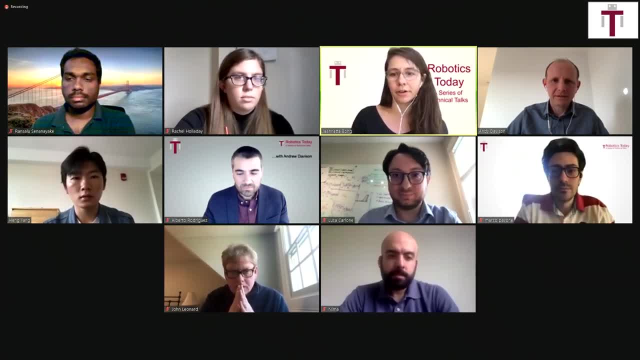 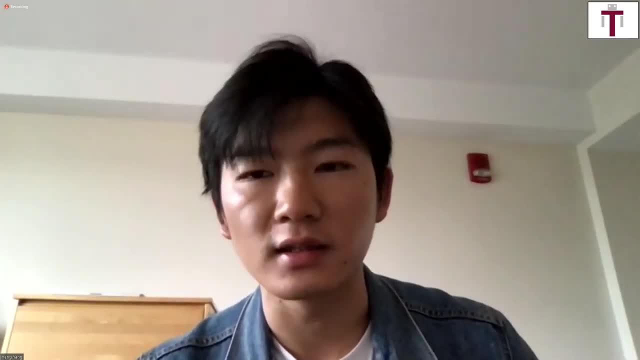 So, Hank, you have selected one question from the audience. Can you give it to you? Yeah, Thanks, Andy, for the nice talk about perception, vision and SLAM, But I have a very highly ranked question from Harman Rohit. 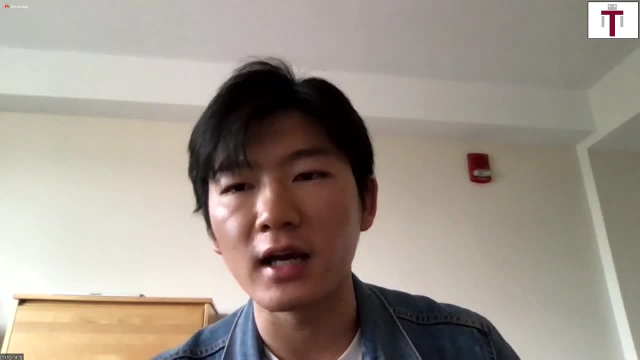 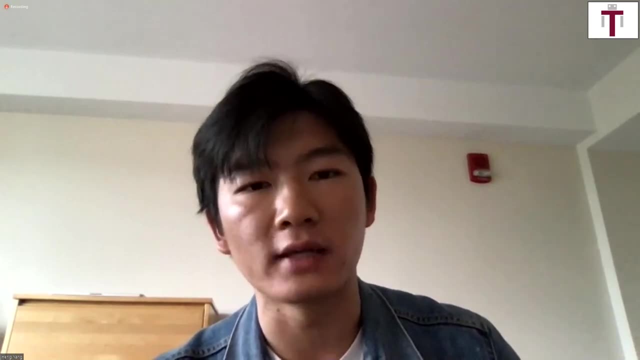 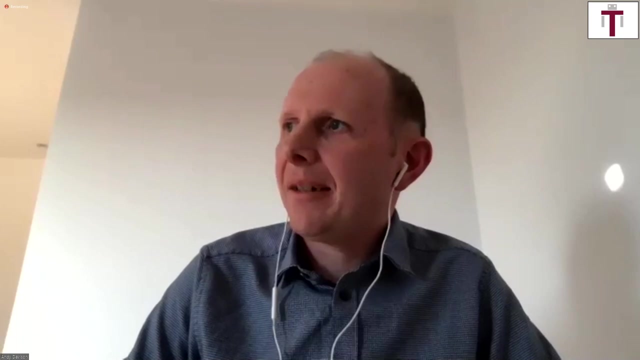 that asks that, rather than solving SLAM as a standalone problem, What are the new developments in active SLAM, in particular with control and planning in the loop as well? Yeah, great question. So no, I mean, I'll put my hand up straight away. 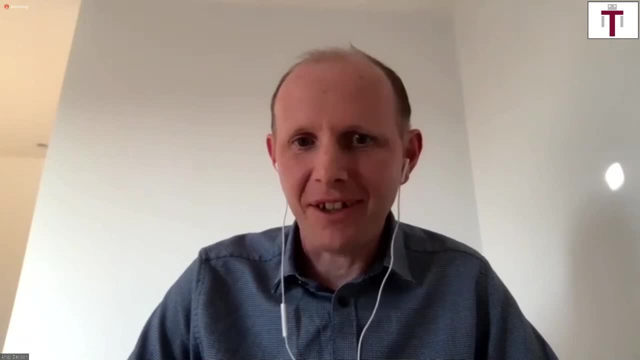 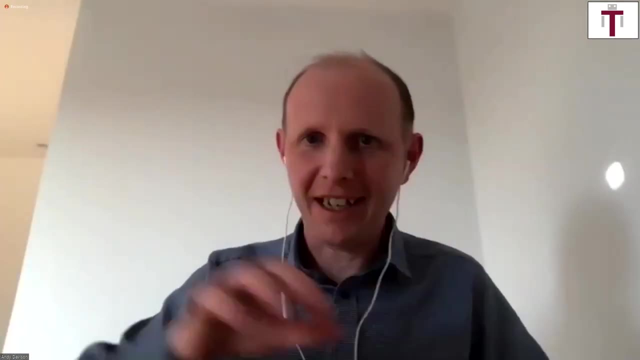 and say it's not something. I've worked on very much And for a lot of my career. the output of the work has been: this is the video, this is the map, this is the camera trajectory that we've estimated, But very clearly. 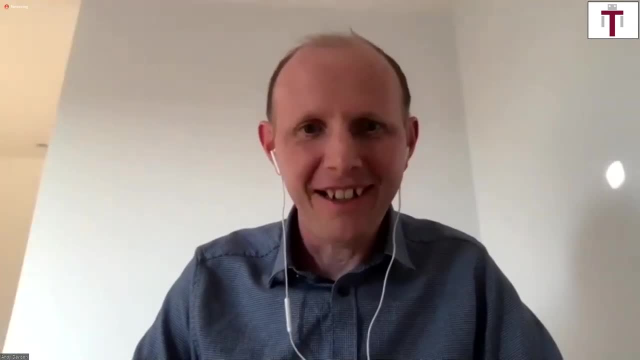 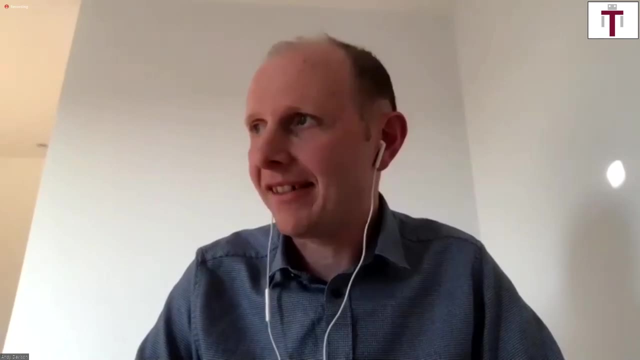 That's not the end goal. The end goal is embodied intelligence manipulation And, as you see, we're really trying to work on those things now. So it has to be said that there hasn't yet been much feedback in any of the things we've done from the action to actually improve. 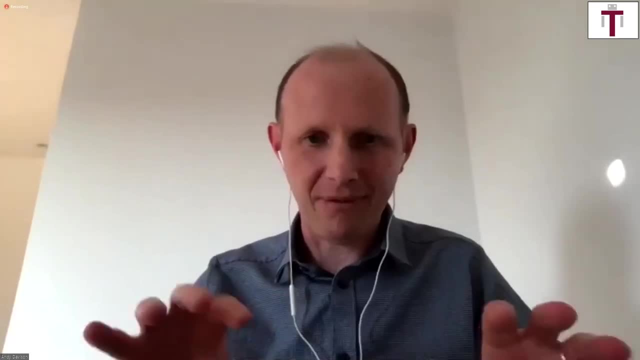 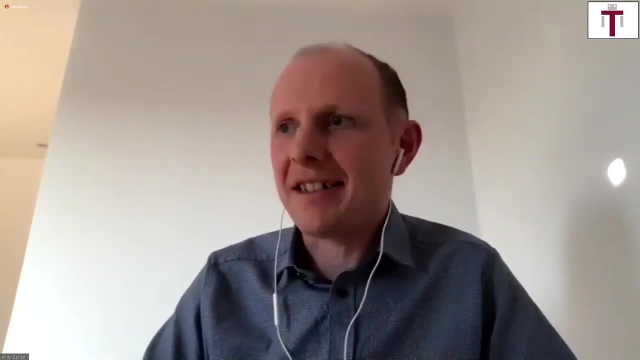 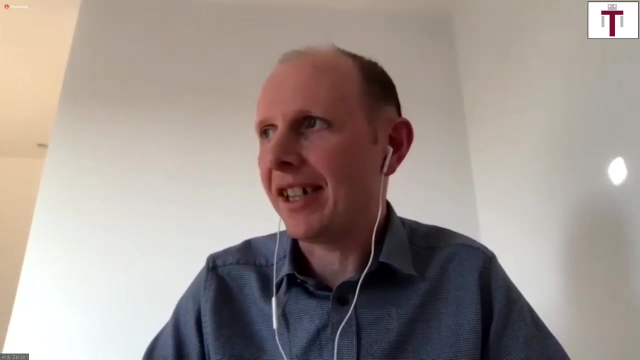 the representation. So we scan a scene, we get the representation from vision and then we act. But clearly, once you start touching the scene, understanding the physics of how things move, then that should, Yeah, Really improve your perception and feedback on it. 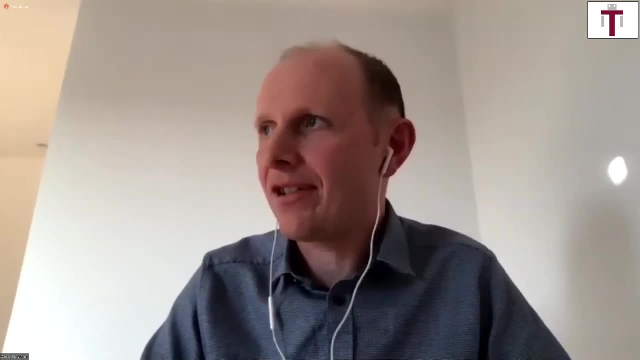 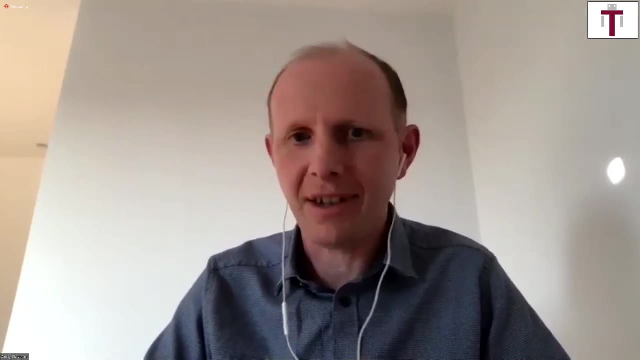 So I'm really, really interested in going in that direction. So, for instance, bringing physics simulation into the perception system is something I'm very interested in. So in the system, I showed you with a pile of objects that the robot was going to interact with. 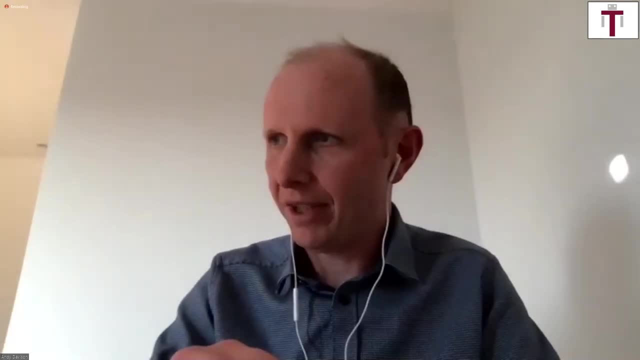 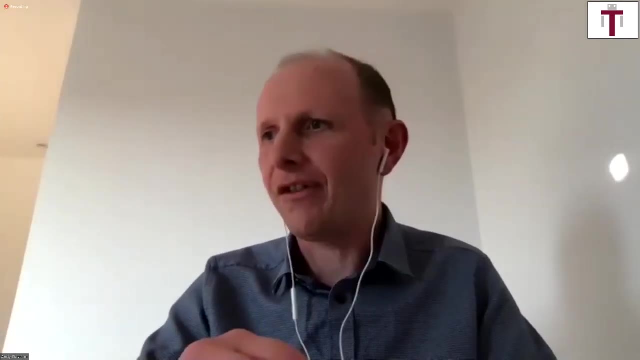 So when we're estimating the positions of those objects, we do take account of the fact that the object shouldn't be intersecting Each other. But we could go further and for instance say: well, physics says that this object can't. 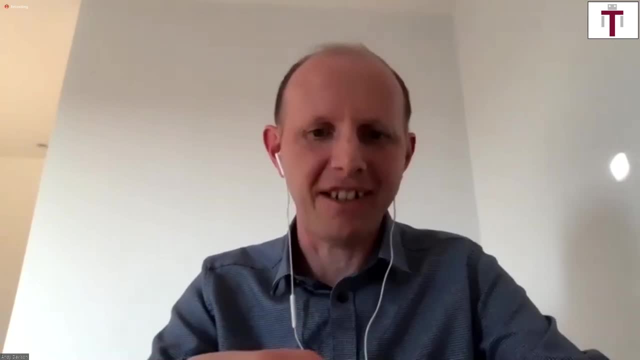 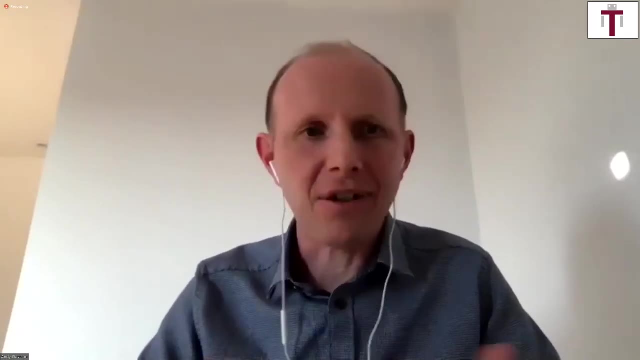 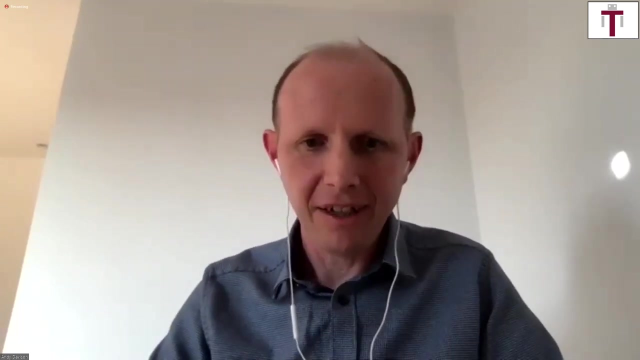 be floating in the air, So there must be another object kind of right underneath it which is supporting it. So bringing that kind of physics into the actual estimation of what's going on And then hopefully then rolling that onwards So as the robot then starts to interact with the scene. 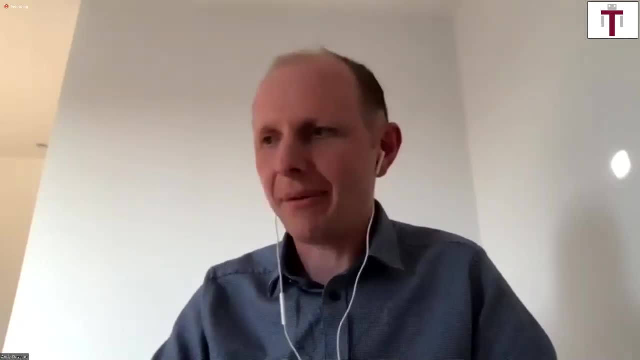 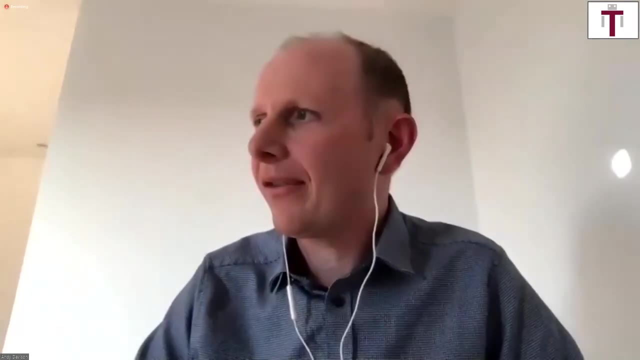 and maybe poke one of the objects and sees how it moves. you know, we probably We may get some kind of force information from the robot, But we'll also get some updated visual information. But then we've got to come up with a new estimate, which? 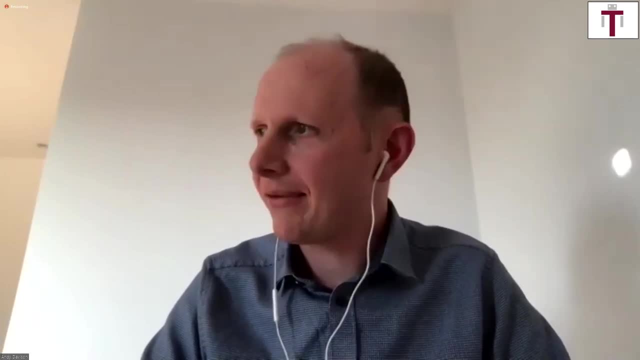 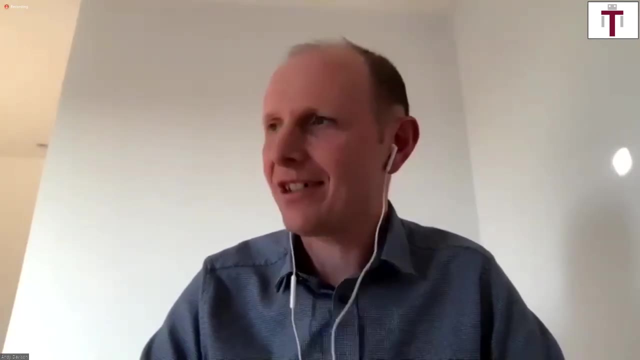 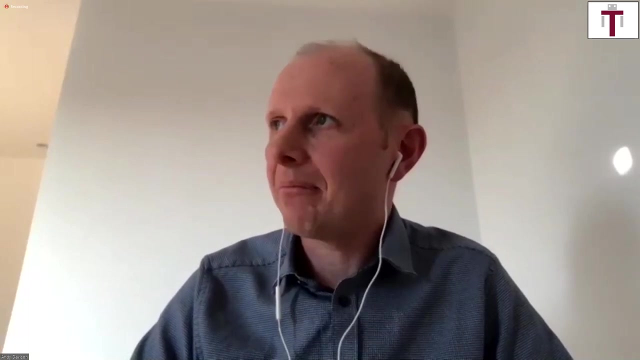 is still consistent with physics. I think those things are very hard because simulating physics of contact is incredibly difficult And we've tried lots of different physics engines and so on that have different strengths and weaknesses. But yeah, Those are things, Those are directions I'm really interested in. 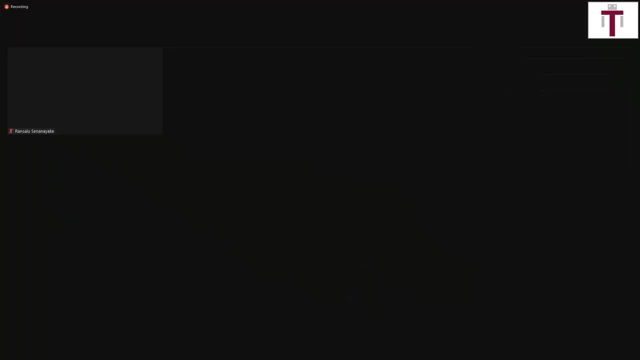 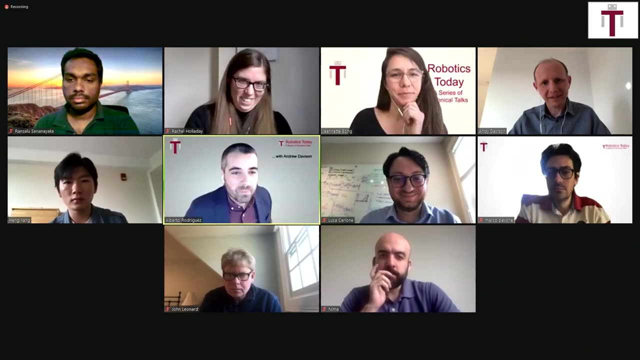 but can't claim too much progress so far, OK, OK, Looking forward to it. Adato, you have a follow up on this one. Yeah, I wanted to follow up, Andy. So if you bring physics into the estimation loop, 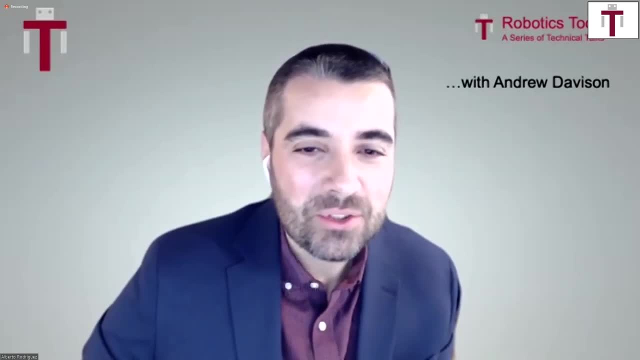 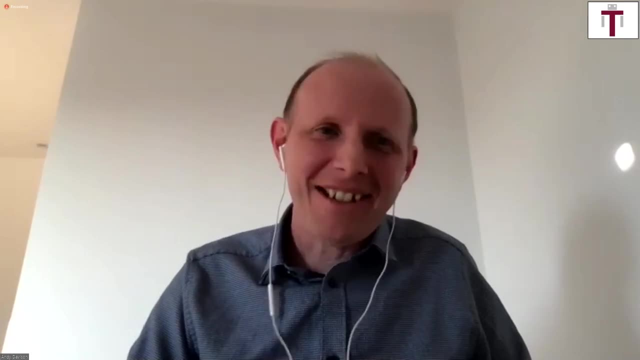 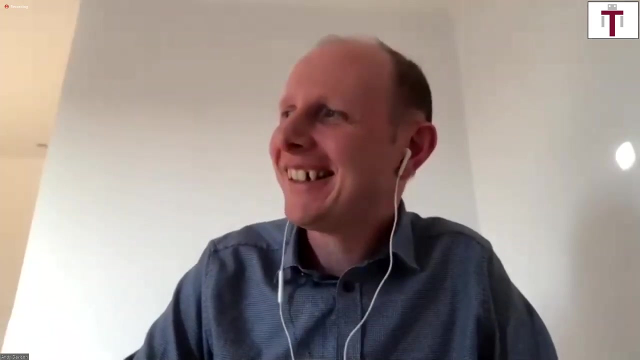 would you still call it the spatial AI, or would you have to change the name? I don't know. I'd still try. I wouldn't claim that name, but I don't know. It's up to everyone else whether they accept that. 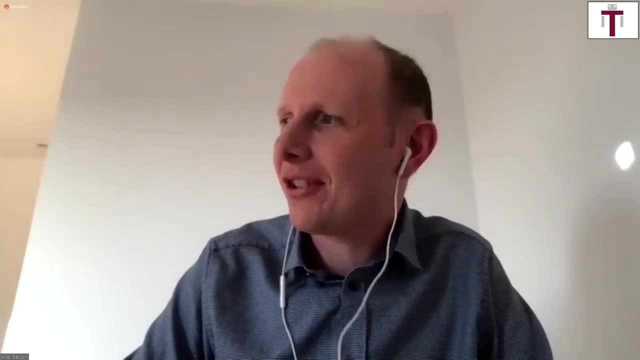 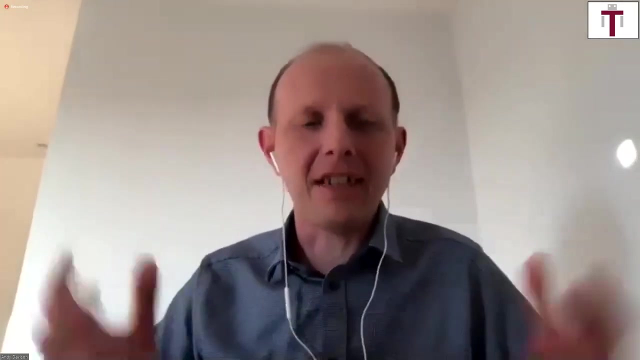 I think so. I think embodied spatial intelligence involves all of those things. It's about all of the sources of information, sensing and priors that an embodied agent needs to use in order to understand enough about the scene to do intelligent things there. 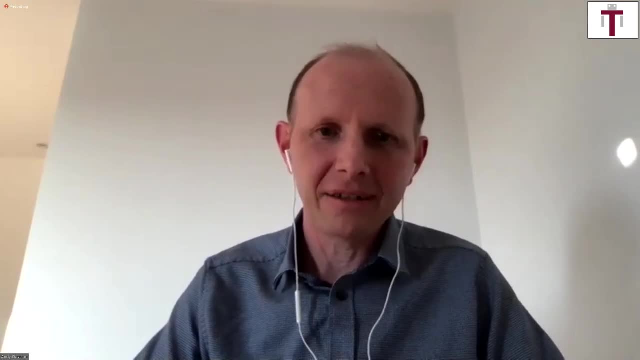 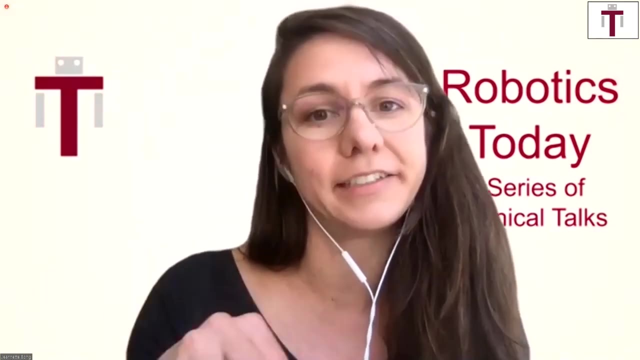 So, based on that definition, I think, yeah, OK, I think it still fits Right, Thanks. So I was actually also a follow up question: When you were grasping the objects, they did stay in the gripper. Did you not take any visual information? 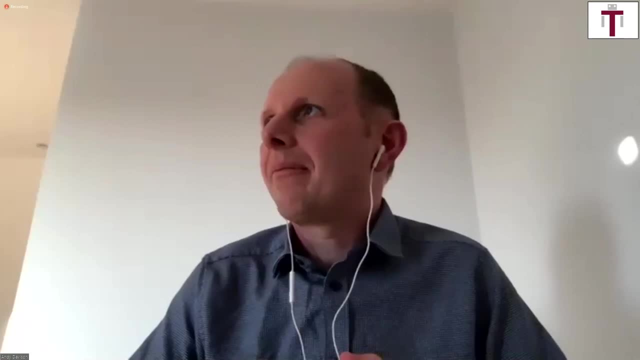 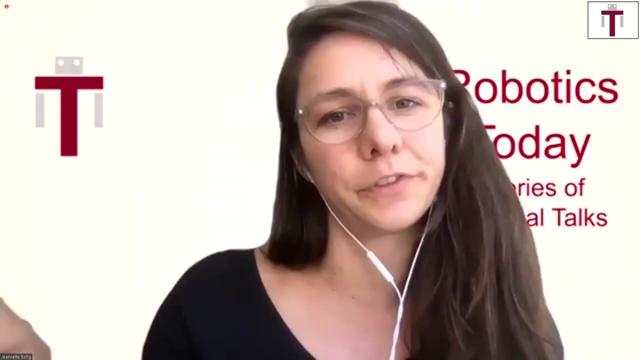 into account to track it. So we, to be honest, we're doing something fairly. you mean, once they're actually grasped, Yeah, and then they're moved into the box. They were actually moving with the gripper. They were wobbling a little bit, do you mean? 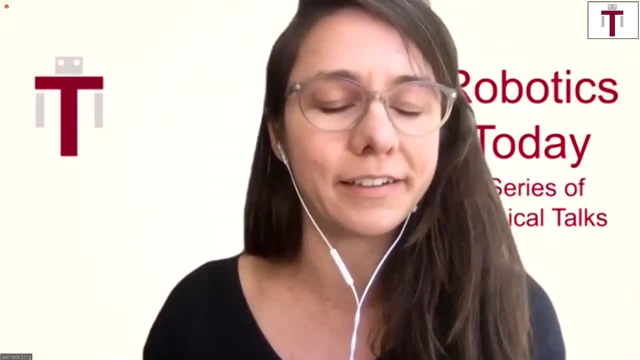 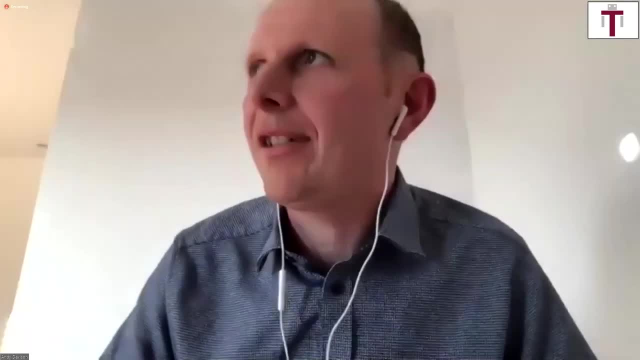 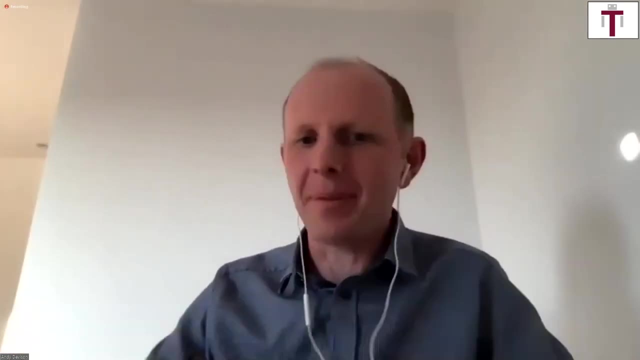 Yeah, They were just being transported right, But I wasn't sure if this was actually tracked visually. No, So at that point we were assuming that once we grasped the object, the object would stay in a fixed configuration relative to the hand until we place it. 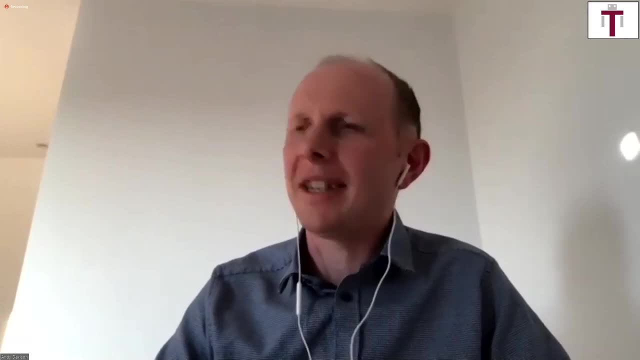 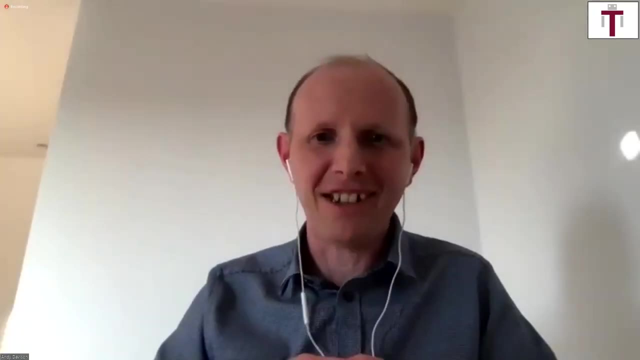 But certainly that might be possible. I mean, it's difficult with a depth camera on the hand, because the range of the depth camera is normally the minimum range is such that you can't necessarily get an accurate measurement of something you're actually holding. 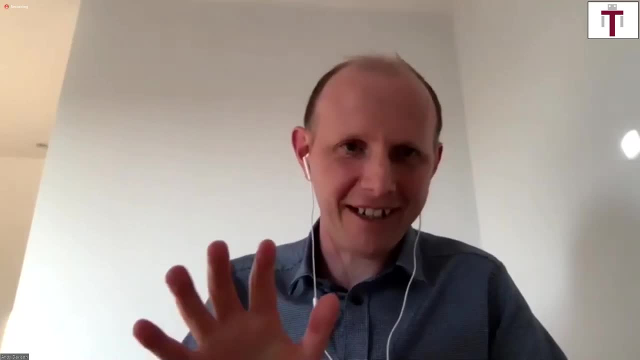 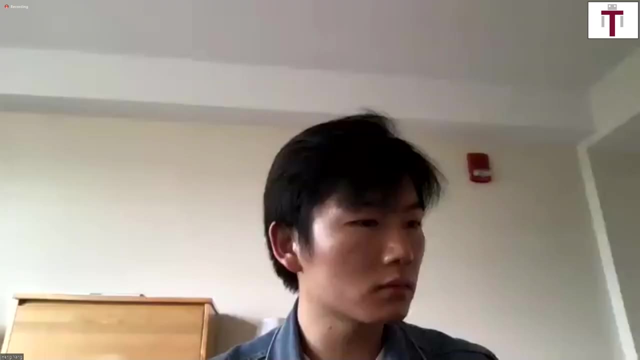 But cameras are cheap. Maybe we just put more cameras, one right there, kind of in the palm or something. Yeah, that would be great. Ransalu, you picked another question from the audience. Yeah, so thanks for the talk, Andy. 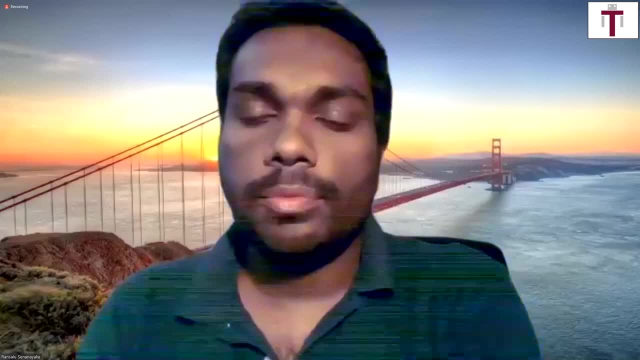 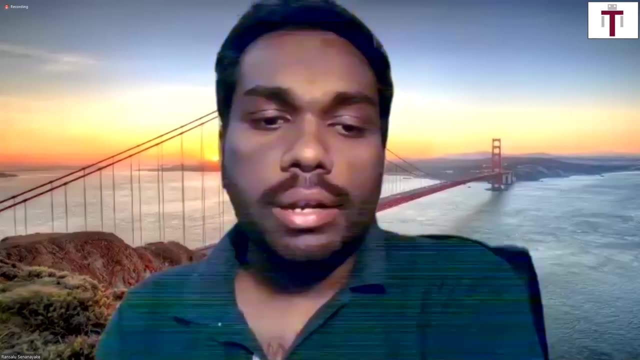 I'm really excited about all the new developments, and this seems to be an evolving field. So we have a question from Karni: Is there an accepted grant goal For SLAM, upon reaching which we can comfortably say SLAM is solved? 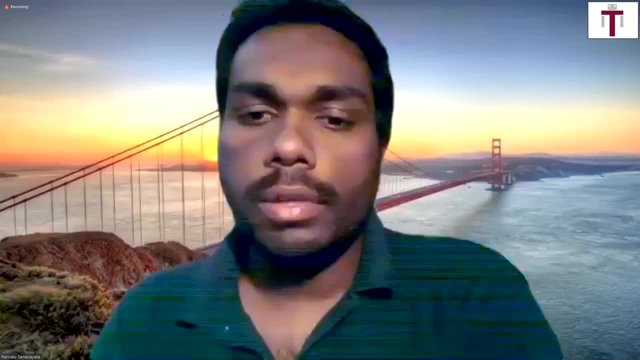 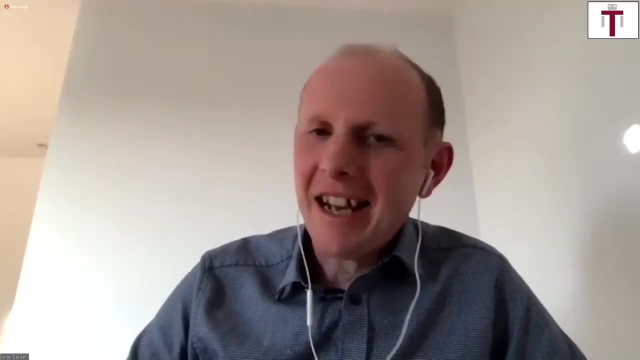 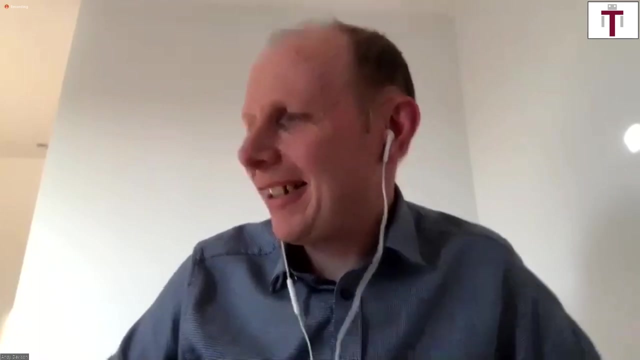 Or do you think it is continually evolving, Or are there any standard challenges for SLAM? Yeah, I mean going back to the question right at the start of the talk. yeah, people have been saying SLAM has solved since 20 years ago. 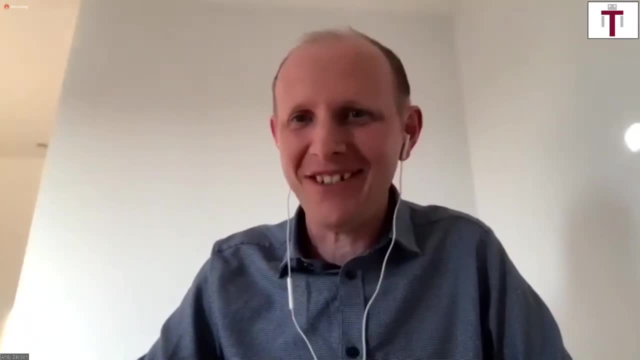 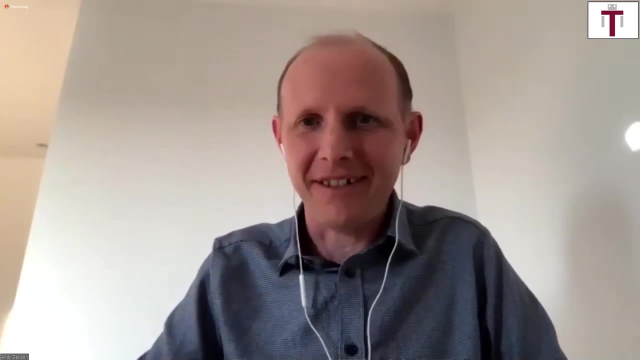 And I've- and I think John have- always been among the people that have said: hang on. I'll immediately give you a way to make it more difficult, like try and do it with a single camera rather than a laser rangefinder on a 2D robot, for instance. 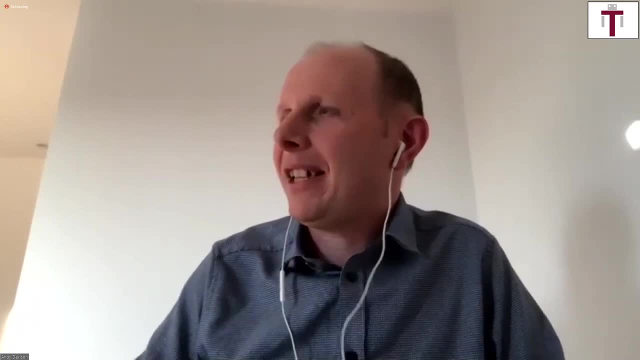 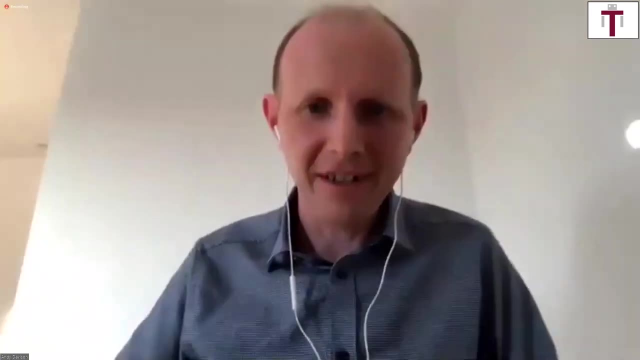 So I wouldn't want to set a kind of fixed target. I mean, I think for me the targets now are really about embodied intelligence. That's what we're trying to get to, and what we call SLAM has to be. It's a means to an end. 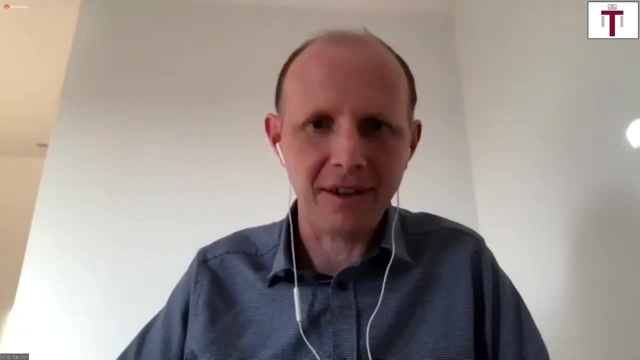 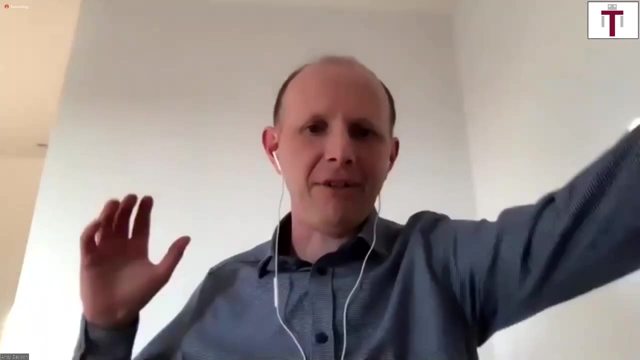 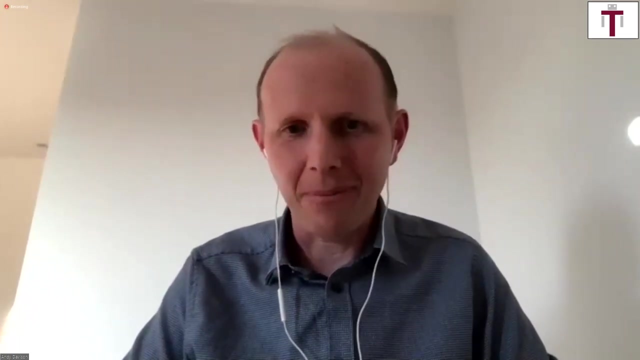 So it could well be that a lot of the things we've done are many of them are not good enough, but some of them are overkill. So, for instance, accurately estimating the metric shape of a building that's 100 meters long probably isn't really needed for many intelligent things. 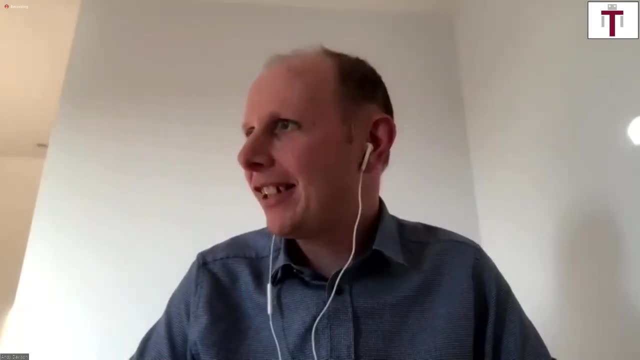 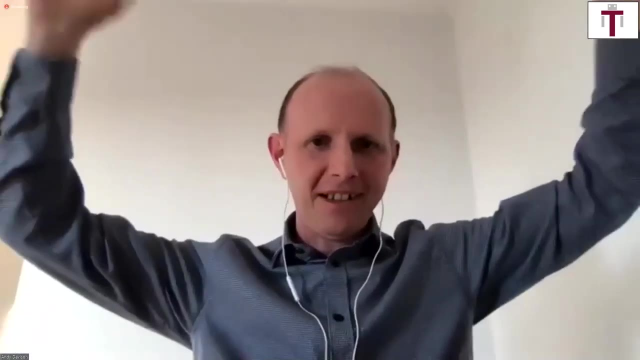 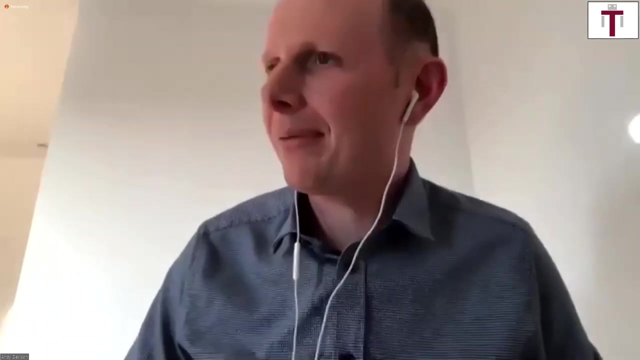 that you would do within that building, or mapping a room with 5 million surfers, especially the parts of the room, like the ceiling, that you're never going to be interested in actually interacting with. So I think the way that we should measure the performance 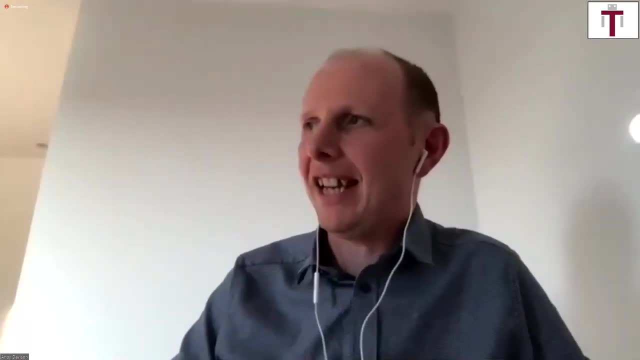 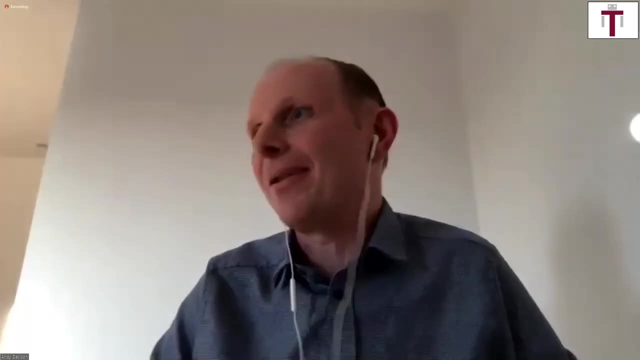 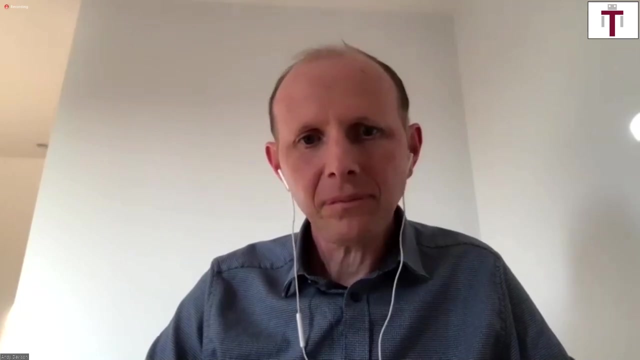 of these systems should ultimately be much more about the end goal, actions and intelligence that they enable, And then we should feed those back into how the SLAM systems work. If I can follow up on that, I think that in easy in quotes: 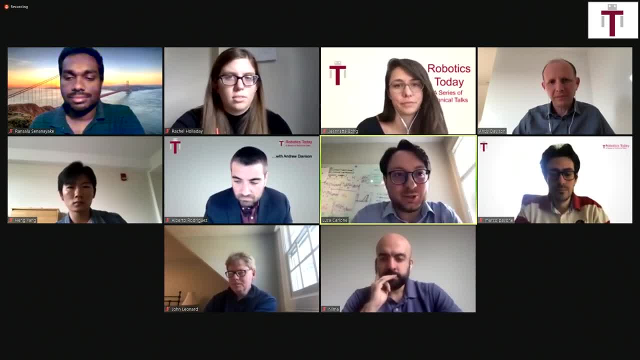 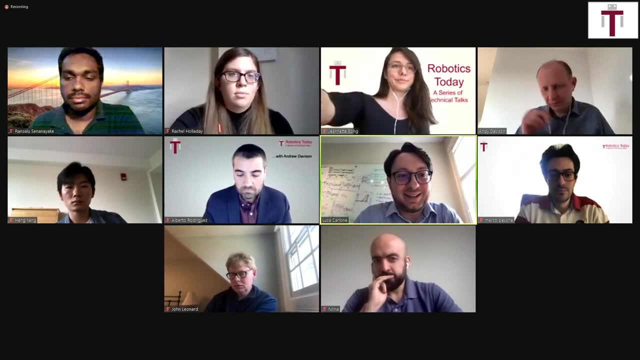 an easy goal is just to see a SLAM system or a spatial perception system to be as capable as a human perception system. So whatever a human can answer using sensor data, it's only to expect for a robot, for a smart robot, to answer. 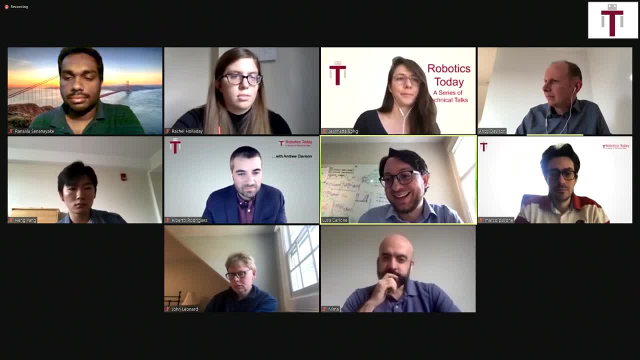 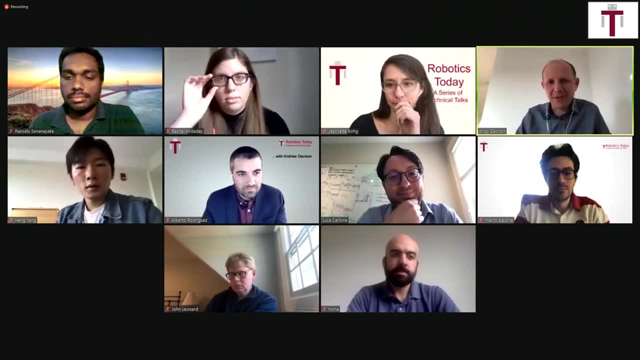 I don't know if it is a definition which is really actionable, but I would love to be at that point. I mean, of course, there's many things that current SLAM systems that can already do that are far beyond what humans can do. 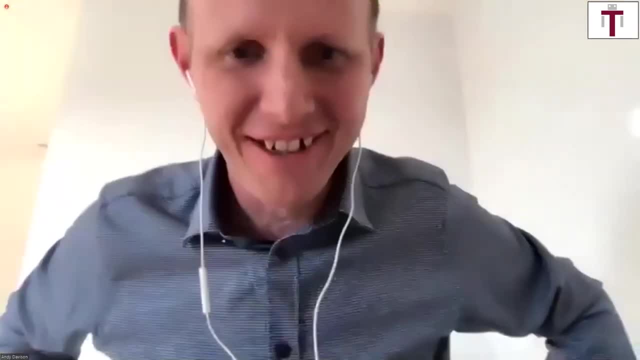 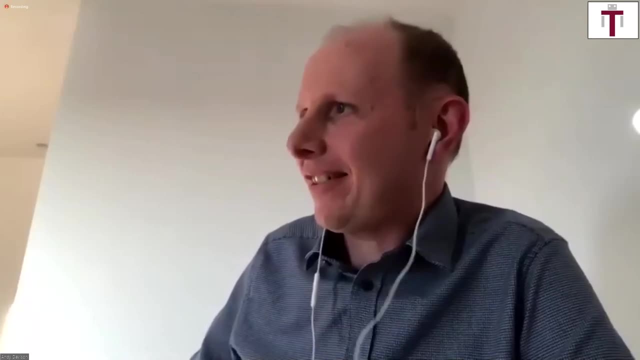 like, tell me the precise distance between those two walls, and your SLAM system will tell you within a millimeter. But yeah, clearly, many things that humans can do with a spatial perception, SLAM systems can't yet. So I think that that's useful. 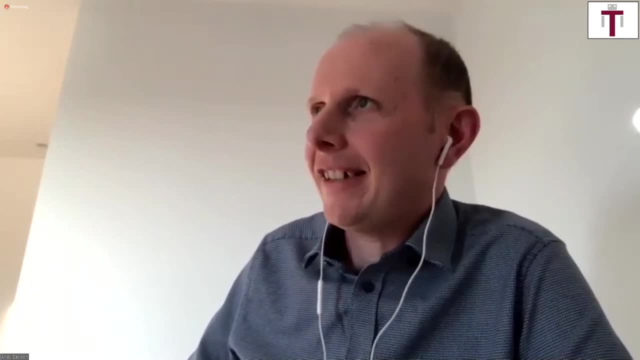 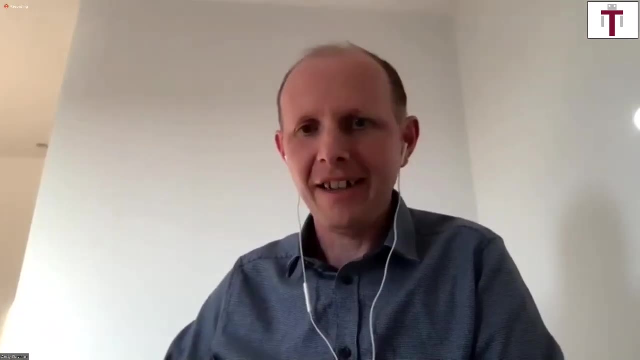 And of course, it's always an inspiration, And I think that I've realized more and more that I think I'd always thought the only thing I'm interested in is making systems that work, But I've realized more and more that I think I am also quite interested in understanding how some 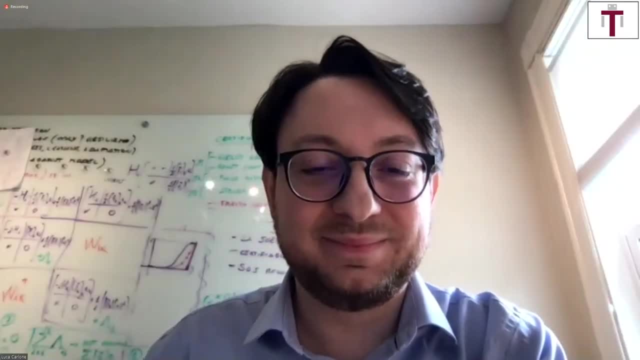 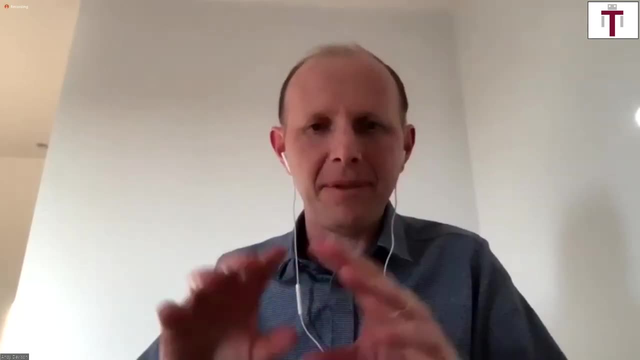 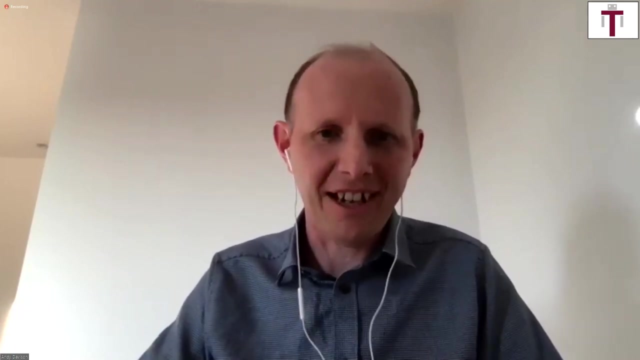 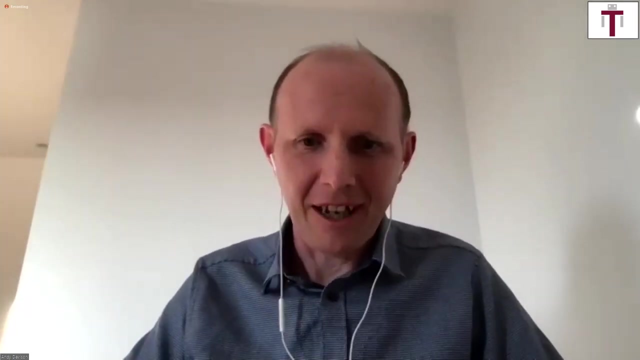 something about biological intelligence works, and I would never claim to have any expertise on that, but I just have a feeling that if we discover, you know, representations and computational patterns that enable really generally useful SLAM systems to work that are also efficient, I think we may also learn some useful things about other sorts of embodied. 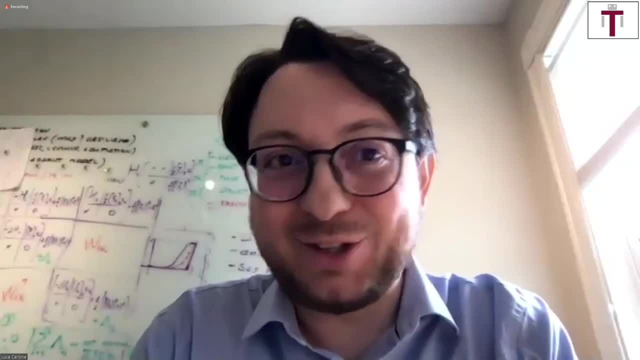 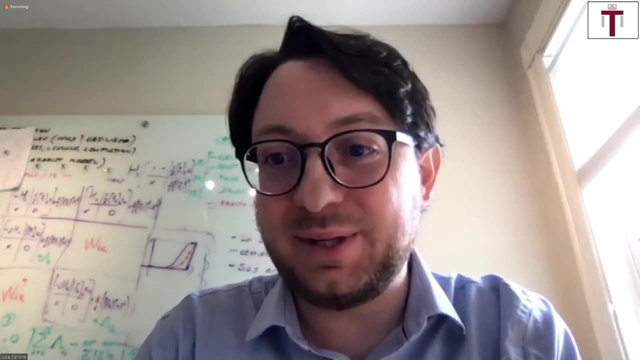 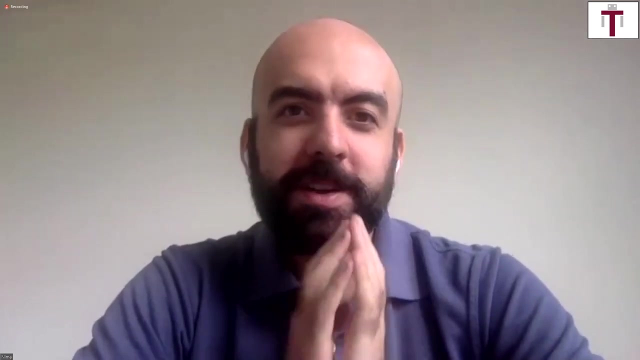 intelligence Very cool. So that is going to be like a much longer discussion, but since we have many questions from the audience, I will maybe call out on Nima to ask a question from the audience. Great thanks. So we had a question regarding memory. So, as you get these more interesting, 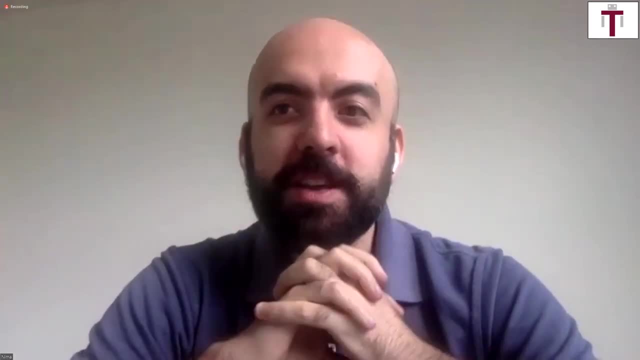 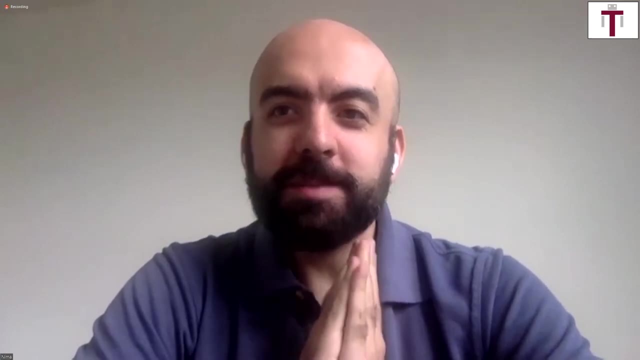 more high-dimensional maps or with the semantic information. if you're having an embodied AI, an agent that is supposed to move around and be untethered, how do you think that we can overcome the challenge of memory and capacity for maintaining these maps? 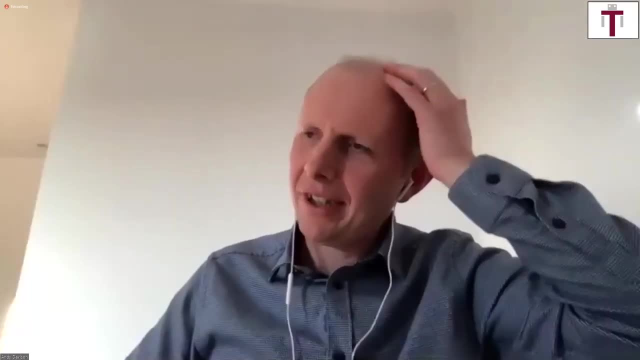 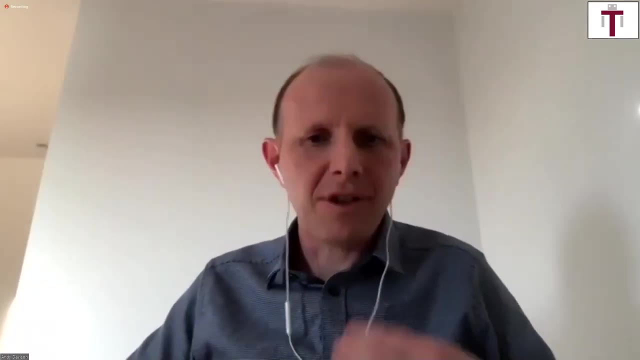 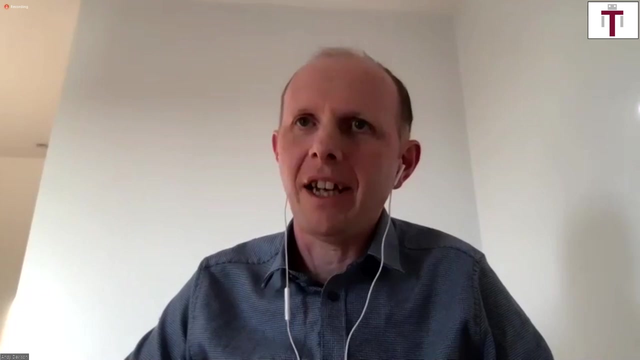 Yeah, great question and something we've thought a lot about. So I think the key is, you know, introspection and abstraction. So this is actually something we're concretely working on now, kind of in the graph processing work. So, you know, we've got this computational. 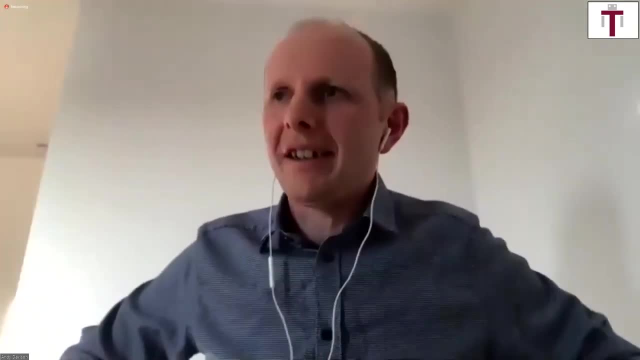 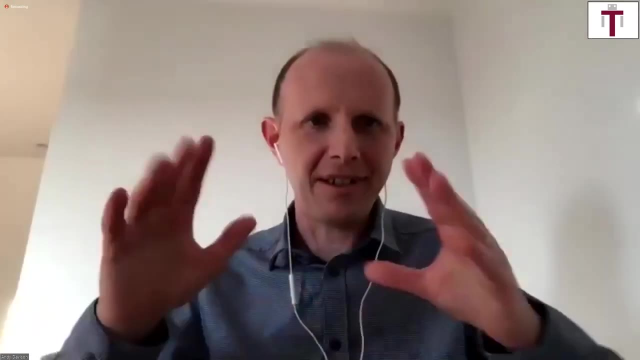 resource. you know, maybe it's an IPU chip that is able to basically process a certain size of graph and clearly, as if a camera keeps moving, mapping more points, the graph we're interested in is going to get bigger and bigger. but I think that what we can do to overcome that is always be looking for. 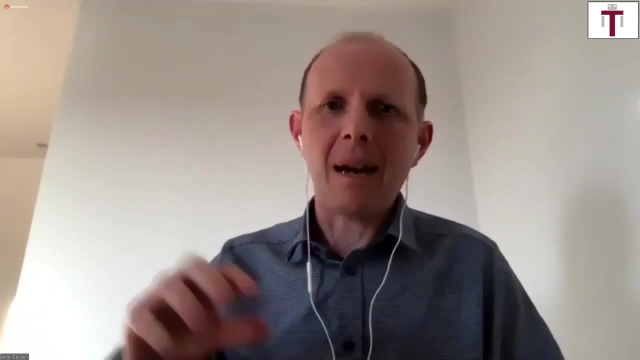 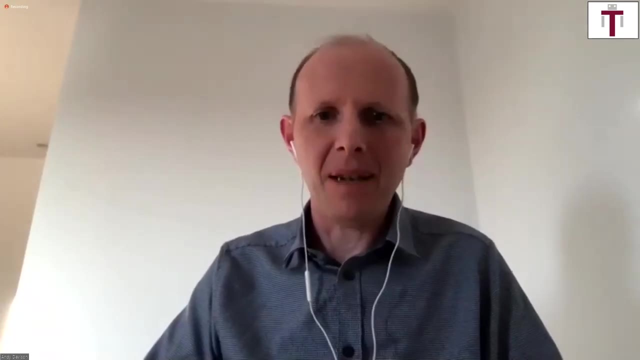 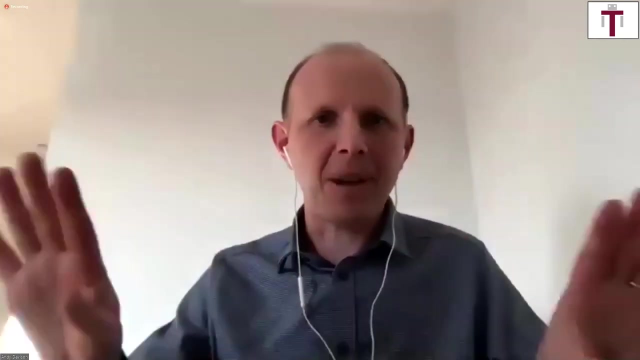 ways to simplify the graph. so, for instance, if we've mapped a hundred points and at some point we realize they lie on, all lie on the same wall, and maybe that information comes from, you know, a neural network that's telling us it's recognized a wall, or maybe it's just pure introspection that 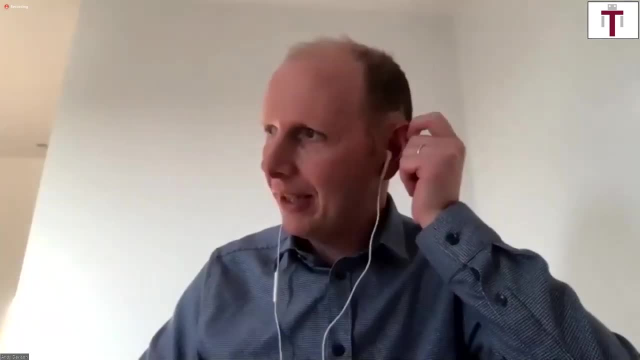 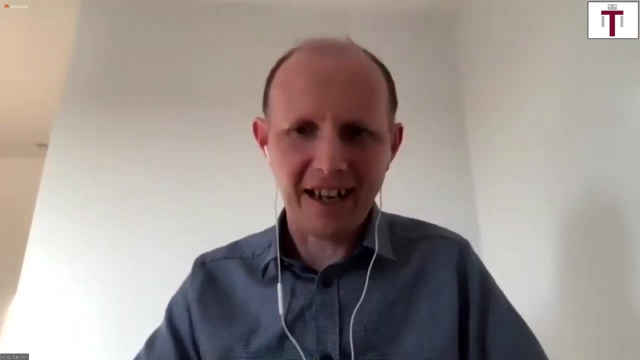 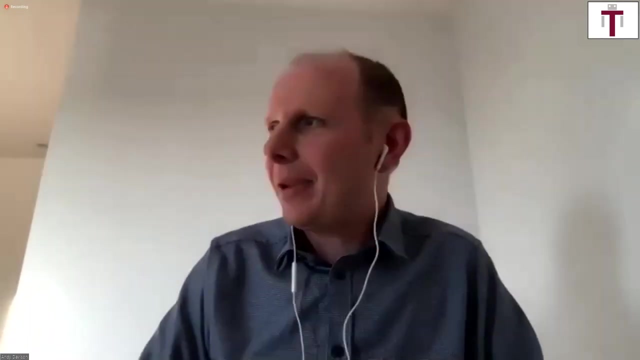 we check, we keep finding all those points are really planar. we could replace all of those nodes in the graph with a single, you know, plain node that abstracts and and captures all of the relevant information and then reconnect it to all the all the necessary places. so so I kind of think 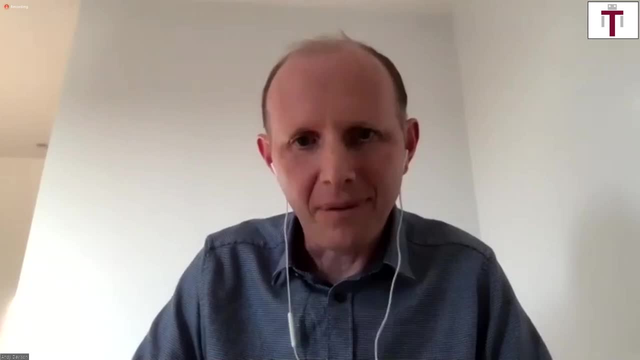 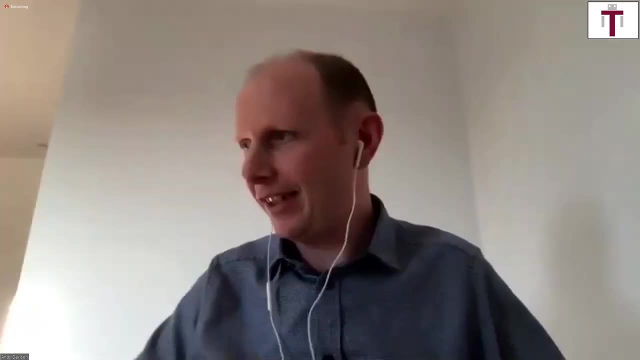 that's, that must be how you know scalable memory works. so you've got a lot of detail about the things you're looking at right now and then the things you've. you've, you know, maybe the things you're not looking at right right now they fade down to something more. 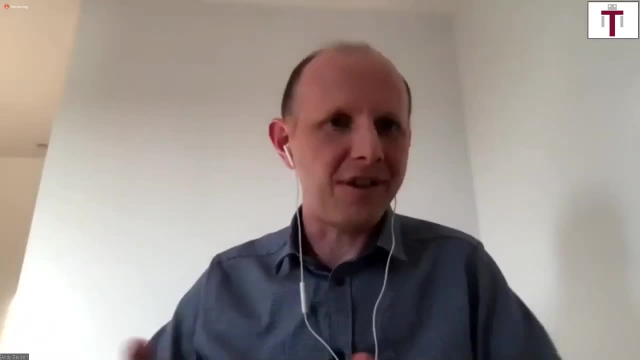 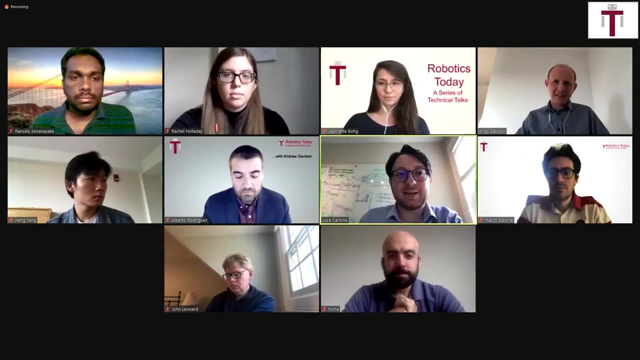 more abstract, which is, uh, still sufficient to to for them to be useful, but is much more efficient, and I guess the semantic understanding can also guide you, know what to compress and can inform how to compress uh things in the past. that's definitely absolutely yeah, yeah, so I think. 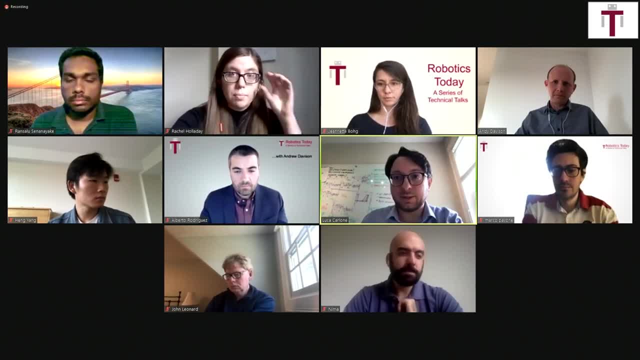 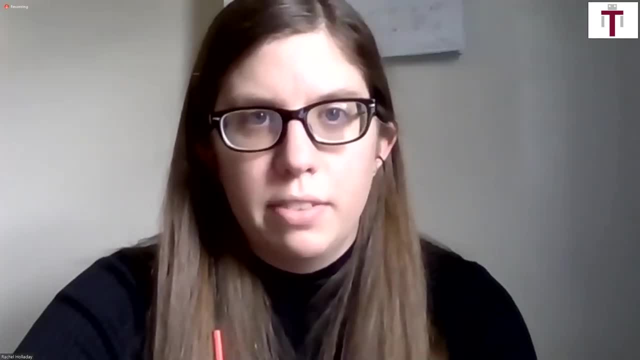 Rachel picked a very interesting question from the audience. uh, do you want to read it? so Lucas Manueli asked: how should the output of spatial AI systems be different, if at all, for different downstream applications like manipulation versus self-driving? and, I think, a related question from Emmanuel Franz. 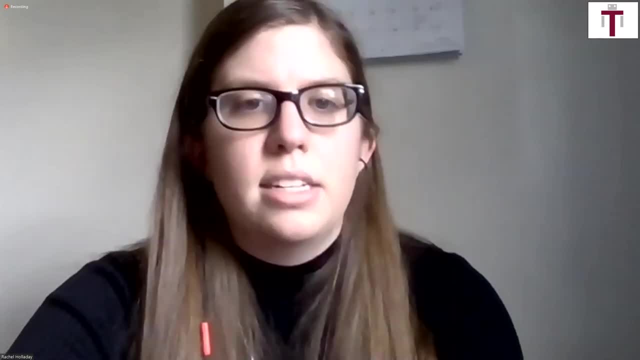 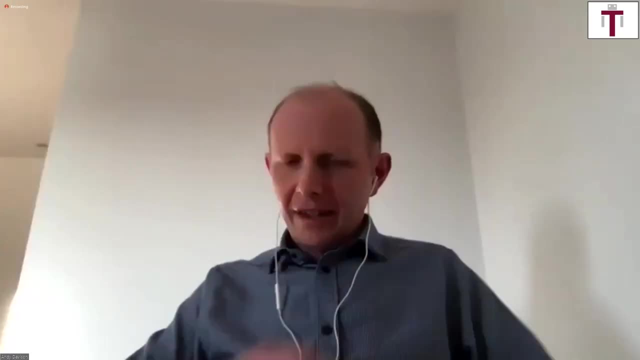 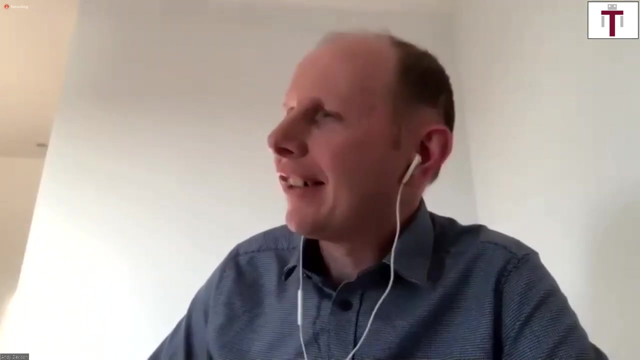 was about: how would you integrate, uh, semantic integration with NLP or human machine interaction in the context of these different applications? uh, okay, so let me take the first one. uh, so that this was about how much the how might the output be different for for different applications? um, 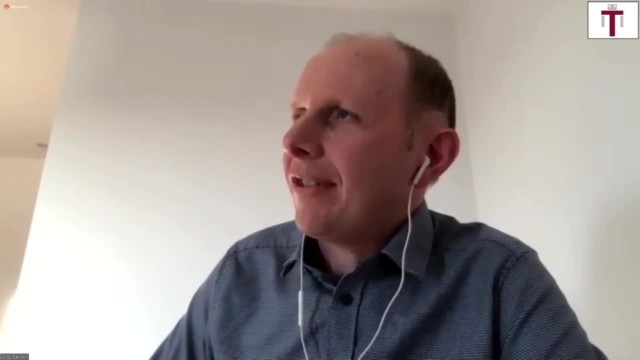 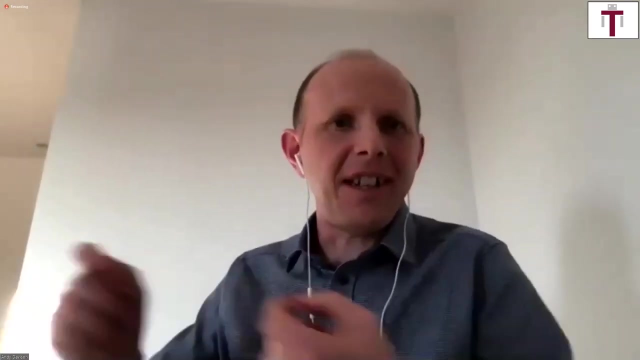 yeah, so it's, it's good question. so so clearly, different applications need need different capabilities. um, I think, you know, I think one of my hypotheses is they might not be completely different. um, so this may be more, more of a sort of continuum, so so I imagine there might be. 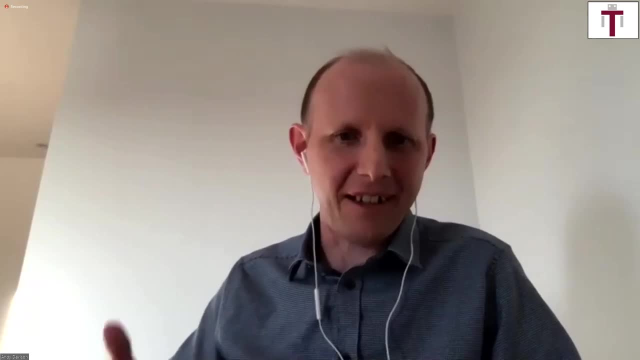 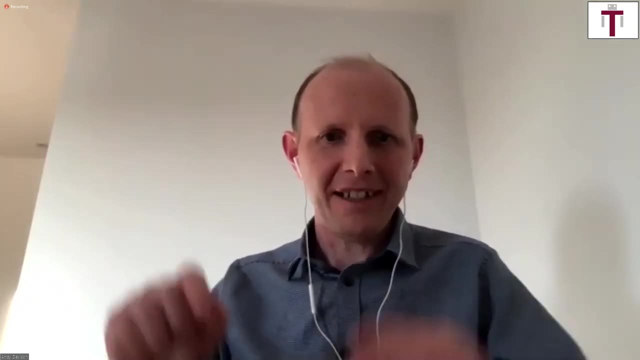 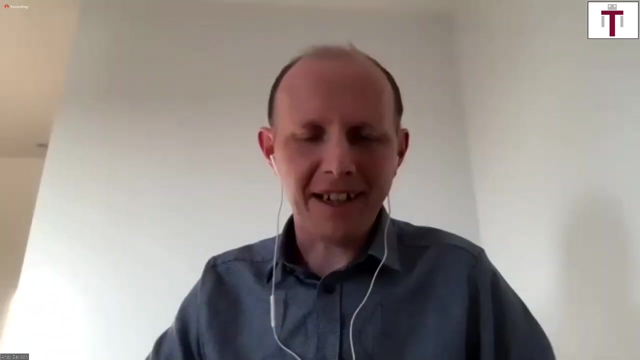 you know a relatively small number of performance parameters that are defining how well your system works. let's say, the accuracy that you can measure pose might be one. the density of, of of reconstruction. you know the, the, the level of fineness of your semantic labeling um the, the precision with 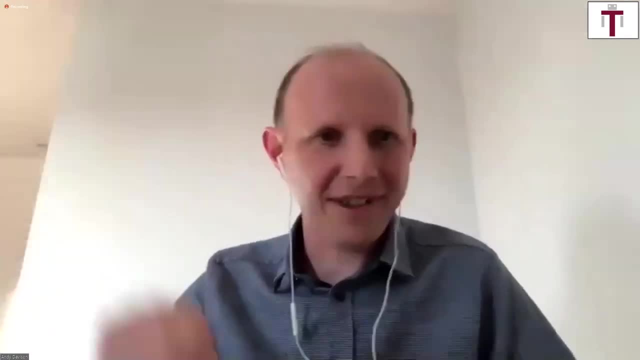 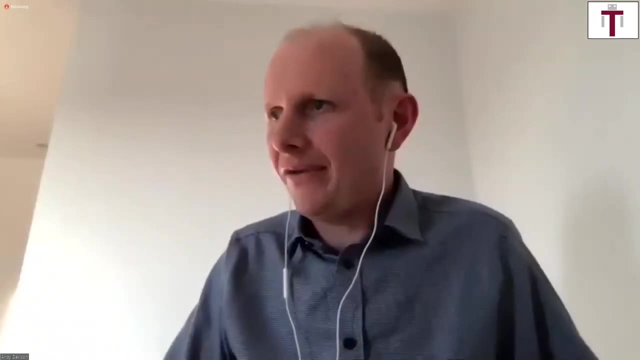 within which you can predict the time to contact of of that point that's directly in front of you, or or something like like that. maybe there are really relatively small set of of kind of system defining parameters like like that which each different application would would have to be. 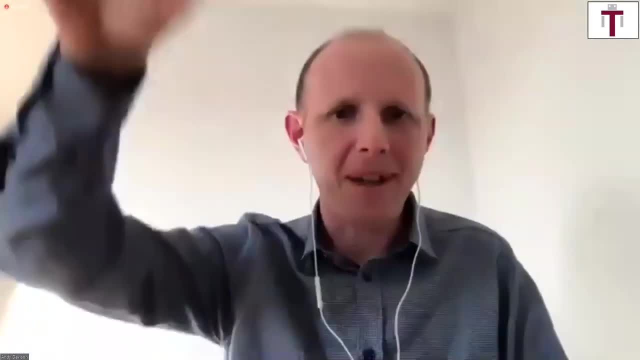 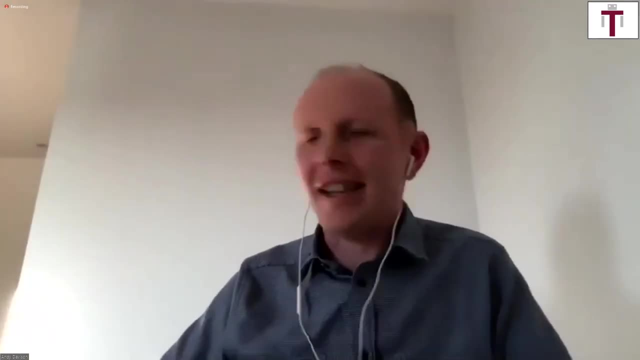 different positions on those sliders, you know. so a drone needs to be able to react to really quick changes, um, but you know, you know in other, in some other regard it might be. you know it doesn't have to deal very much with objects or or something like that, whereas a- you know, a home robot has. 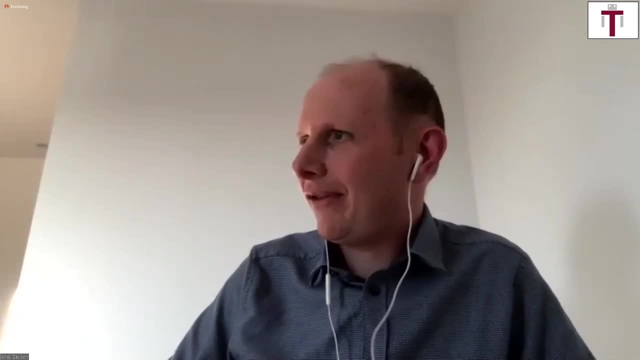 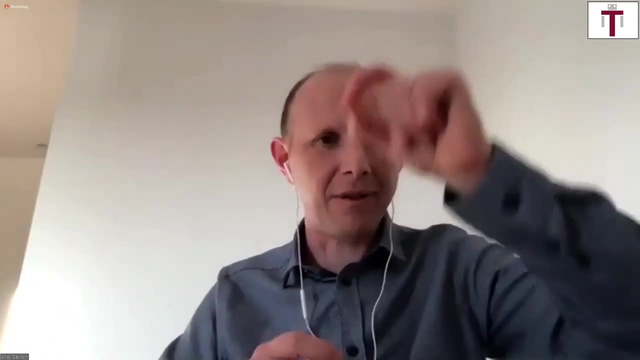 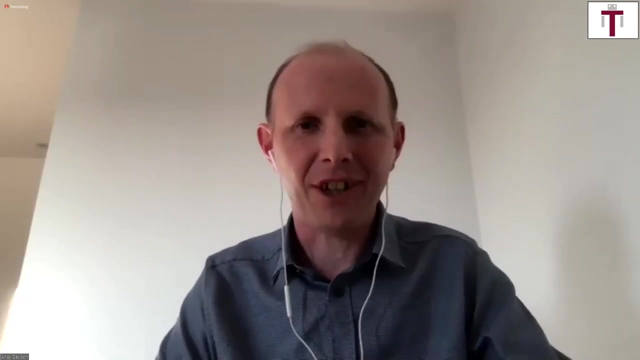 has different um so. so i i kind of hope that there'd be really relatively general sort of architecture for spatial ai which then you would specify a set of kind of performance requirements for a particular application and and the algorithm would hopefully can configure itself for kind of optimal performance with regard to those uh parameters. so could you remind me? 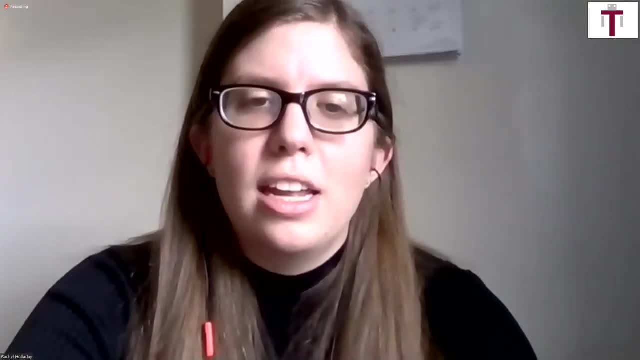 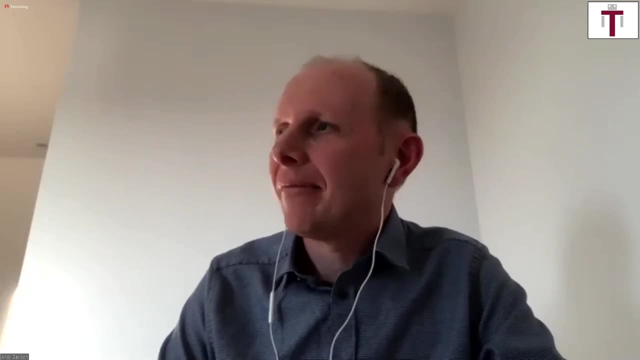 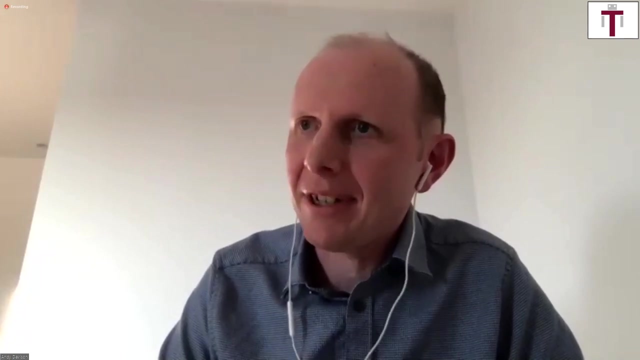 about the second question: yeah, the second one's about integrating in with things like nlp and human machine interaction. uh, yeah, um sure so. so another area that i really haven't uh done done any concrete, concrete work on, but is absolutely um important if robots are going to be, you know, working alongside uh people, so so the only kind, 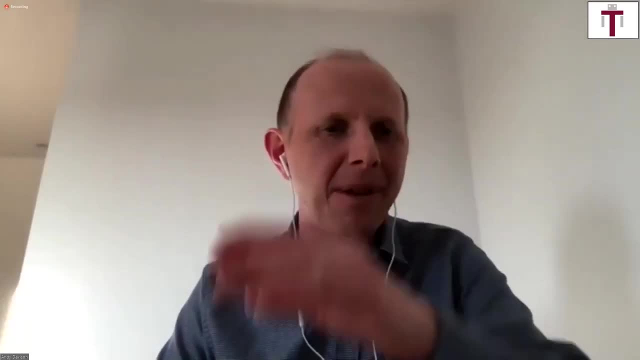 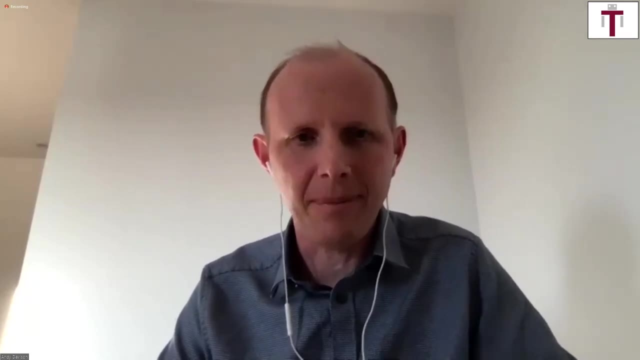 of concrete thing i can say is that i, as i think we step up in spatial ai towards these more semantic representations, we're going to have much more ability to be able to representations meaningfully done to a human. so you know, even when you, you know when you watch a. 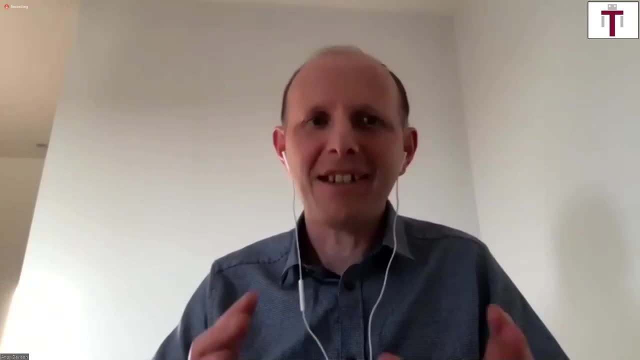 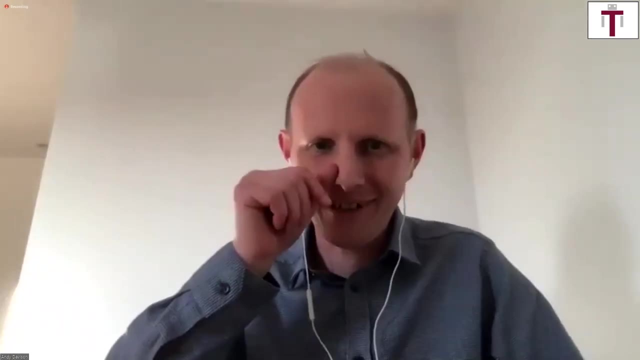 robot, vacuum cleaner, concrete work, but it's sometimes frustrating. i, i, i don't know, i don't. i must admit you, you want to do things like you know. go back to the kitchen. you know it's still dirty, or you know point over there, and so you know, go and spend a bit more time over there. so the 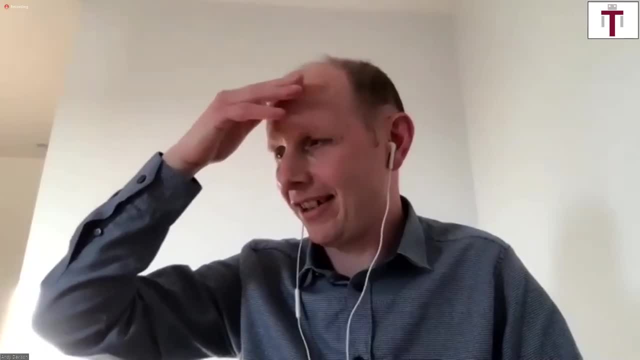 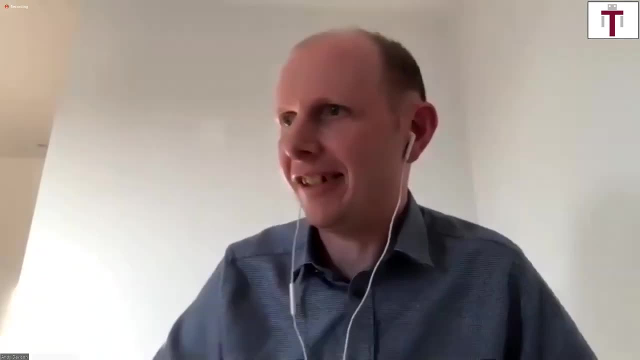 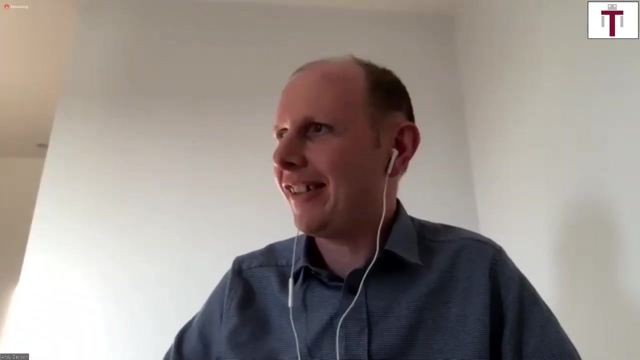 only thing would be fantastic if they can understand those things. so so, yes, i guess, if you imagine a set of queries like that of, of, of, of actions, like you know, go go back to the- you know the chair behind behind the sofa, and clean under there and think about, you know, are, are the, are the? 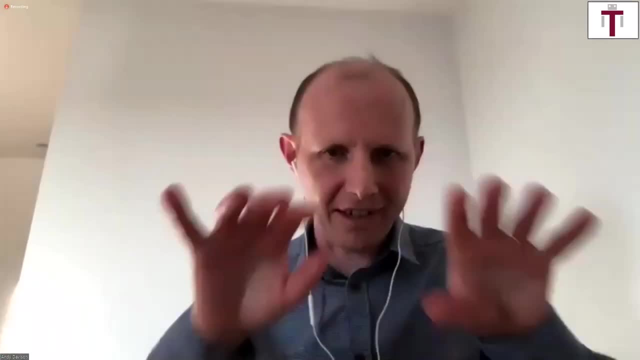 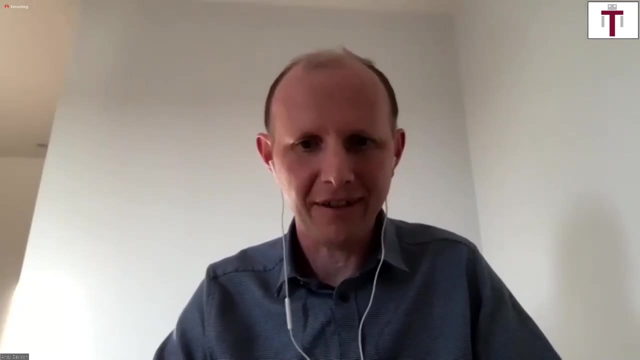 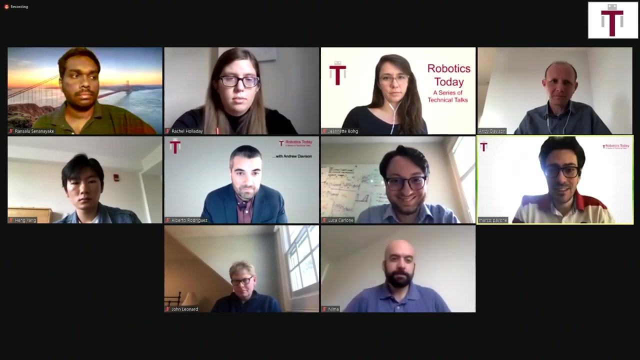 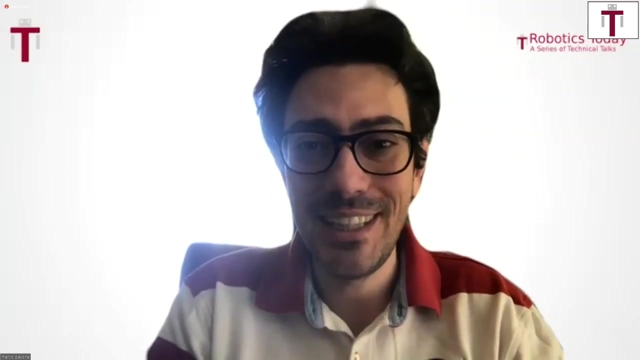 representations that we're building, which will hopefully be abstract and hierarchical. do do they to the scene graph like representations? do they enable those kind of actionable uh queries? thank you, andy. uh, fascinating uh discussion, fascinating talk. i really loved your historical perspective on this one problem. unfortunately, it's time to wrap this up, uh, on behalf of all. 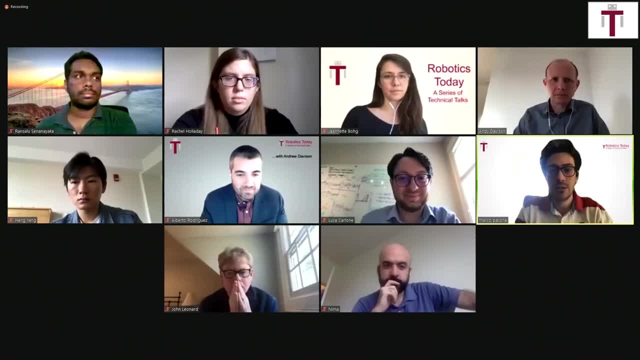 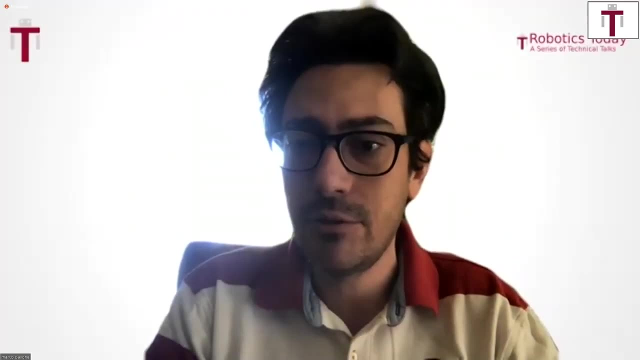 the co-organizers. alberto, i would like to thank uh everyone that has joined us today for the inaugural talk for the robotics uh today talk series. um. next week we're going to have another exciting talk from leslie cabling, from mit, on recent advances in decision making and reinforcement learning. 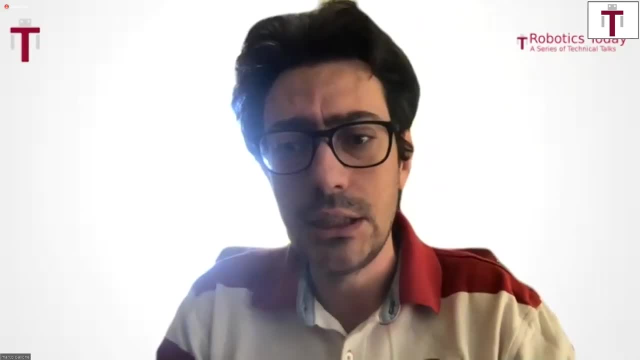 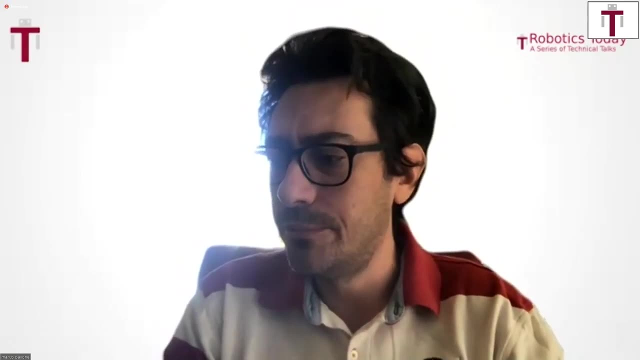 importantly- uh, this talk series is really an experiment on online robotics community building. i would like to thank everyone who has joined us today for the inaugural talk for the robotics, but our goal here is to view virtual talks not as an uh, as a backup option, but really as a new. 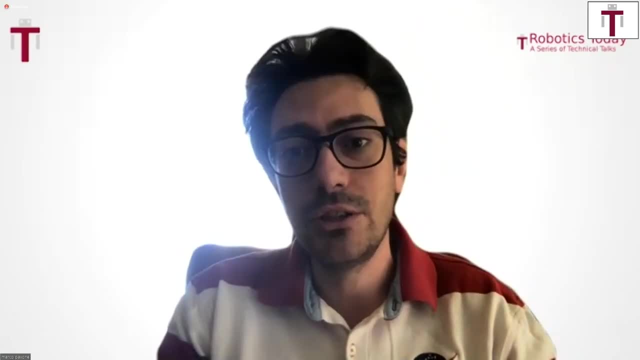 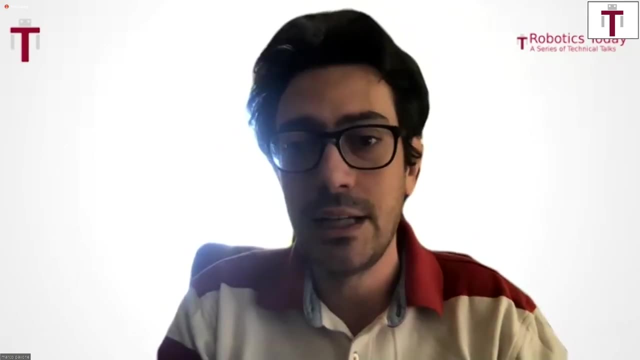 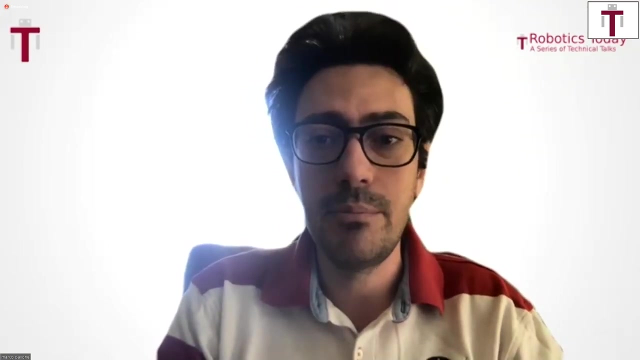 opportunity to achieve a broader reach for excellent talks such as the one that andy gave today. but we want to get it right, so it's very important to us to hear your feedback, so please go on the website, spend a couple of minutes and provide us with any comments you might have. 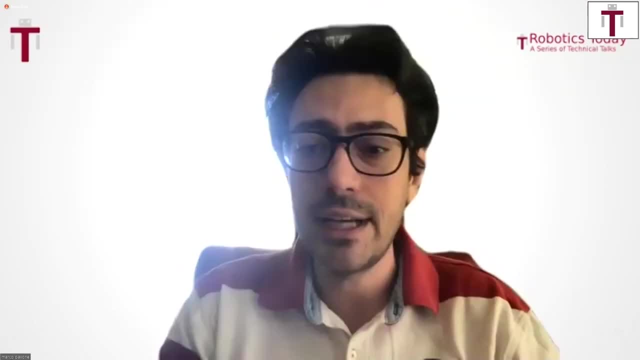 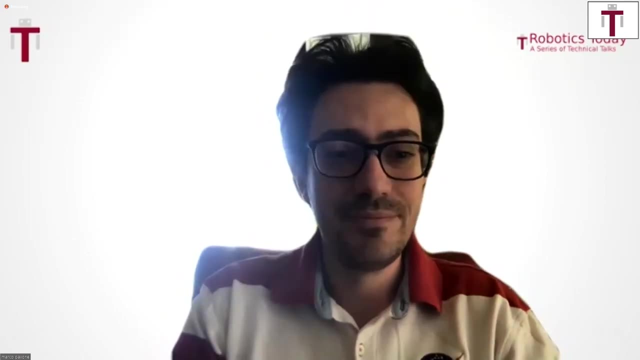 on how to make this seminar serious. uh, you know. at the same time, you know, because we are in a moment, more effective, more useful in general, great, thank you very much and I'll see you next week.